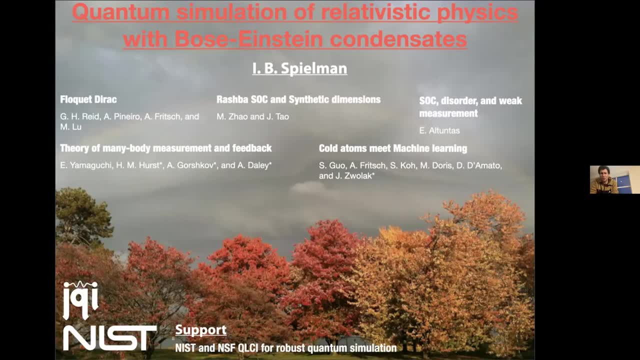 for Junior Experimentalists, which maybe doesn't say so much to you, but it's the APS most important award for junior experimentalists. In addition, he received an honorary doctorate from the University of Vilnius, which he is also proud of. 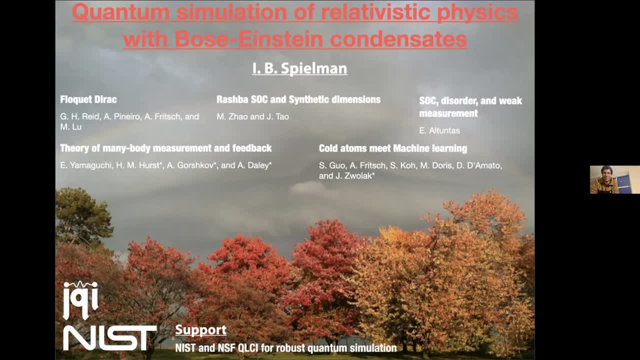 So with that, let's let me turn it over to Ian and his talk on relativistic physics. Is that right? I think the slide is a little cut off on my screen. Yeah, that's, I mean. it seems to be okay. I have a monitor screen next. Yeah, 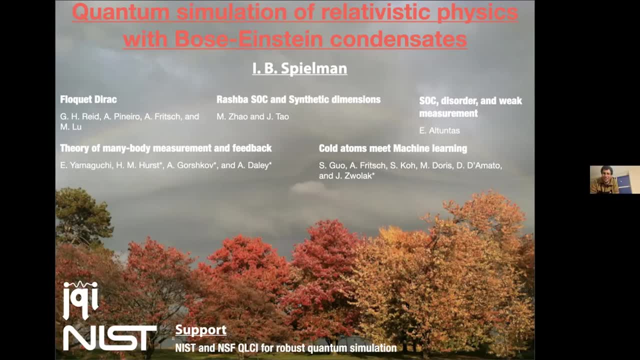 this relativistic physics with both Einstein condensates. So, Ian, to you, thank you for giving this talk and everybody enjoy. Thanks very much, Gil, for the kind introduction, And thank you for the, for Patty for setting this up and all of you for spending part of your. 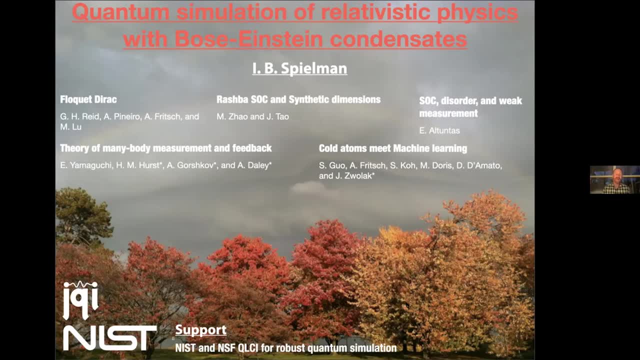 evening with me On the tour. we're going to have through some early predictions to quantum mechanics that were only now, by quantum simulation, ever realized. So, as Gil said, the talk's title is going to be quantum simulation of relativistic physics with both Einstein condensates. 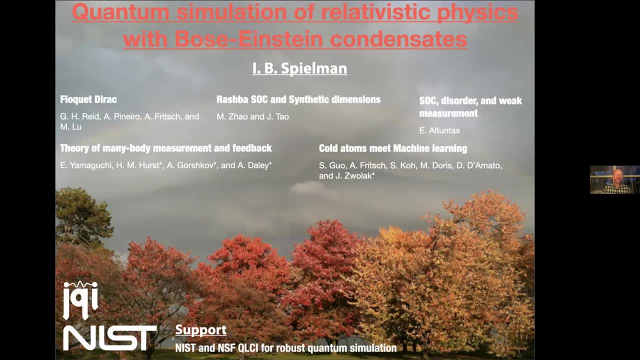 and for those of you who are not specialists in any of this, which I assume are most of you, I'm going to go through all of these sort of fancy sounding words and break them down so we can have a good understanding what's going on. And the names underneath my names are sort of 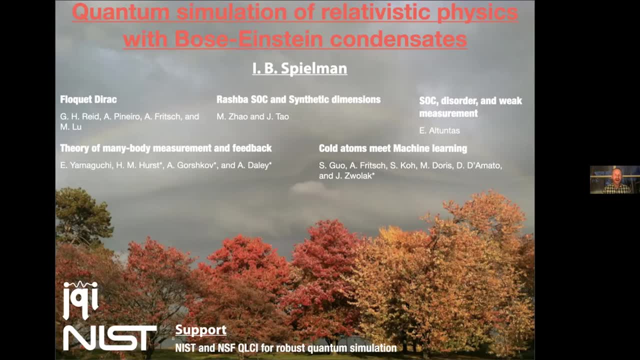 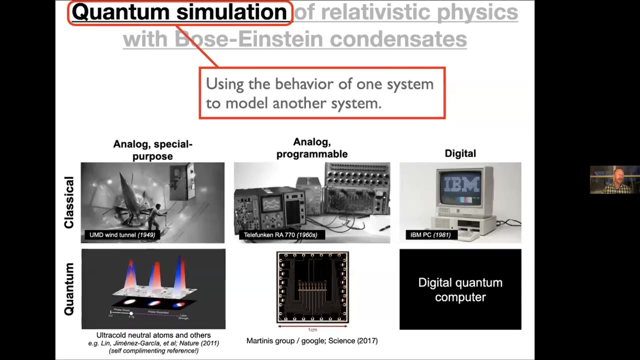 a list of current projects going on in my group. The only one person actually on this list whose work will be reflected today is Alina Pineros, who has done one of the two relativistic projects I'll be describing to you. All right, so let's start out with the first word of my title. 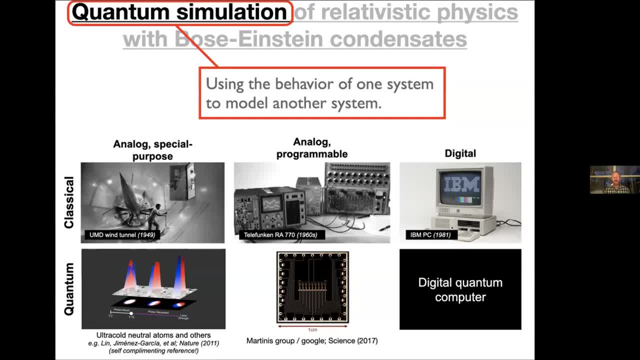 quantum simulation. So what we're trying to do is use the behavior of one system that we can control really well to model some other system that we either can't access or have limited control over, And I'd like to sort of place this idea of quantum simulation in the broader context. 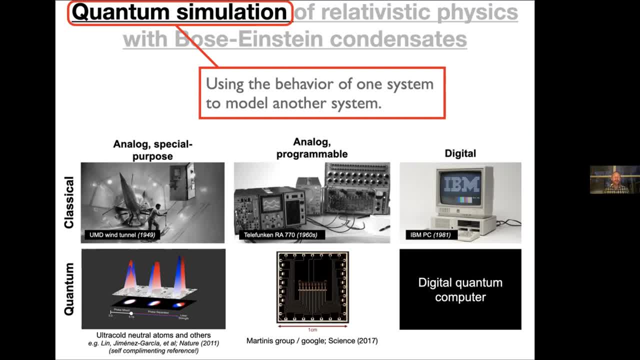 of computation in general. So if you look on the grid in the bottom, the first element down here is classical analog simulation, And what I mean by that are things like wind tunnels, where one builds an analogous system, a physical system whereby, scaling the appropriate equations, one will see the same physics that this sort of 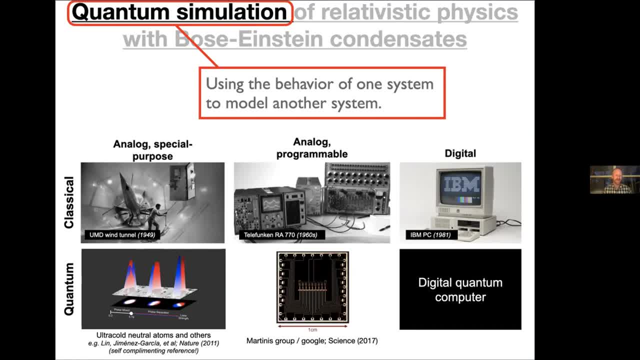 hypersonic device might see were constructed to full size. So this is a special purpose device custom built to test aeronautical applications. In the 1960s and 70s, devices called analog programmable computers existed. This one, for example, was to predict the weather. 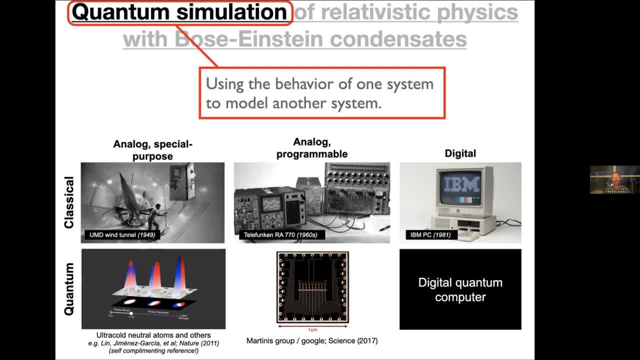 And it was consisted of nonlinear elements like transistors and diodes, along with linear elements like inductors, capacitors and resistors, And what it did essentially is solve a wide range of nonlinear differential equations And, until the advent of rapid and accessible digital computers, 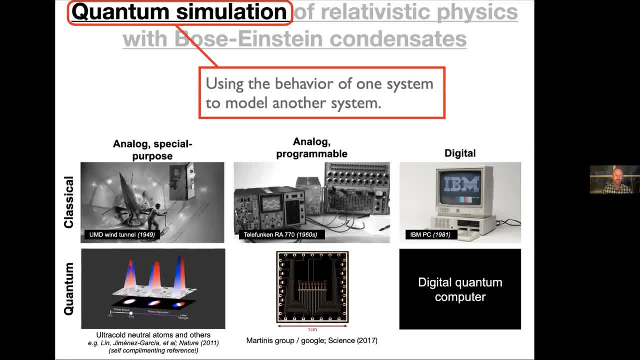 such analog devices in fact were the most powerful computational tools we had for these kinds of nonlinear problems, And digital computers- the workhorses of this type of computation today- really got their claim to frame because of easy programming and highly robust computation. So this is sort of the classical computational paradigm, And if you look, 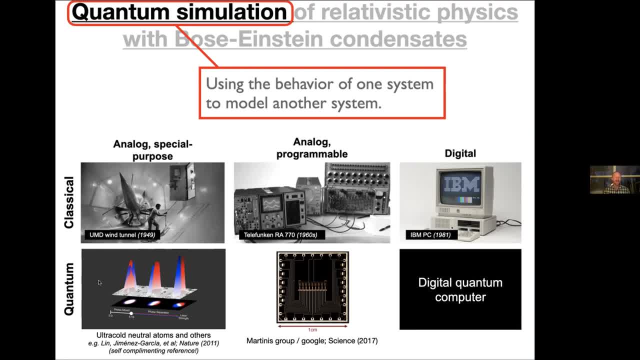 at the bottom row we'll see the sort of analogous steps that are being currently undertaken in quantum systems. So the first category is again a special purpose, And one example I'll give, which is sort of self-aggrandizing, is creating special Hamiltonians or understanding. 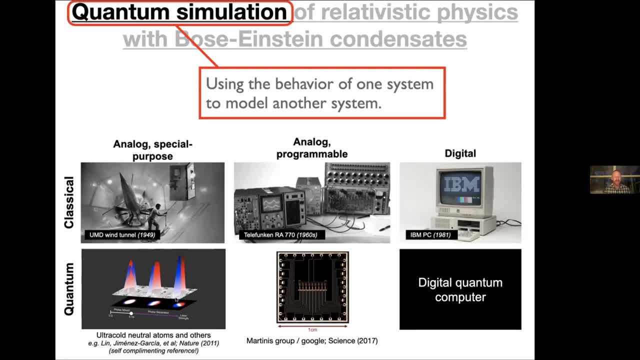 certain quantum systems by building analog systems, in this case out of a cold atomic gas. Similarly, great progress is being made using having programmable but analog quantum devices. In this case, I have an early picture of a Google-based, a Google-designed quantum circuit, And although they're pitched as 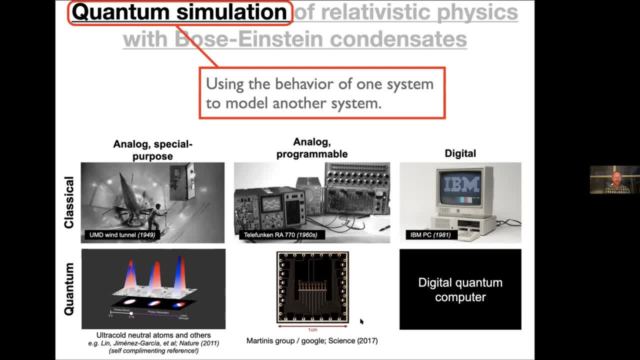 quantum computation devices because of the lack of error correction. they're really analog programmable devices very similar to this kind of programmable differential equation, solver above. And of course, currently the last element of this grid does not exist, which is a fully complete digital quantum computer that can in fact execute arbitrary algorithms. 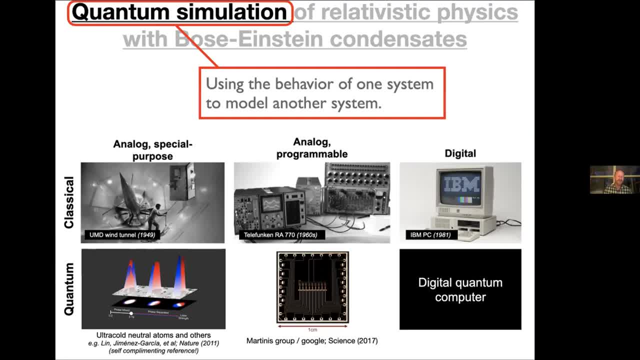 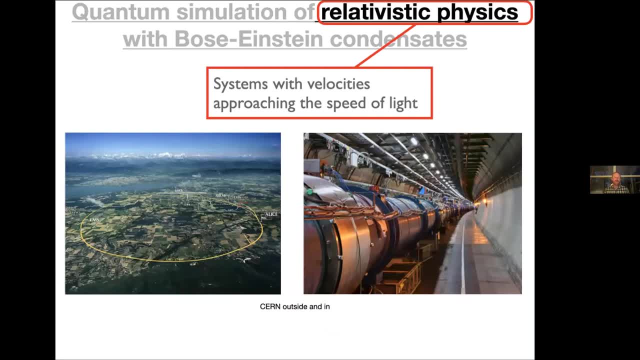 So certainly this would be wonderful to have, But right now we're in these bottom two categories for quantum simulation. So the next thing I'd like to sort of think about is relativistic physics. I'd like to tell you what I think of and, for the purpose of this talk, what relativistic physics is. 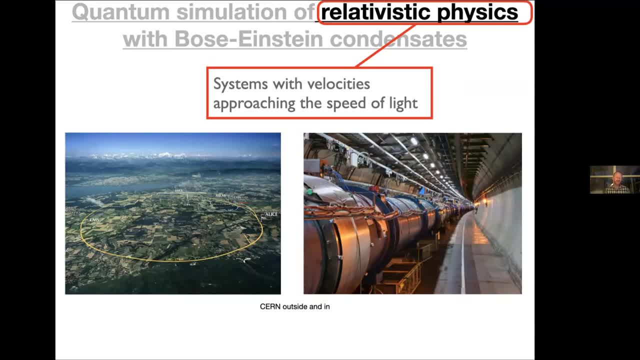 So really it's any system where the speed of light becomes important, where the particles are moving fast enough that their velocity is close to the speed of light. We're going to call that relativistic. Ordinarily relativistic physics in experimental laboratories might be. 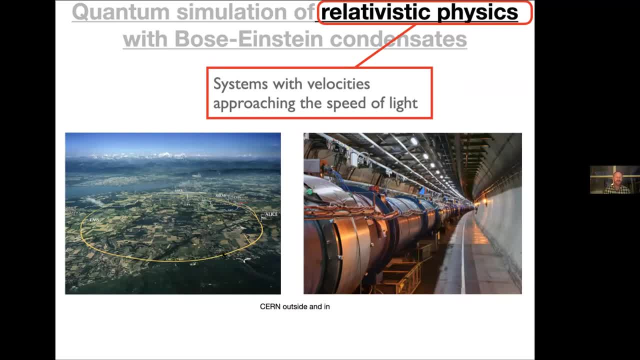 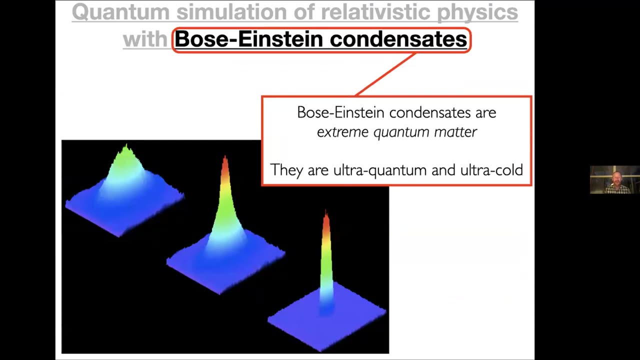 confined to things like these: two pictures of sort of the large storage ring, And here is a photograph showing the very gentle curvature down this collider system. And the last ingredient on this are bosons and condensates. And bosons and condensates are extreme quantum matter. They're both ultra-cold and ultra-quantum. 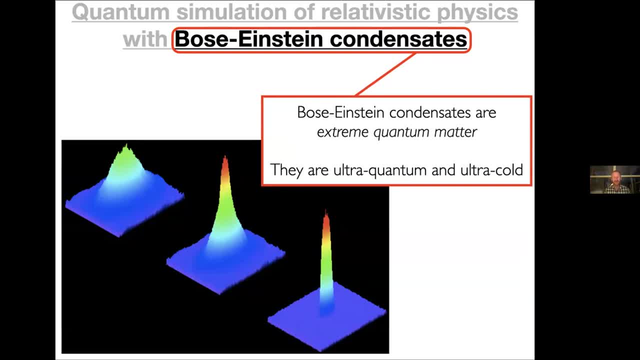 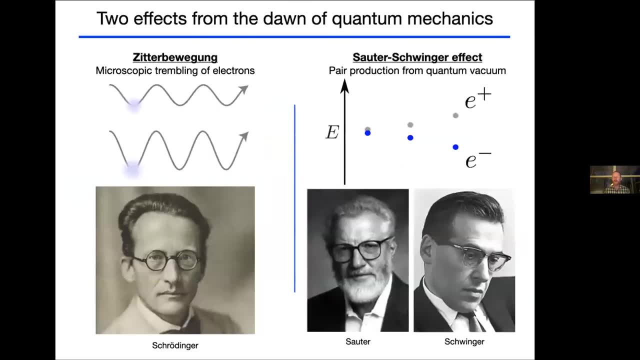 And I'll be shortly describing what I mean by both ultra-cold and ultra-quantum. So in this talk I'll be describing two effects from the dawn of quantum mechanics as we take our tour through quantum simulated relativistic physics. The first of these is Zitterbewegung. 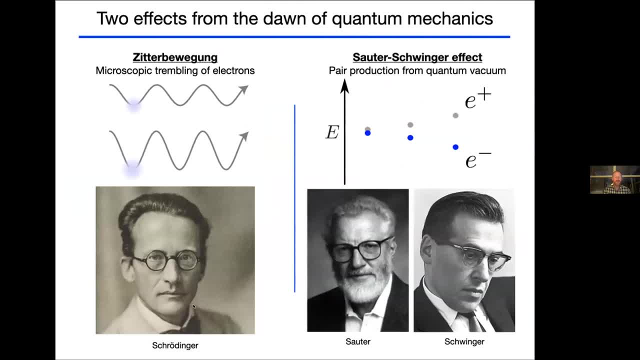 which is a prediction from Ernst Rodinger very early in quantum mechanics in the 1930s, that if one looked carefully enough at a fundamental particle, an electron, you would notice it would undergo microscopic trembling motion, both very fast and very small. 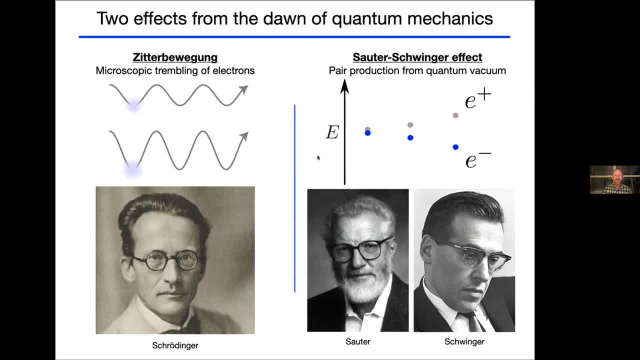 And I'll again give you scales shortly. And the second effect I'll be talking about is the Sauter-Schwinger effect, And this is pair production from the quantum vacuum. The idea is, if you apply a sufficiently large electric field and you visualize semi-accurately, 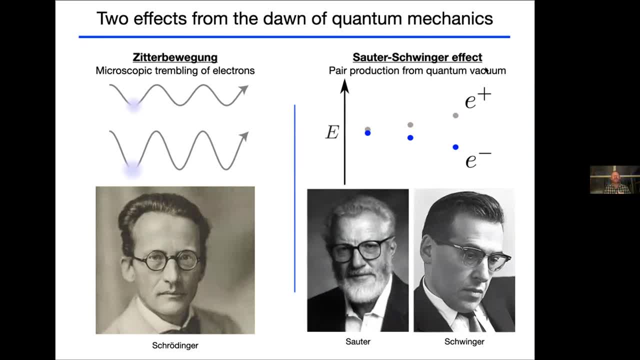 the vacuum of the quantum system, as sort of having fluctuations that occasionally produce electron-positron pairs out of nothing. a larger electric field can accelerate these particles away from one another, giving real life to these otherwise virtual particles, And we will also see in the end of the talk. we'll be talking about the Zitterbewegung, which is a prediction of 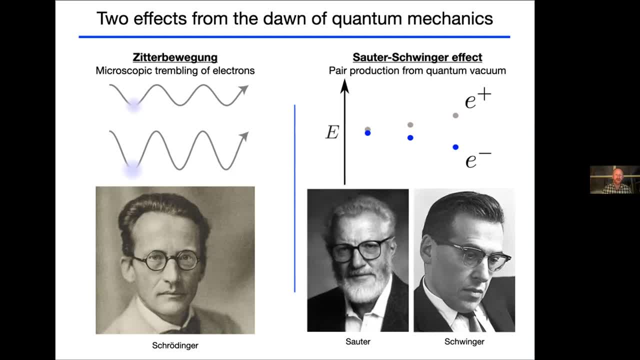 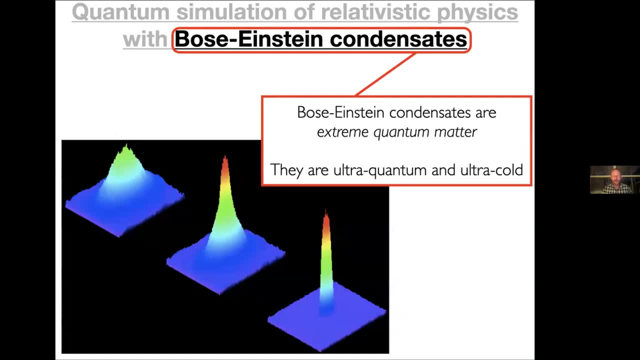 an analog to this in our cold quantum system. All right, So with that I want to turn back to Bose-Einstein condensates. What do I mean by ultra-cold and ultra-quantum? Well, I want to start out with everyday quantum mechanics, the quantum mechanics that, at least myself, has gotten very 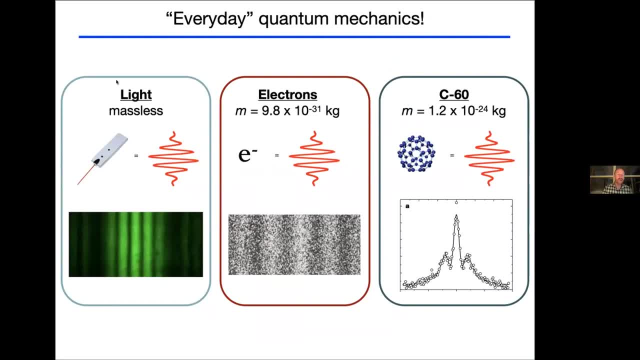 used to. So I think everyone here is familiar with the idea that light is composed of massless particles, that we would call photons, And these photons can interfere with one another, for example giving this double-slit interference. So if you have a double-slit interference, 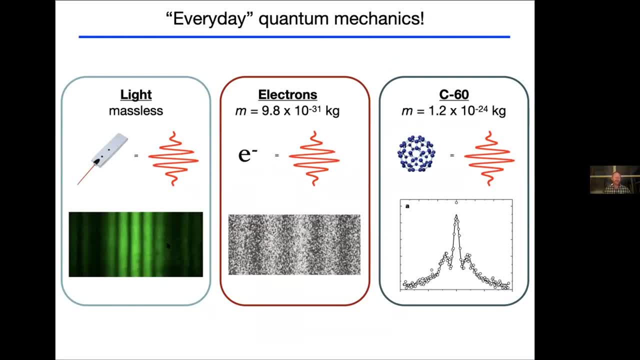 you have a double-slit interference pattern here, And this really has been surprising to no one for a very long time, not since a modern electrodynamics was developed 150 years ago. So that also predicted that light is a wave. However, much more surprising was the quantum effect that electrons. 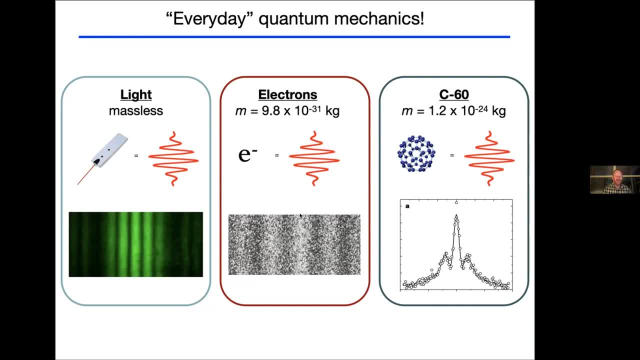 can behave as waves as well, giving double-slit patterns as I'm picturing down here. And really this fact that particles can act like waves extends to every scale if you work hard enough to find it. And here's an example, perhaps 15 years old, of an interference pattern of a molecule. 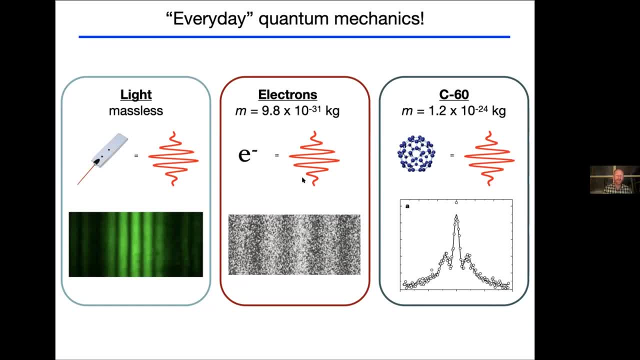 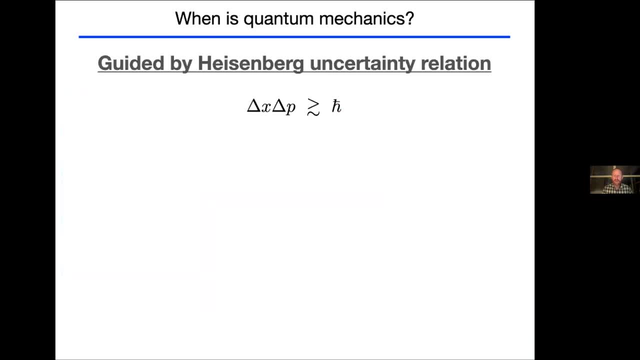 of carbon-60, also showing the same kind of double-slit pattern that both light and electrons can display. So this is some great wave quantum mechanics, And a question you might want to wonder is: well, when are you going to see quantum effects roughly? And we can be guided by the 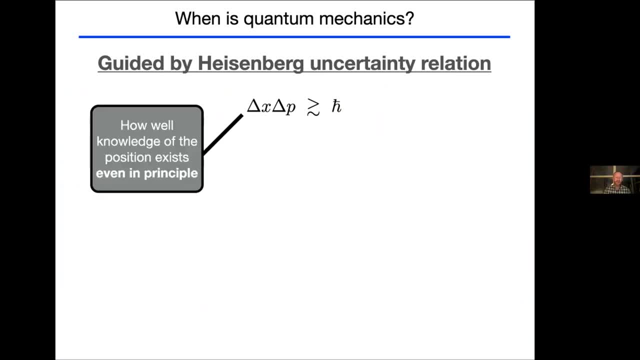 Heisenberg uncertainty relation to ask this And we can ask: well, how well, even in principle, can we know the position of a particle? That's what I'm going to call delta x. It's not how well you bother to know, it's really how well, in principle, you could have known. 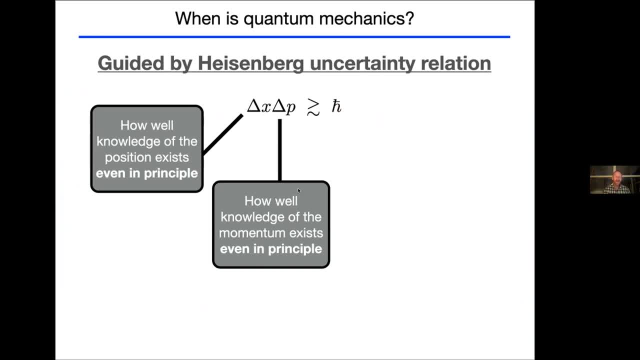 We can next look to delta p. P is the momentum And it's how well, even in principle, knowledge of the momentum exists. And the Heisenberg uncertainty principle tells you that the product of these two, the uncertainty in principle of position and in principle of momentum, 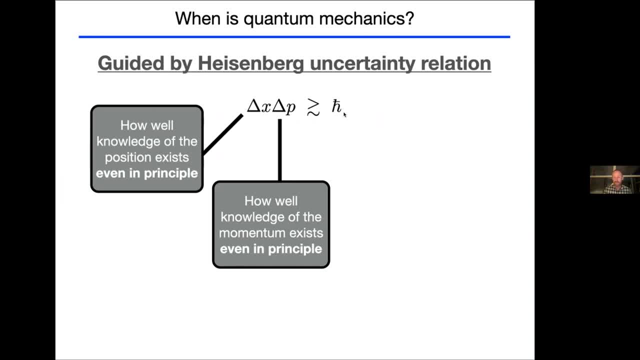 is going to be greater than or comparable to Planck's constant. Now, Planck's constant is a really, really tiny number, so 10 to the minus 34 joules per second. It's really hard to comprehend 10 to the minus 34, but that's a billionth of a, billionth of a. 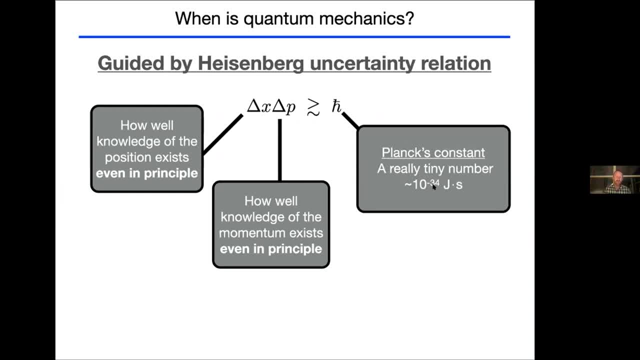 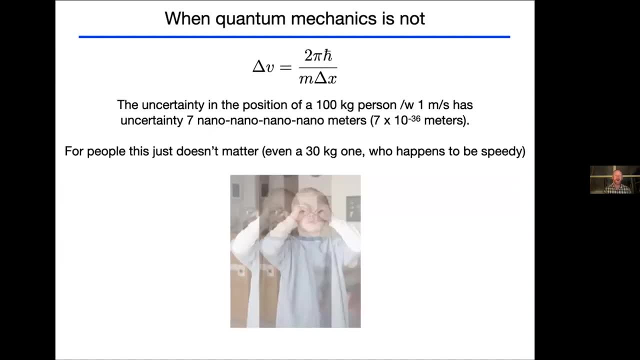 billionth of a billionth, that kind of small. So it's a really really tiny number compared to terrestrial scales And for that reason one really almost never sees quantum effects in real life. So, for example, if I was to wonder about the fundamental uncertainty in the position of 100. 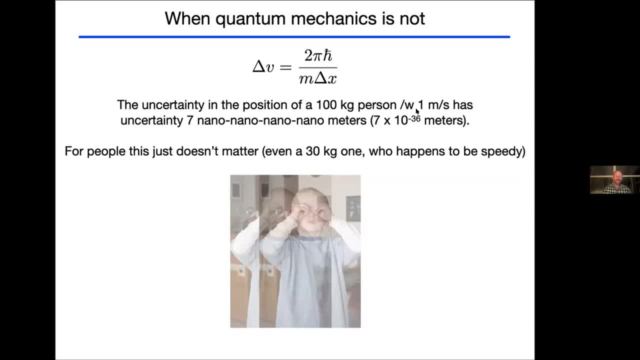 gram person, whose velocity uncertainty is about a meter per second. well, the positional uncertainty is seven nano, nano, nano nanometers. So that's seven times 10 to the minus 36 meters, which, of course, is an incredibly tiny number considering that the size of, for example, 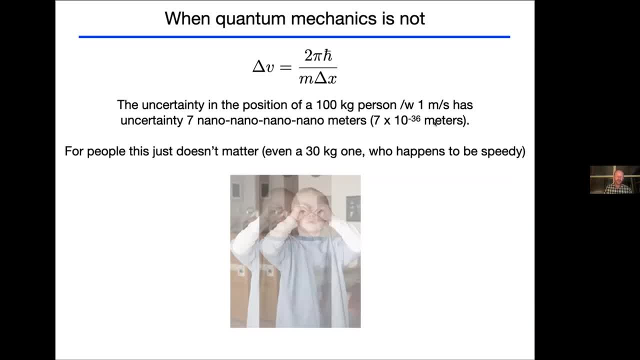 of a hydrogen atom is only a fraction of a nanometer, so a billionth of a meter. So this is much, much smaller than any scale you'd ever see. So for that reason, even for comparatively light people, for example, this one who is relatively speedy- you don't see any kind of 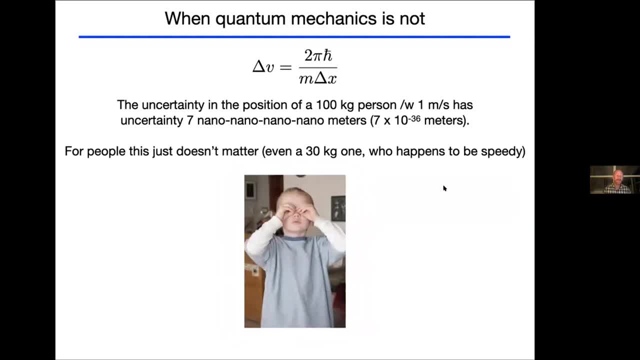 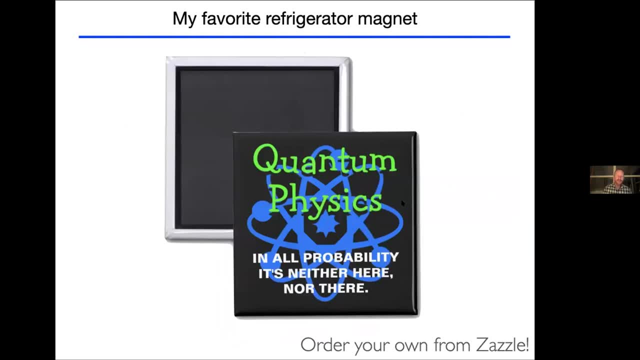 quantum effects at all. So quantum effects appear in your everyday life, And this brings me to my very favorite refrigerator magnet. So quantum physics: in all probability, it's neither here nor there. Of course, in real life it's here and not there. Okay, so that's, when do we see? 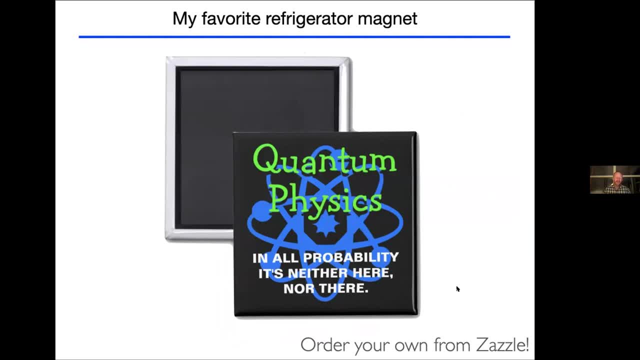 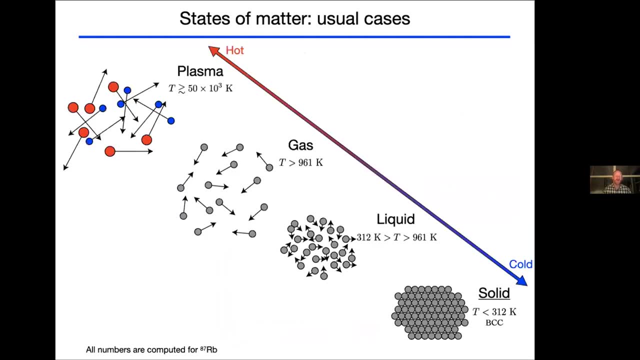 quantum mechanics for systems that have the product of the position and momentum are very, very small. So when can we see that? How can we approach quantum physics in the laboratory? Well, one way to do it is to make things very cold. This phase diagram, or the 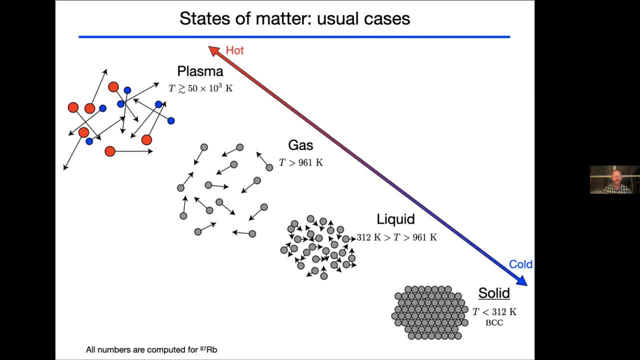 sketch of the typical phases of matter. I'm plotting here really don't have anything particularly quantum about it. At very, very high temperatures, a typical gas with enteroplasmic phase, that's when there's a significant fraction of electrons that have been stripped off, the atoms moving. 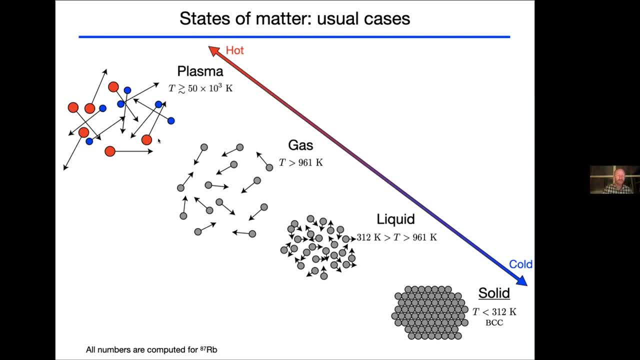 around in tandem now with the charged ions, that were the atoms. At lower temperatures, the electrons bind strongly to the atoms producing conventional gas, such as in the room around us And even lower. this gas condenses into a liquid and, of course, 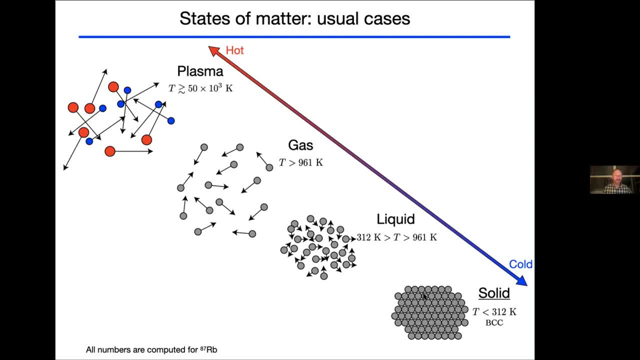 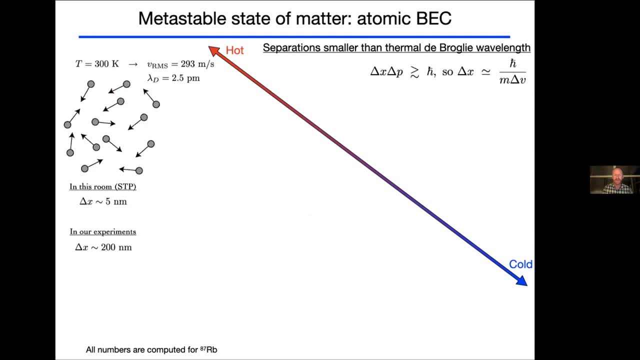 at lower temperatures it freezes. So, on this list, where is the Bose-Einstein condensate? How have we managed to miss this really important phase of matter, this quantum phase of matter? Well, in reality, a Bose-Einstein condensate is a metastable phase of matter. 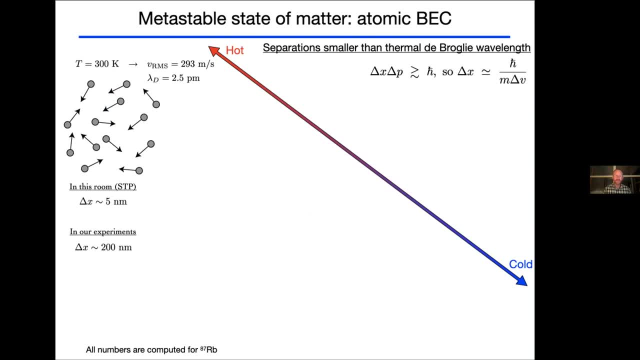 If we did make a Bose-Einstein condensate in the laboratory, if we were to wait long enough, we would find that ultimately it would find a way to disappear and turn into a flake of cold rubidium or whatever atom you're using- on the bottom of your vacuum. 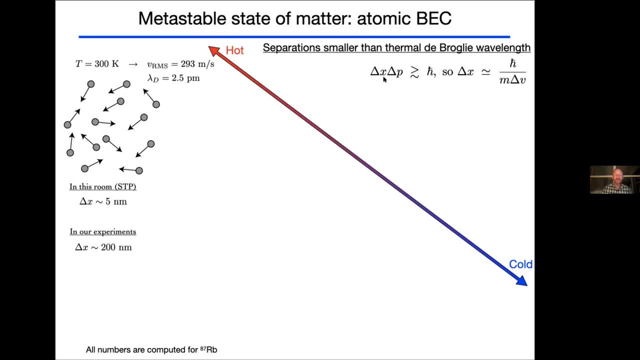 system. So again, guided by the Heisenberg uncertainty principle, let's see how this works. So again, we're going to consider the product of the uncertainty in position times, the uncertainty in momentum, And we're going to try to see when this uncertainty in 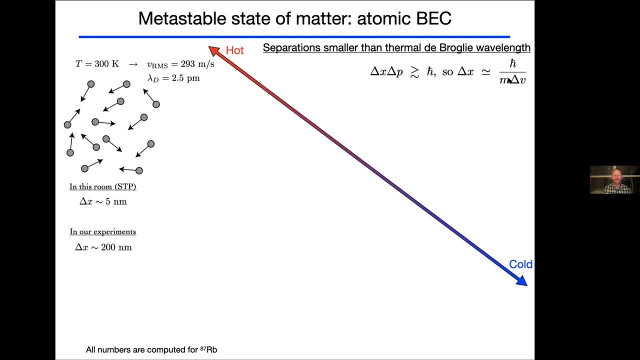 position becomes comparable or is fundamentally given by this uncertainty, Which is simply from the uncertainty relation. So, starting at room temperature, the typical uncertainty of the velocity of a particle, this is the thermal uncertainty. it would be about 300 meters per second at room temperature And finding this uncertainty in 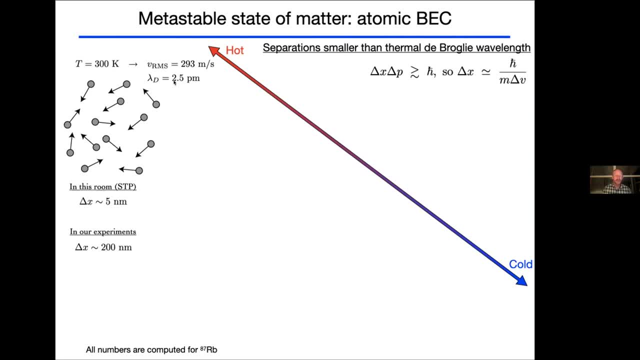 position associated with that size. by the Heisenberg limit you find a scale of 2.5 picometers, So that's 2.5 times 10 to the minus 12 meters. It's a really small number, smaller even than the atoms themselves, But a really important thing I haven't mentioned. 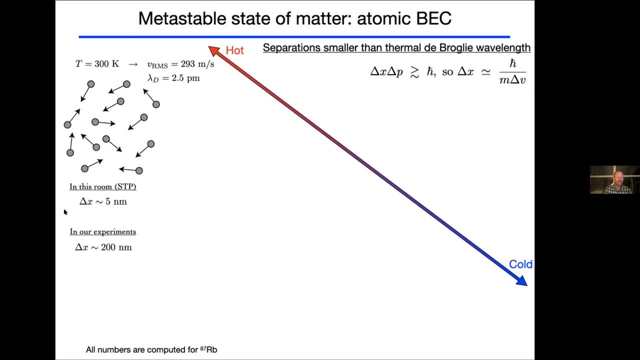 too, is a different property, which is a separation between particles. So, for example, in this room right now, gas atoms might be five nanometers apart, And in our experiments they're perhaps 200 nanometers apart. So what we're going to really 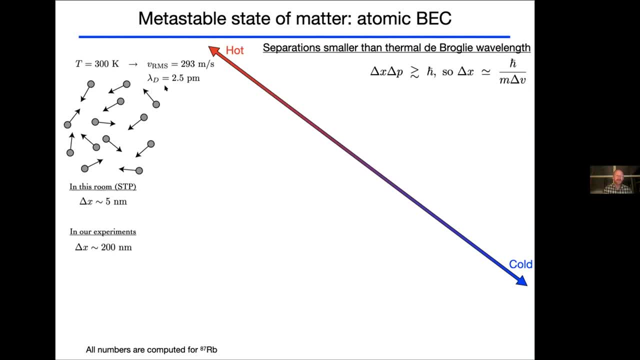 do is compare the separation between particles to the fundamental uncertainty about how well we can know where they are. So as we cool this gas down from a balmy, 300 Kelvin- that's about room temperature- to one Kelvin, that's just one degree above absolute zero- the velocity. 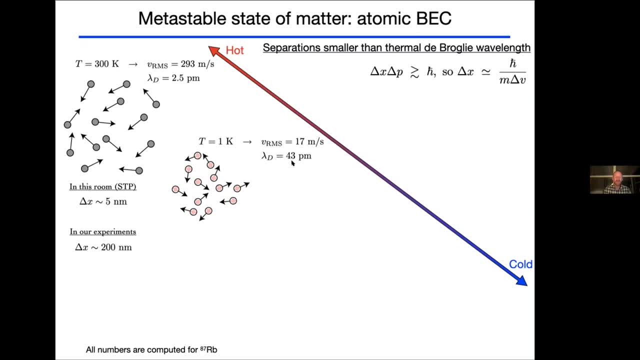 might slow to 17 meters per second And the uncertainty in position would increase somewhat to 43 picometers, which is still really tiny, still smaller than even a hydrogen atom. So in this case you still wouldn't see any quantum effects Yet cooling down further at about 100. 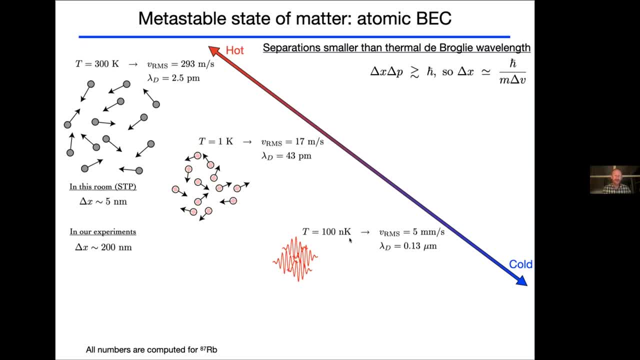 nanokelvin, that's 100 billionth of a degree above absolute zero. finally, the uncertainty in position becomes approximately 130 nanometers, or 0.13 micrometers, which is now comparable to the separation between particles. So that's about room temperature. So in this case we're going to 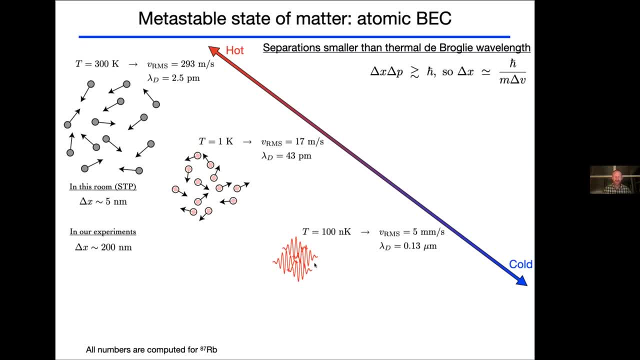 measure the temperature between our particles, meaning that these particles, in the case of bosons, become fundamentally indistinguishable in the form of a phase of matter called the Bose-Einstein condensate And, in cartoon sense, at very, very low temperatures every particle is in. 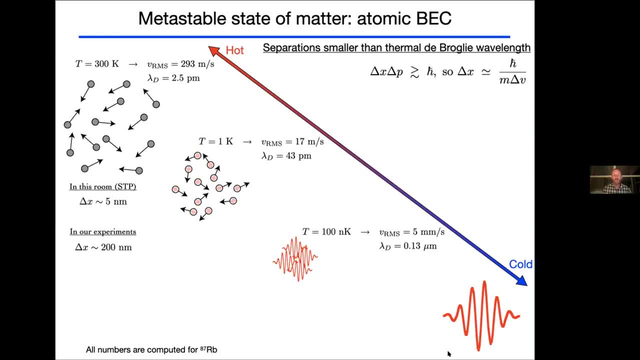 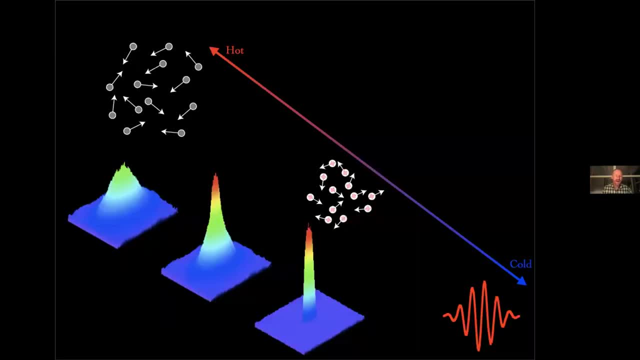 the same quantum state. You can't tell them apart and it's just one big wave that describes the system When we perform these experiments in the laboratory. here is a series of images representing what we see At high temperatures. we have an image of a blob like this: 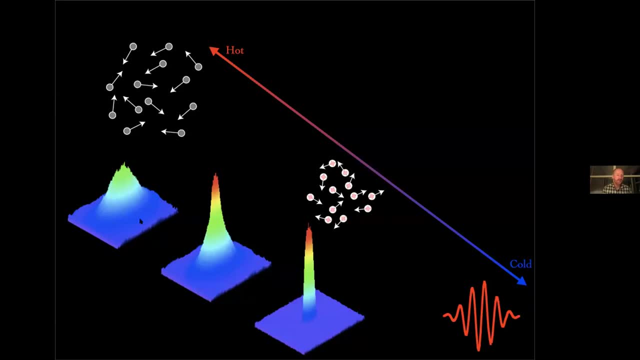 This is the momentum distribution, or velocity distribution, of the atoms. As the system cools, a small peak appears in the center. This is the onset of the Bose-Einstein condensed phase And finally, at very, very low temperatures, virtually every atom is in the same quantum state. 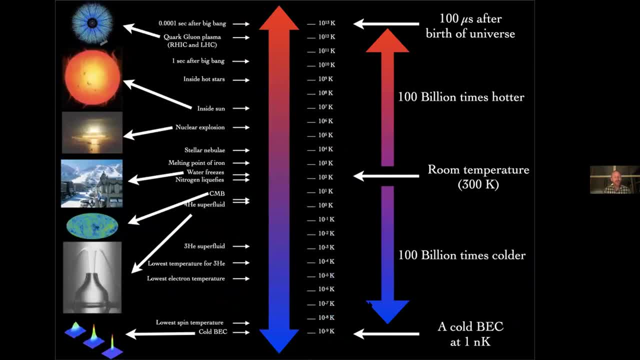 So I use words like nanometer, nanokelvin and kelvin very loosely, but these kind of SI prefixes really disguise the amazing difference in scales that we're talking about. So this is the momentum distribution or velocity distribution of the atoms. As the system cools, a small peak appears in the center. This is the onset of the Bose-Einstein. 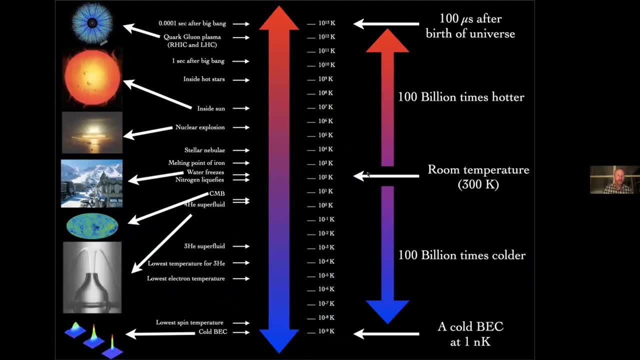 condensed phase. We have a large peak here. This is the momentum distribution or velocity distribution of the atoms. As the system cools, a small peak appears in the center. This is the momentum distribution or velocity distribution of the atoms. So on this graph I've made here, the white arrow here indicates the room temperature of about 300. 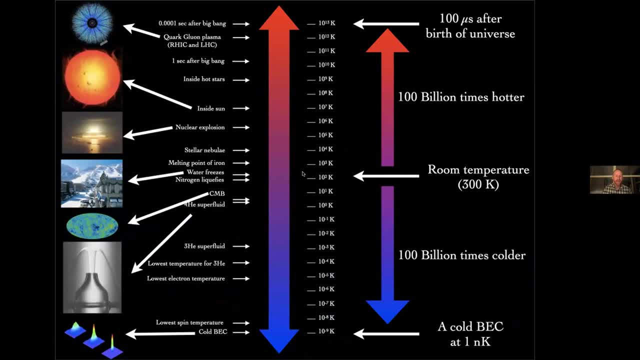 kelvin and for all intents and purposes, on this scale every terrestrial temperature is exactly the same place. So water freezing is 270 kelvin, but for practical purposes that's the same place. Here is a picture of a balmy winter day here in Aspen. only slightly below this On this scale, 77 kelvin, we see the. 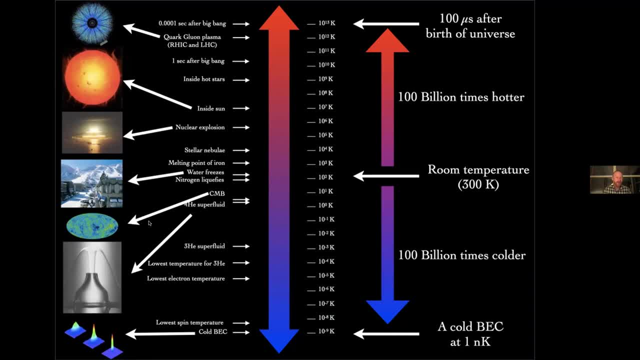 liquefaction point of nitrogen. Below that, on the scale of about 4 or 5 Kelvin, we see the cosmic microwave background And below that we see the superfluid transition temperature of helium, helium-4.. Well below that we see another kind of superfluidity of fermionic helium-3.. 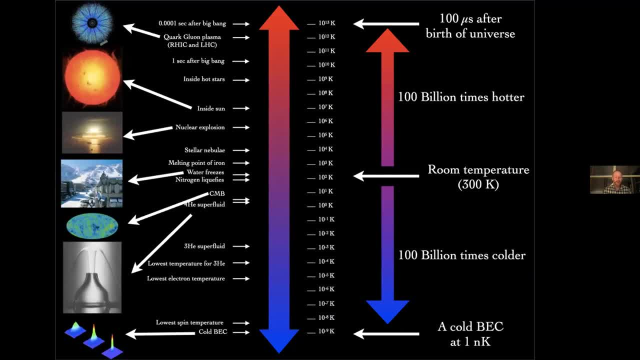 And below that we see the lowest temperature ever recorded for helium-3,, which is only 100 microkelvin. 10 to the minus 4 Kelvin Below. that is the lowest recorded electron temperature ever recorded, which is about 10 microkelvin, That's 10 millionths of a degree. 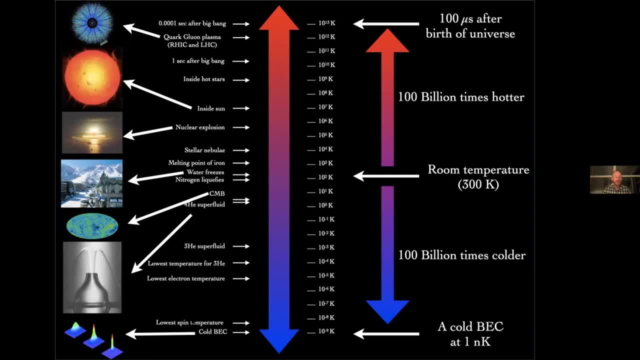 above absolute zero And at these very lowest temperatures- lowest spin temperatures and cold BECs. finally, we reach the 10 nanokelvin scale, So that's 100 billion times colder than room temperature. That's really cold And to put that into perspective, if you go up in temperature, 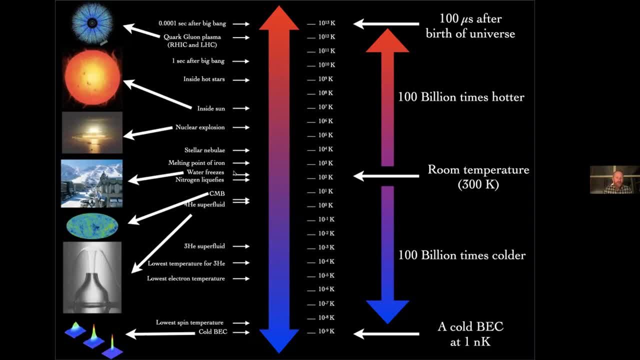 by a similar amount, we see that the difference between room temperature and the melting point of iron is only the width- That's the width of my cursor. Then a stellar nebula, only slightly higher than that, And even sort of the very hottest things we tend to do, you know, in our technological world like 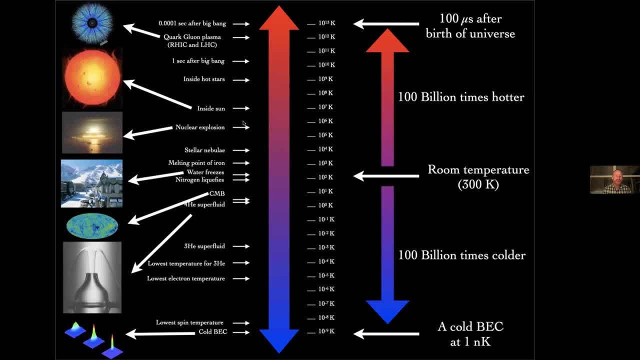 nuclear explosions are only slightly above room temperature on the scale. The inside of the sun is hot, is yet hotter Inside hot stars. we're finally at a billion Kelvin And now we get to sort of really astrophysical scales. A second after the Big Bang we believe the universe was. 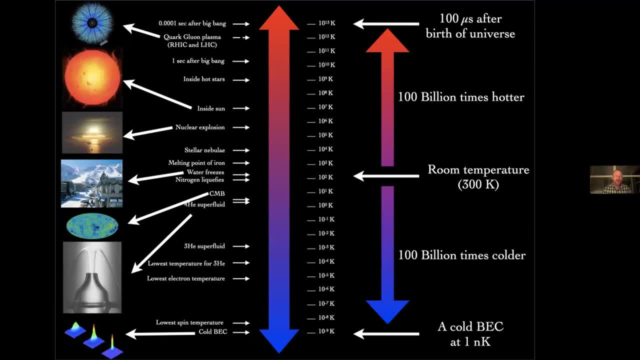 at 1 billion Kelvin And that's really hot, And that's really hot, And that's really hot. So the cold you can see on the right is 10 to 100 billion Kelvin. The hottest temperature that people have created is currently a quark pornography on plasma, both at RHIC and LHC, which is 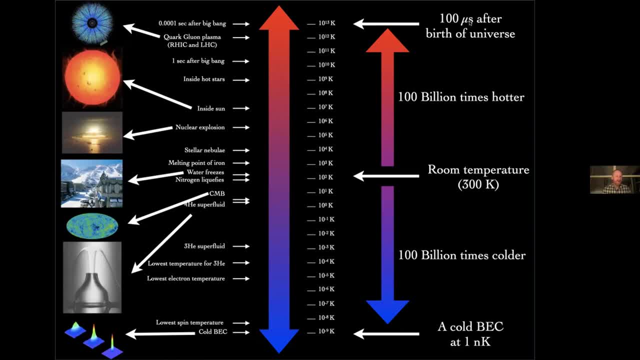 approximately a trillion Kelvin And approximately 100 microseconds after the inception of the universe, the temperature was about 10 to the 13 Kelvin, or 10 trillion Kelvin, which is 100 billion times hotter than room temperature. So the point here is that increase in temperature is 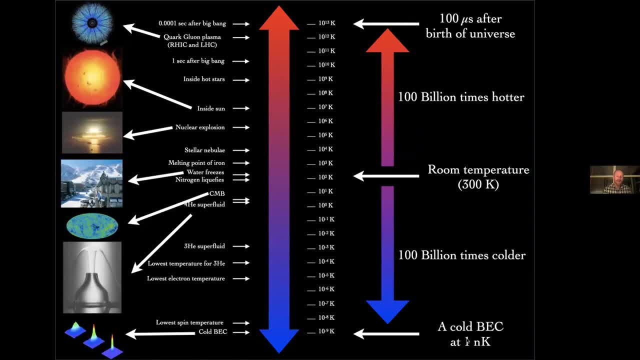 the same fractional increase that we see when we decrease the temperature. And there are two and make a Bose-Einstein condensate of a couple of nanofelvin. So this is an enormous scale of temperatures that scales from ultra quantum to the beginning of the universe. 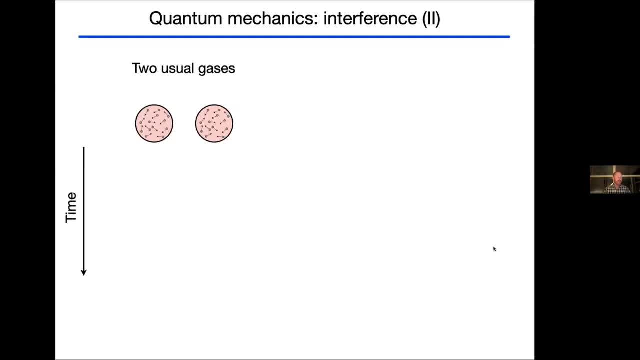 So now I want to turn back to sort of quantum effects. So first, if you imagine two balloons somehow in a vacuum and you were to pop them simultaneously, I think we all agree on what would happen. The gas would expand And at some point this expanded gas would overlap. 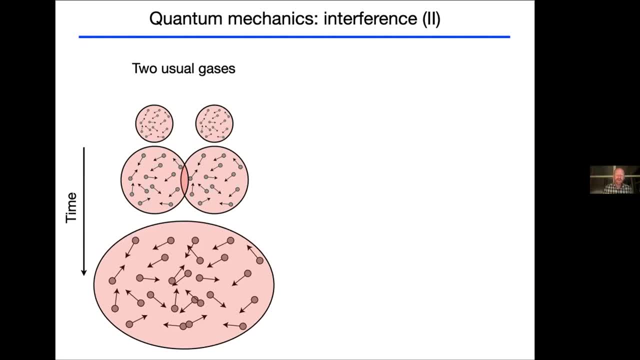 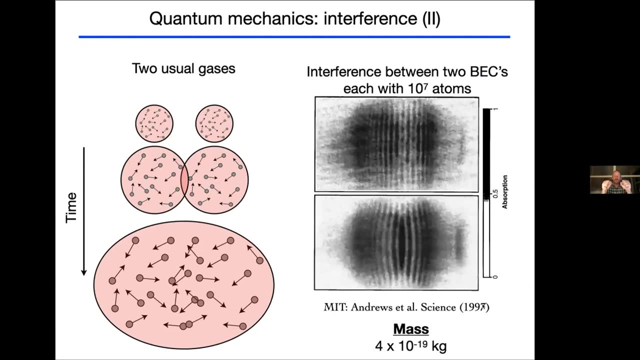 forming a larger ball of expanding gas. But this is not the case with Bose-Einstein condensates. One of the early experiments in the late 90s of BECs consisted of two BECs prepared next to one another, allowed to expand and overlap. 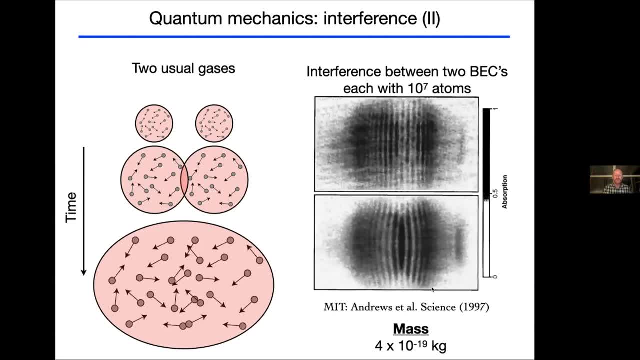 And rather than just overlapping interference fringes formed, just as we saw with light, just as we saw with electrons and even C60. But now this experiment consisted of about 10 million atoms all interfering together, So this is ultra quantum. So, having said that, introduced BECs a little bit. 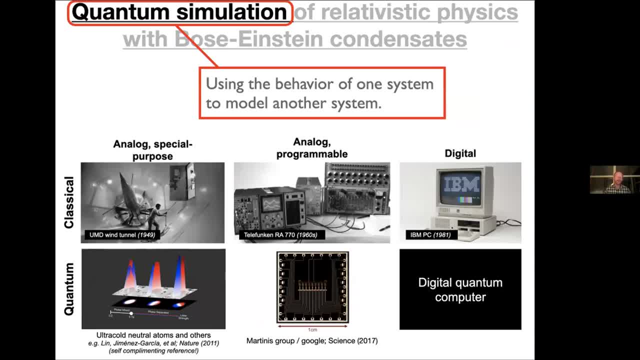 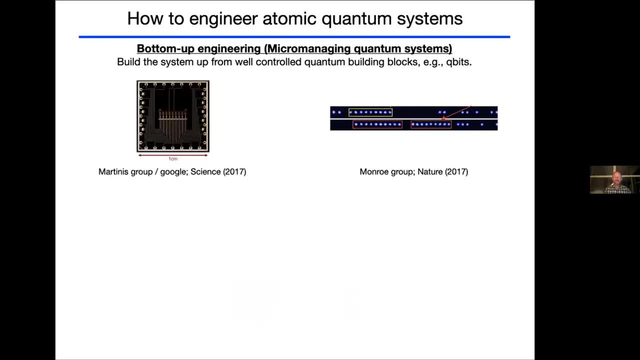 I'd like now to turn to quantum simulation and give a bit more flavor about what I mean by quantum simulation. So when we imagine simulating one system with another, we can sort of envision two paradigms for doing this kind of work. One we'll call the standard, bottom-up engineering. 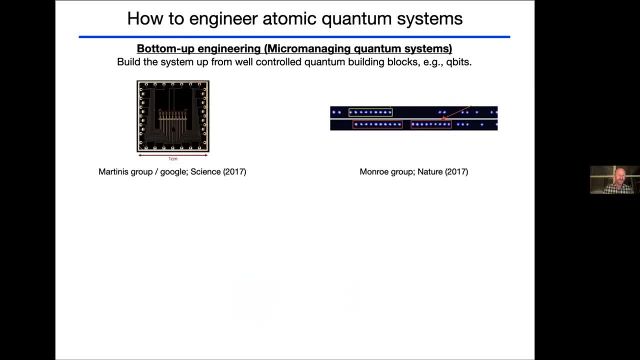 where you get ingredients. These could be quantum bits, for example, qubits, as in the superconducting system or this atomic ion system, And the basic way you do this is you have a certain well-defined number of qubits And you control each and every one of them in such a way. 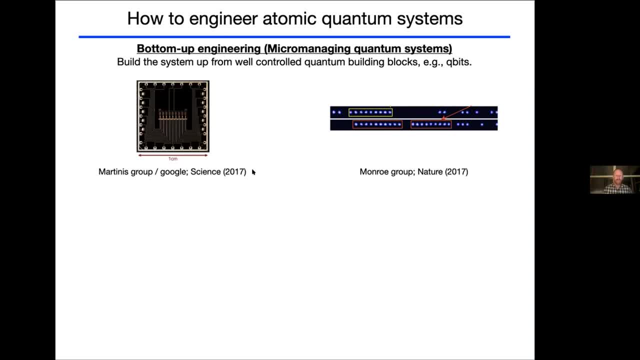 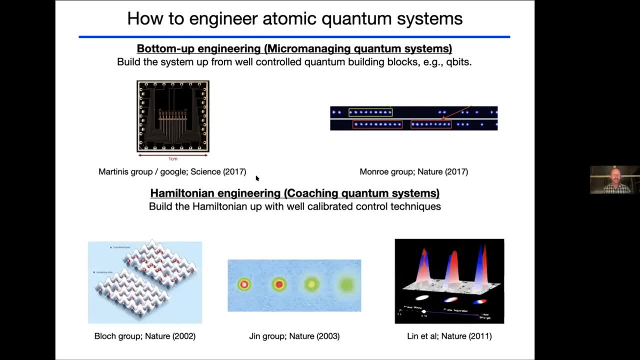 that you can execute the quantum simulation of interest. What I'm going to describe to you today is really very different than that. Technically you'd call it Hamiltonian engineering, But I think a better way to think about it is sort of quantum coaching. 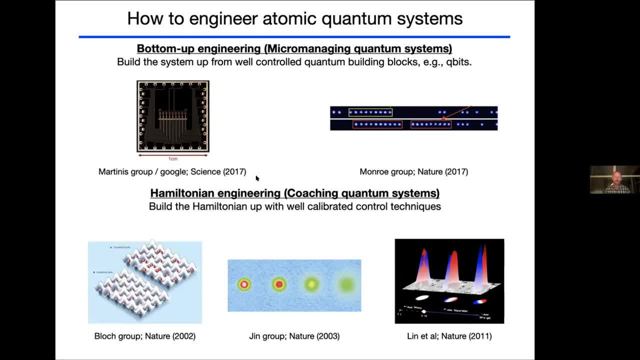 What we're going to do is tell these particles how they should play their game, what their rules are, And we're going to prepare them and let them go And we'll see what happens. So we're going to be simulating a system described. 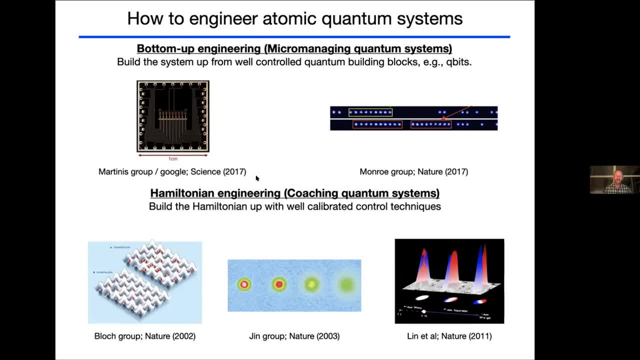 to the rules that the system follows, not by telling each and every particle what it should be doing at every time. So we'll be building up the Hamiltonian, That is, the rule book, using well-controlled and well-calibrated techniques. The three examples pictured at the bottom: 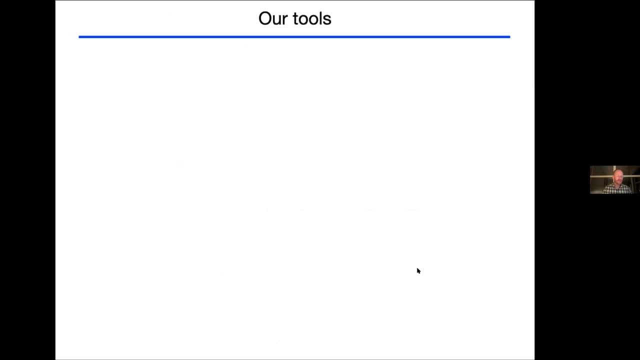 will be the ones I describe on the next slide. So the first such example is what I'll call an optical lattice- Now, this is a fancy way of saying an energy landscape, such as a hilly landscape. I've pictured here that the quantum particles can move about in or even tunnel. 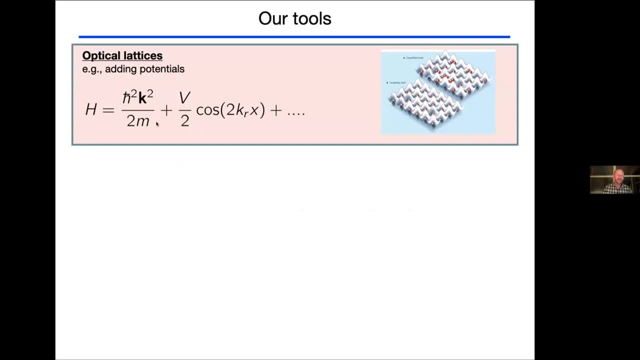 quantum, mechanically, through barriers within, And we describe that by an energy. What I'm picturing here is an optical lattice formed by the interference of two laser beams, just like I described before, just like the double-slip pattern I showed earlier. that gives a standing wave of intensity. 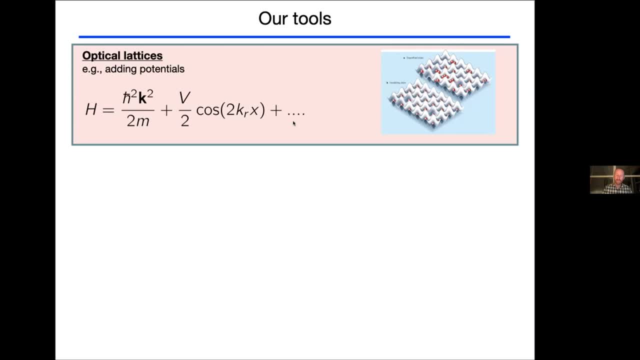 And the atoms are trapped by the standing wave of that intensity. A second thing we can do that I will not be using in this talk is interaction tuning. We can in fact determine, by using a tool called a Feshbach resonance, how strongly atoms either attract each other. 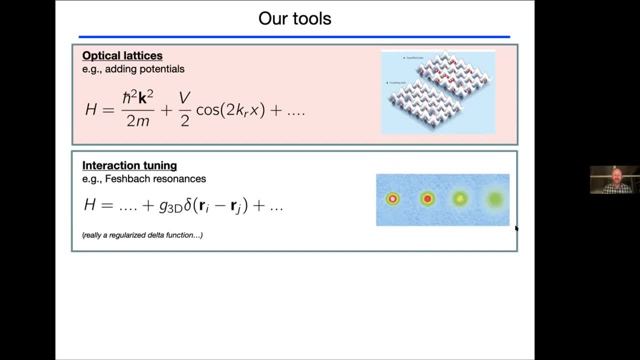 or repel one another, And the picture I'm showing you here, the picture I'm plotting on the right, is a really cool piece of data. It's showing a transition from a. I'm going to actually go from the right to the left. 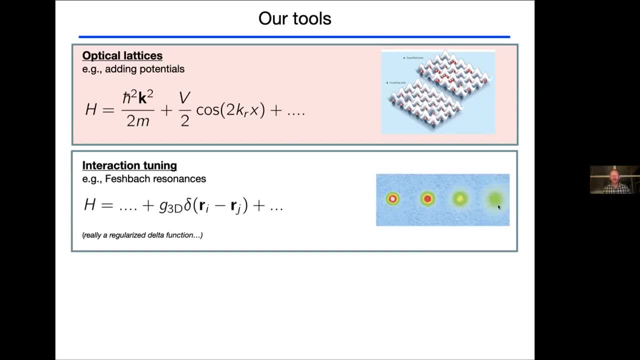 On the right. this is a gas of fermions. These are the particles, like electrons, that tend not to occupy the same quantum state, But if these are made sufficiently strongly interacting, these particles, these fermionic atoms, can bind, forming composite particles that are bosons. 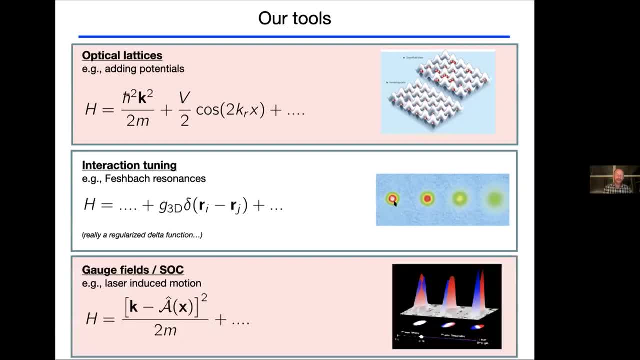 And these bosons can both condense. The last tool I'll be using a little bit today is what are called gauge fields, And this is a little bit more nuanced than anything I've described before, But an example of a gauge field in everyday life. 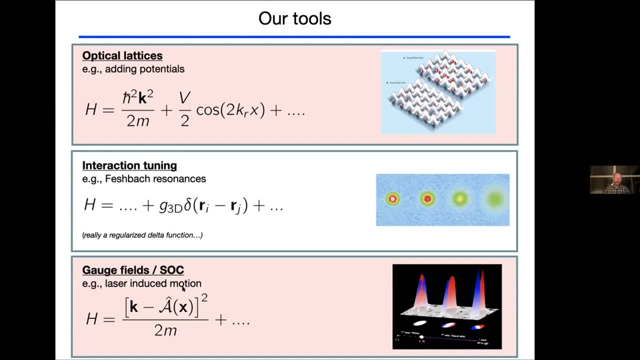 might be a magnetic field, And a magnetic field is something that, for example, if you have a uniform magnetic field and have a charged particle move in it, its velocity will stay the same, but its momentum will change. It will undergo circular cyclotron orbits. 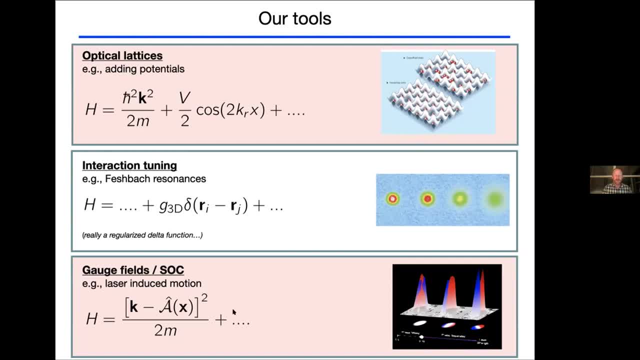 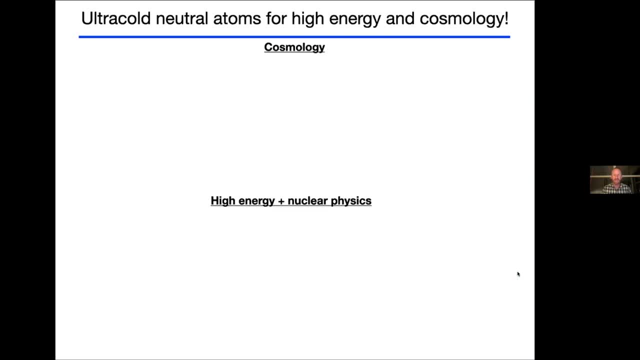 And mathematically this is represented as a change to the kinetic energy part of the rulebook, or the atomic Hamiltonian, And I'll give some graphical interpretation of this as needed later. So this is a gauge field, So that said, a coal. atoms have been doing quite a lot. 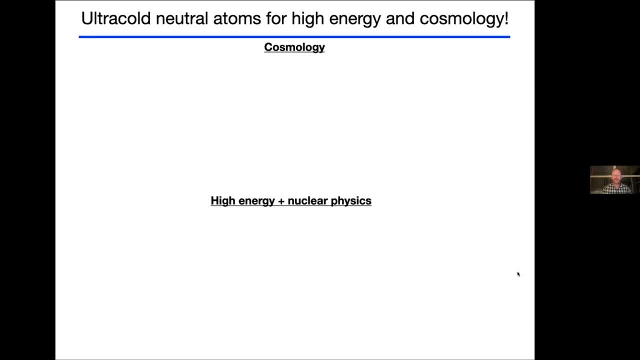 actually of simulations of high energy and cosmological physics beyond what I'll describe today. So, for example, moving barriers in Bose-Einstein condensates have been used to emulate black hole event horizons and even image Hawking radiation in that system. 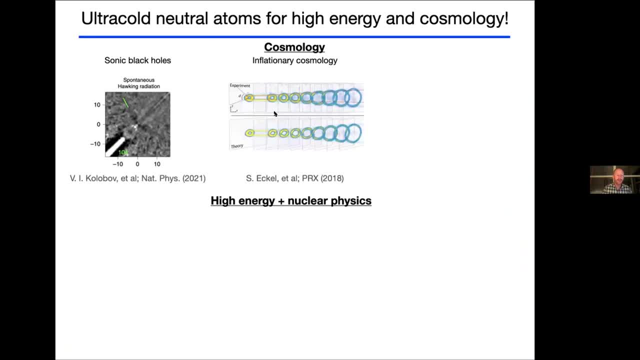 In an experiment that I've done in collaboration with Gretchen Campbell and Steve Eckel, we studied expanding ring-shaped Bose-Einstein condensates, which are roughly analogous to a brief period of inflation in the inflationary epoch of the universe. A similar experiment by Chang-Chin's group. 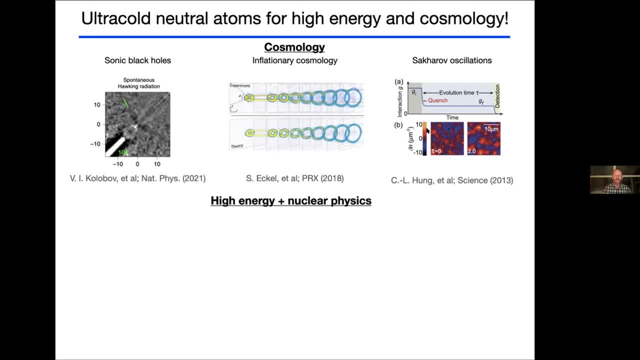 changed the interaction strength of the system, which is very much like expanding a system, and observed the cosmological effect called Sakharov oscillations In the high energy and nuclear context. strongly interacting systems of fermions, in this case lithium 6, have analogous equations of state. 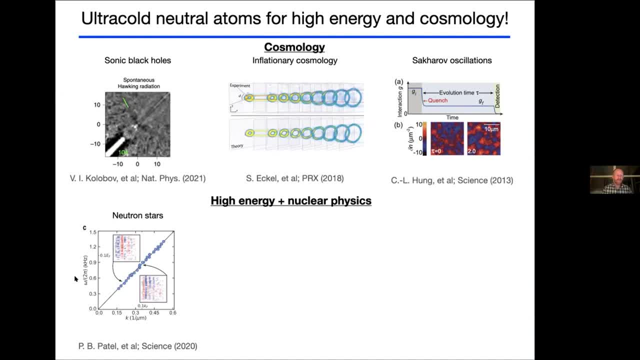 that is, analogous Hamiltonians to the certain parts of neutron stars, owing to the very, very strong collisions between neutrons as well. At higher temperatures, the same fermionic system has properties analogous to the quark-gluon plasma I described earlier. at extremely high temperatures, the 10 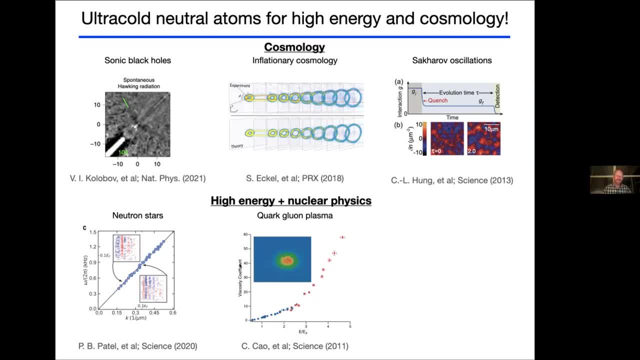 to the 12 Kelvin example And both of these systems. the system has a viscosity, given by a quantum of viscosity that can, in fact, also be predictive for a string theory. And lastly, today I'll be giving examples of relativistic physics. 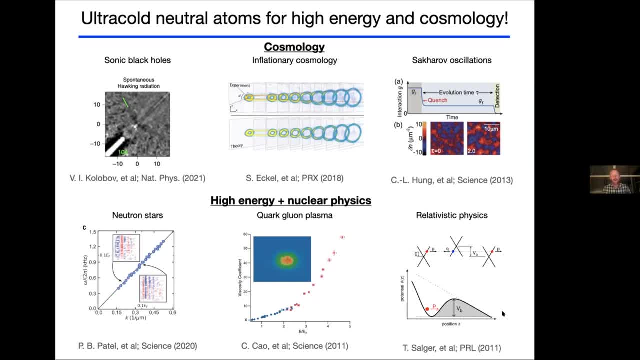 The data I'm plotting here in fact is from Martin Weitz's group, and I'm just putting this up to indicate that, although I'll be describing my group's research, there are other teams as well who have been looking at relativistic physics. 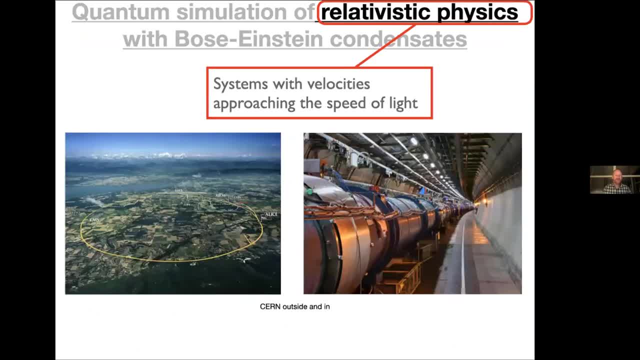 with bulldowns. So then, turning to relativistic physics: systems with velocities approaching the speed of light. for the purpose of this talk, I'd like to go a little bit more into detail about what I mean, And I'm going to take a little bit of time on this graph. 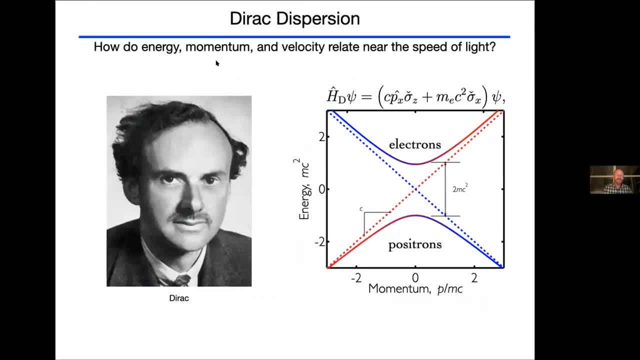 So what I'm plotting is the relationship between energy, momentum and velocity predicted by Dirac at the beginning of the quantum era for relativistic particles. So what this graph is showing you is energy on a vertical axis, plotted as a function of the momentum of a particle. 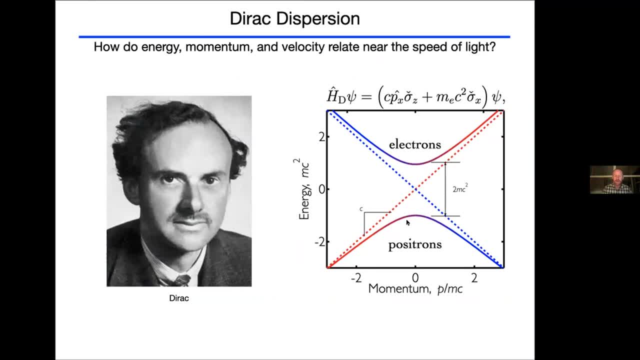 So what we first see- and this should be familiar- is if you're at zero momentum, the energy isn't zero. And if you go up from zero, you'll see it's exactly the rest mass of the particle, mc squared. That's a familiar equals mc squared. 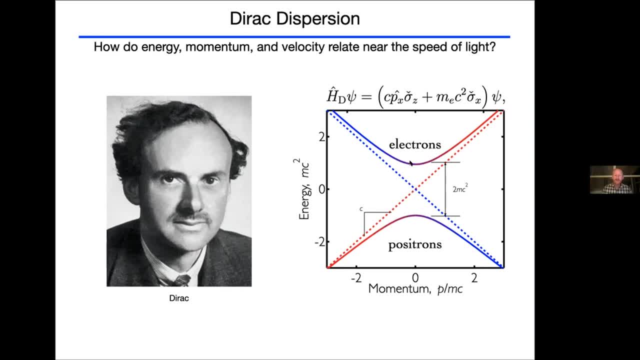 for a non-moving relativistic particle. But as you begin to accelerate the particle, you'll see that the momentum changes and the energy increases, But it increases in a peculiar way, And this peculiar way can be understood by thinking about these straight lines. 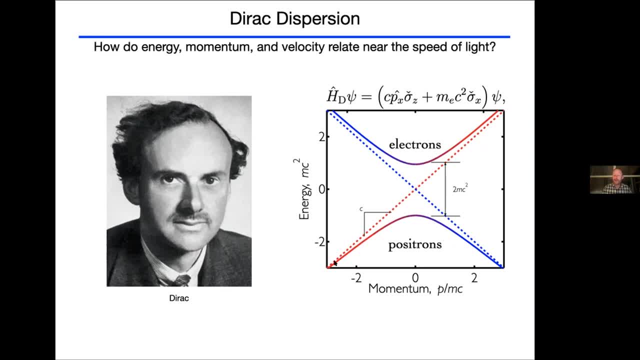 These straight lines are plotting the energy momentum relationship, not for electrons, necessarily, but, for example, for light, And what you should remember is that light, no matter what its momentum, always has exactly the same speed, of course: the speed of light. 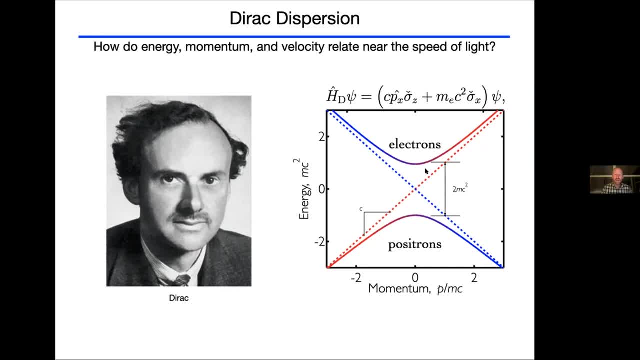 So what this is telling you is that the slope or the angle of this line is the thing that's telling you about the velocity, not the momentum. So if we turn back now to these relativistic electrons, what you'll see is that at zero momentum, the slope is zero. 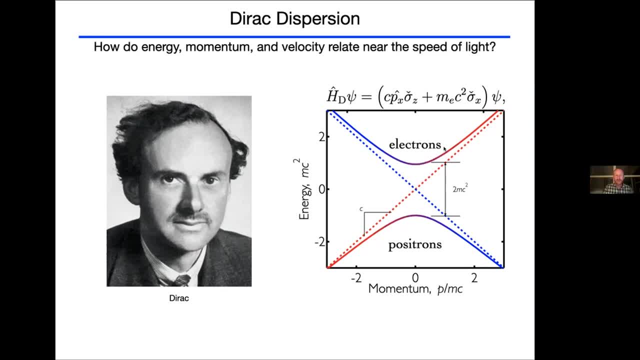 And as you begin to increase the momentum, this relativistic curve approaches the curve given by the speed of light of these massless particles. And this is exactly telling us that these relativistic electrons will never be moving faster than the speed of light, although they 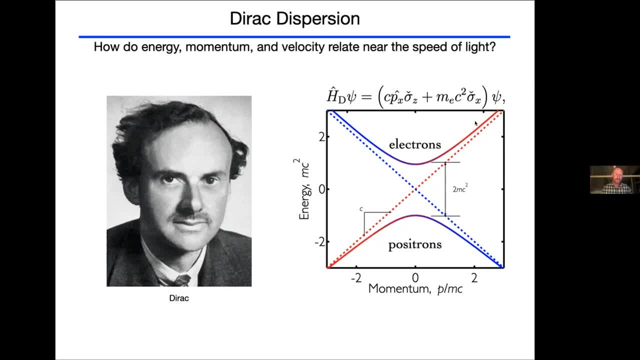 will get incredibly close to the speed of light, And this is exactly what we're going to see. We're going to talk a little bit about equations like this, but it's certainly not essential for understanding the talk. OK, so the thing to see here is there's. 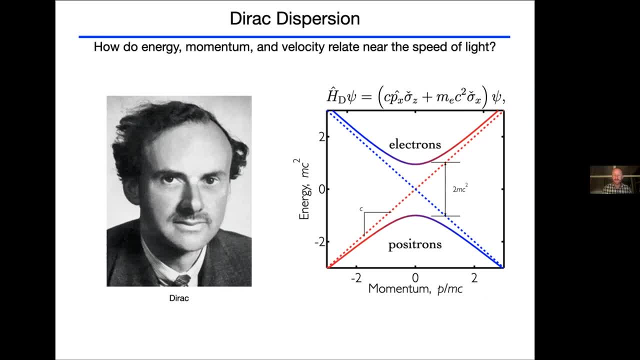 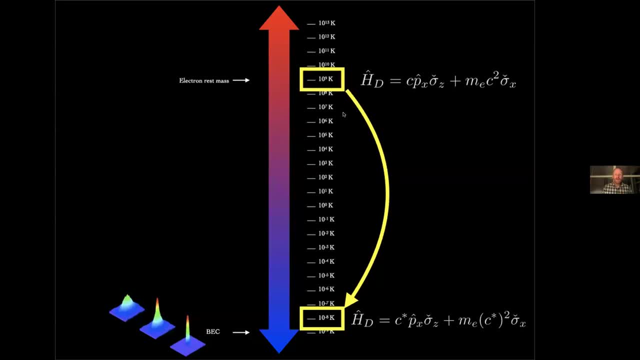 an electron mass and a speed of light. All right, so why did I bother showing an equation? Well, what we're going to be doing in the experiments I'll describe is taking the physics associated with the electron rest mass, which has associated the temperature of about a billion Kelvin. 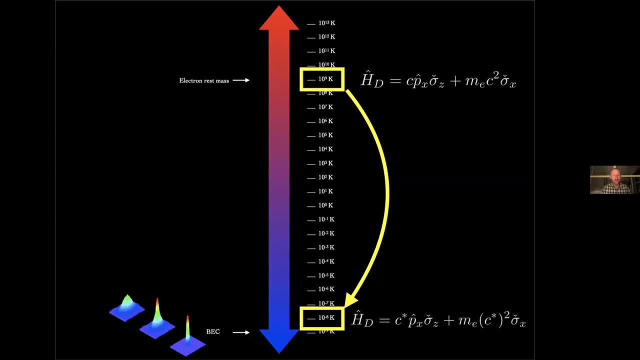 and we're going to be transporting that physics down this ladder of energy to the about 10 nanokelvin scale where we do our cold quantum experiments. And the point is that the equation describing these systems, this Dirac equation- 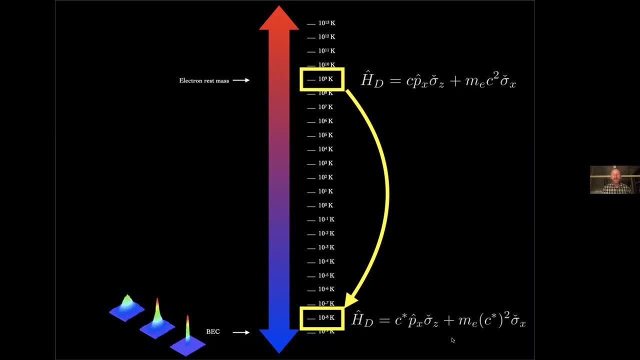 can be an equation that's identical on both of these scales, except that the speed of light can take on a different value and the electron mass can take on a different value, And I think this is one of the really important things we should understand about physics. 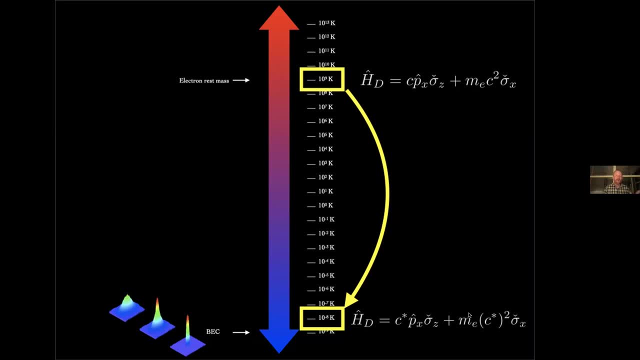 is that if something is described by the same equations, no matter what the scale, it will exhibit the same phenomena, whether we'd be talking about 10 billion Kelvin or 10 degrees above absolute zero, All right. so I would like to get more specific. 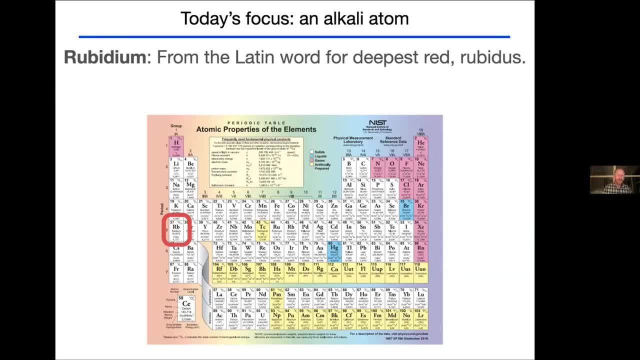 and tell you a little bit about the system that we're actually realizing. So we're going to be looking at Bose-Einstein condensates of alkali atoms, That means the atoms that are here on this first column of the periodic table, Every atom except the radioactive francium. 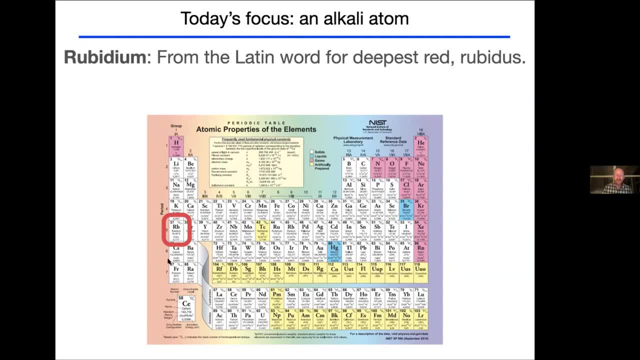 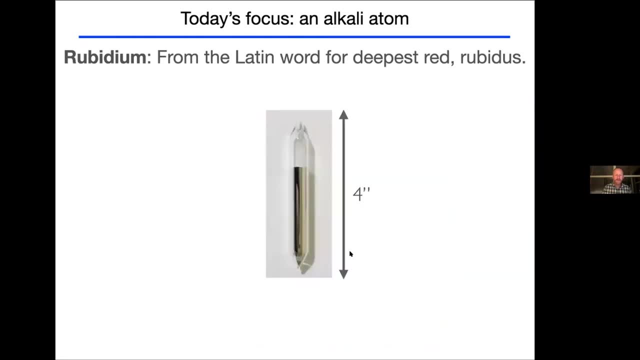 in this column has now been brought to quantum degeneracy. That is either a degenerate Fermi gas or degenerate Bose gas, a BEC. We'll be focusing here on rubidium. If you go, purchase rubidium, an ampule like this, or rubidium- 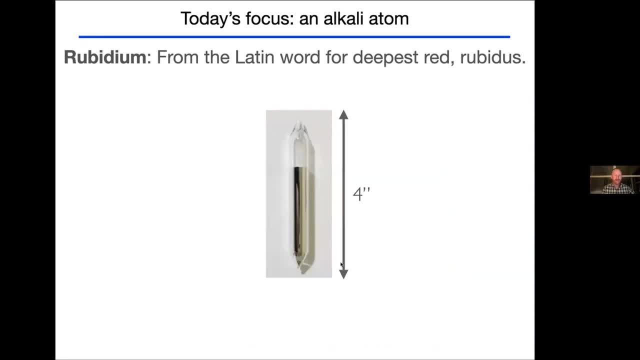 will run you about $100.. It's about four inches long, which should be about the size it actually is on your screen, And we'll get to why it's called red in a second. This is not a Bose-Einstein condensate. 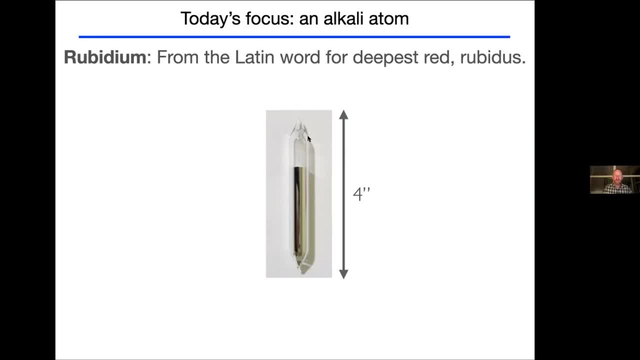 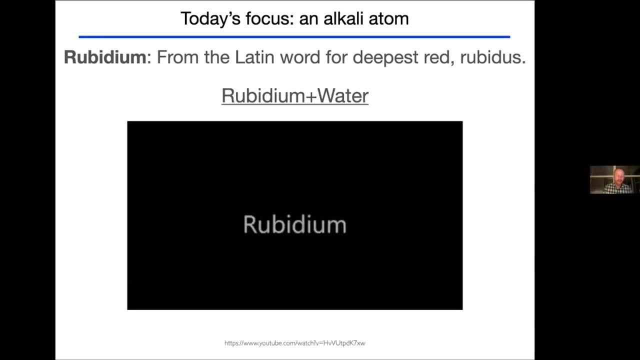 This is a chunk of metallic rubidium. It will melt just above the temperature of your hand- about 45 or so Celsius- And, as you can see by this YouTube video, it is highly reactive, which has nothing whatsoever to do with making Bose-Einstein condensates. 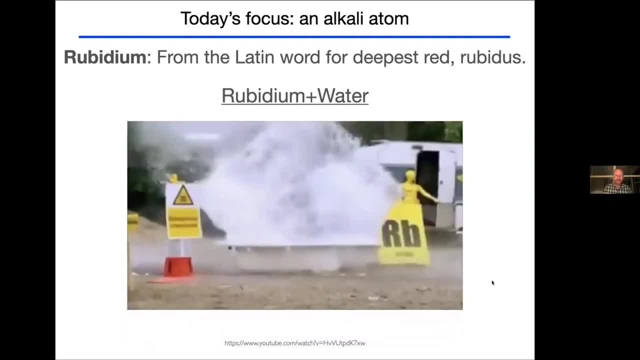 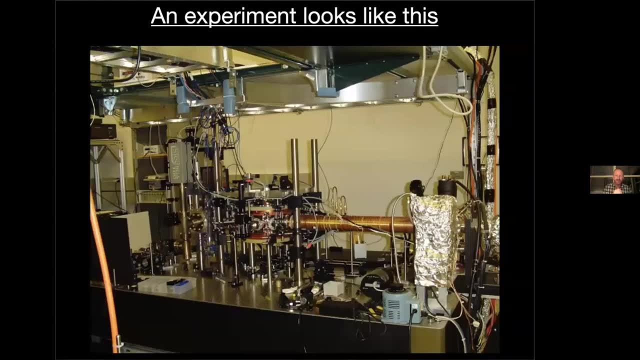 but it's pretty cool. In fact, we make Bose-Einstein condensates in apparatuses that look more like this. Starting on the right side of the graph, this is what we call an oven that heats up the rubidium from room temperature about 30 Celsius. And this is what we call an oven that heats up the rubidium from room temperature about 30 Celsius. And this is what we call an oven that heats up the rubidium from room temperature about 30 Celsius. And this is what we call an oven that heats up the rubidium from room temperature about 30 Celsius. 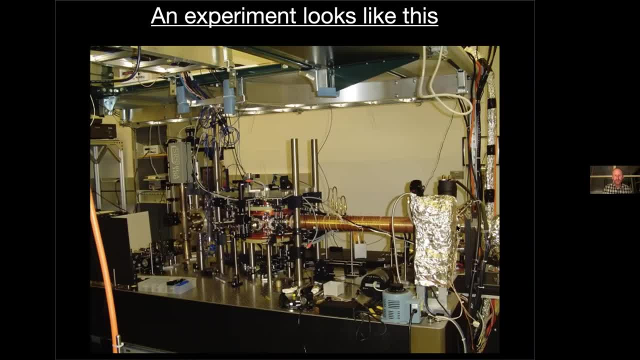 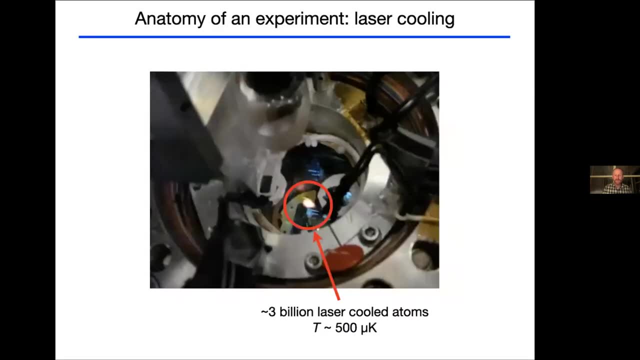 To 100 to 130 Celsius. that makes an atomic beam of this reactive metal propagating in this tube, where it's captured by laser forces. Here's an image of a cloud of atoms encircled there that has lasers shining on it from all six. 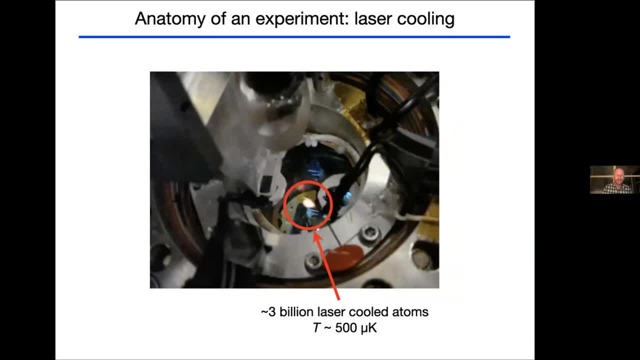 of the Cartesian directions, essentially compelling the atoms to stay in one place and simultaneously cooling them to actually quite low temperatures. This is 500 microcouplements, that's 500 millionths of a degree above absolute zero, And roughly speaking, that ball of atoms has about 3 billion atoms in it. 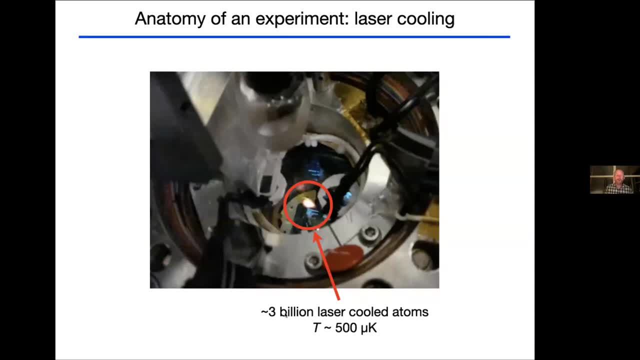 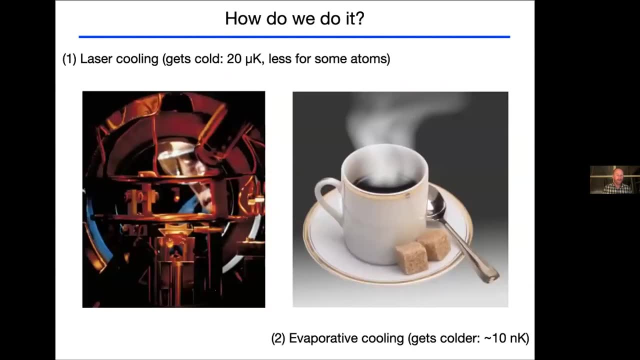 So in these experiments then, we start with a hot source of atoms. We slow them with a laser beam and capture them in this trap called the magneto-optical trap. We then evaporate to them, We take, grab the atoms and we eject or throw away. 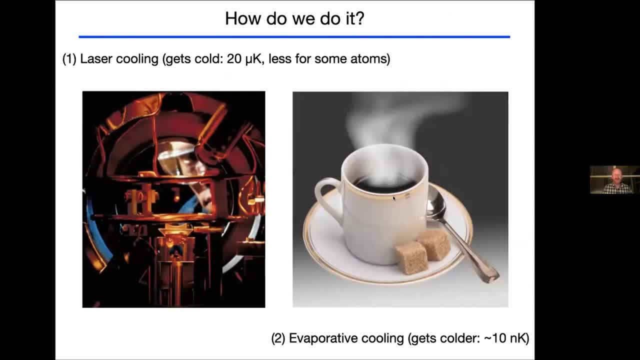 the most energetic or, if you wish, the hottest atoms, just like your coffee cup throws off the most hot atoms or molecules of water inside that coffee, Lowering the temperature We evaporate to be cool then, from this sort of a hundred micro Kelvin temperature. 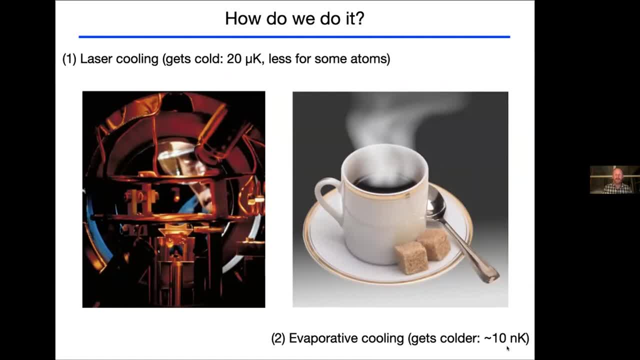 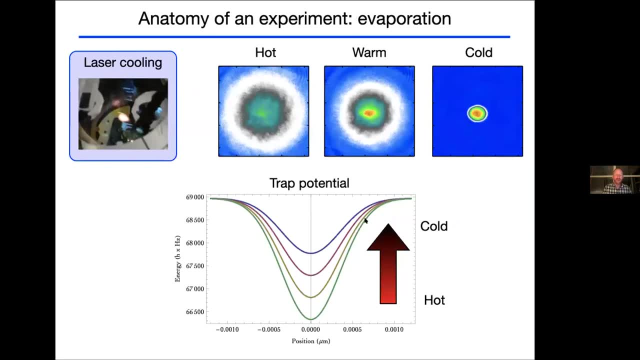 to the nano Kelvin scale, just 10 or so billions of a degree above absolute zero. And the way you can picture this process is holding the atoms in a trap like this and simply making the trap shallower, So you dump out the particles with the highest energy. 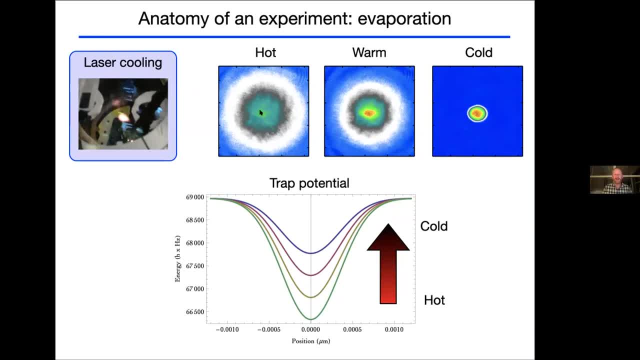 giving images similar to what I showed you before, from a gas that is not a Bose-910 condensate to one that's partially condensed to a nearly pure BEC. All right, so with that sort of introduction about the physical system we've been looking at. 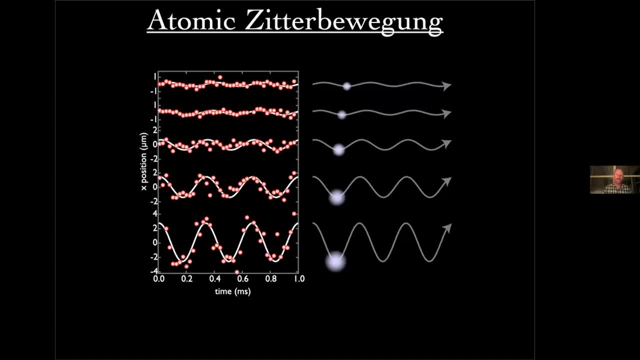 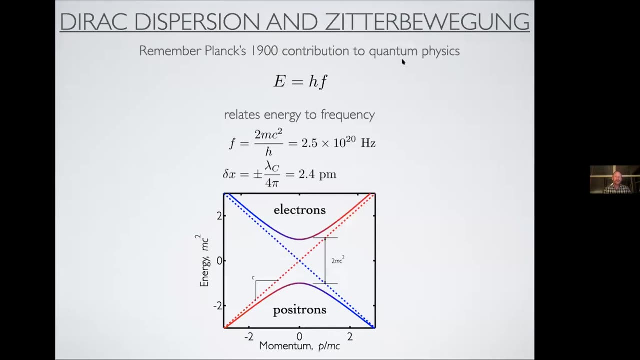 I'd like now to turn to the quantum analog simulations we've actually been performing. The first one I'll describe to you is atomic Zitterbewegen. This is the microscopic trembling motion that a fundamental electron is predicted, under certain circumstances, to undergo. So when I give you the scale of Zitterbewegen, 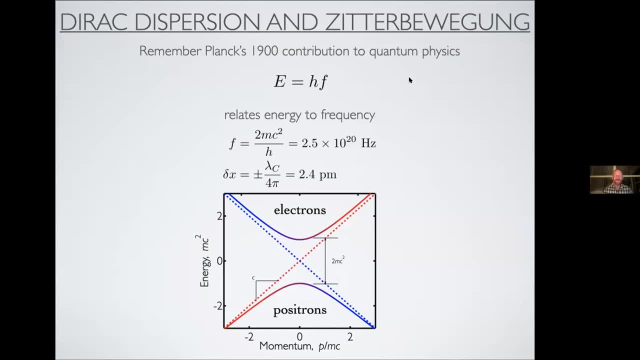 it's useful to think of Planck's 1900s or so contribution to quantum physics, Which is Planck's constant H, And what this constant does is relate a frequency to an energy. Now remember, H is an incredibly tiny number, of the scale of 10 to the minus 31.. 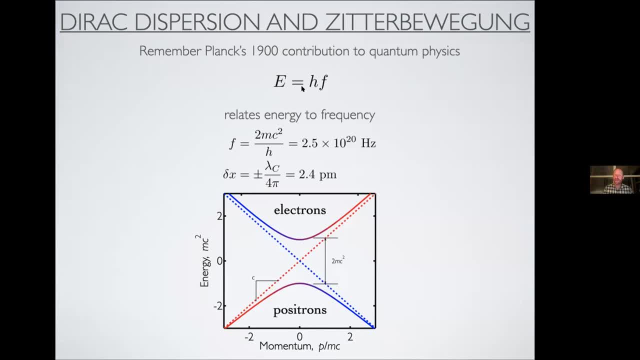 So you need to have. unless you have very, very large frequencies, these energies will tend to be very small. One energy we can think about that I mentioned before is the rest energy of these electrons. So the rest energy of an electron is about half a mega electron volt. 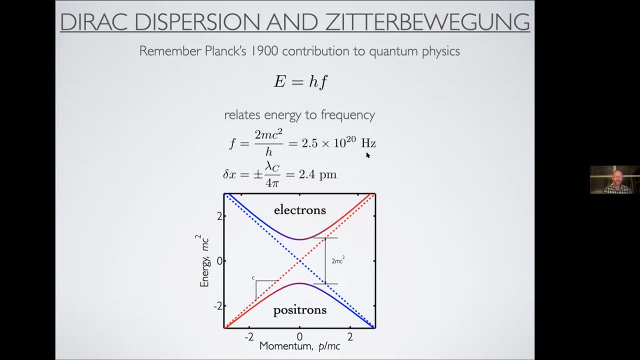 And that corresponds to a frequency that is astonishingly big. it's 2.5 times 10 to the 20 Hertz right. So that's 20, 25 billion billion Hertz 250.. So it's incredibly large number. 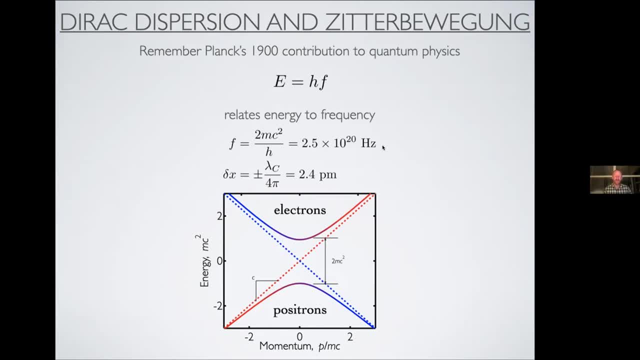 We have no devices in any sense that can measure frequencies on that scale. Similarly, the scale under which electrons might undergo Zitterbewegen is about 2.4 picometers. Now what does a picometer even mean? A picometer is about a 25th or so. 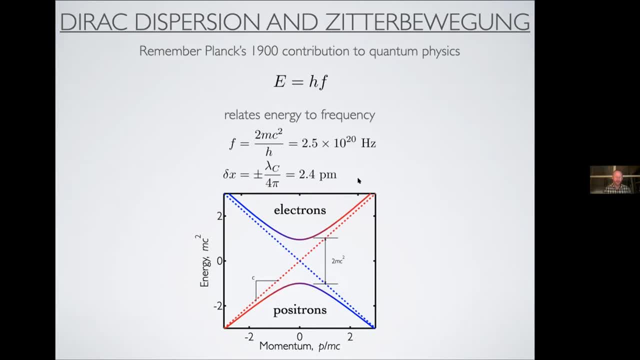 the size of a hydrogen atom. So we would need to resolve micro motion on the scale of fraction of a hydrogen atom in size on a scale of frequencies of billion, billion Hertz, And this is completely out of the question of any technical experiment. 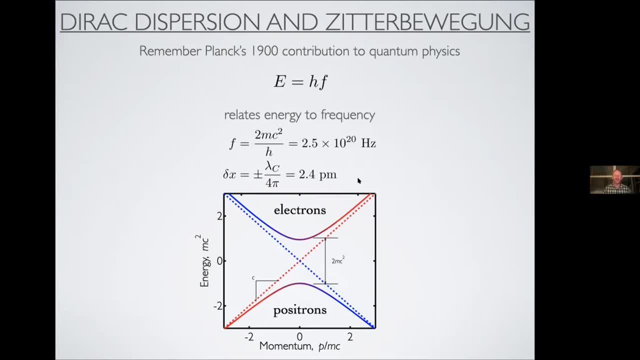 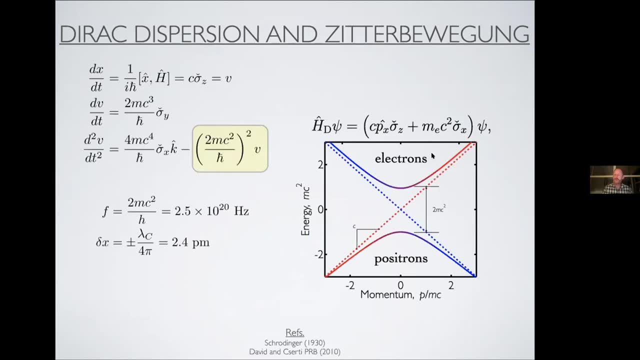 And for that reason, even in principle, the phenomena of Zitterbewegen had gone unobserved. This is my one slide for the specialists in the audience. So what does Zitterbewegen come from? Well, it comes from computing, the Heisenberg equations. 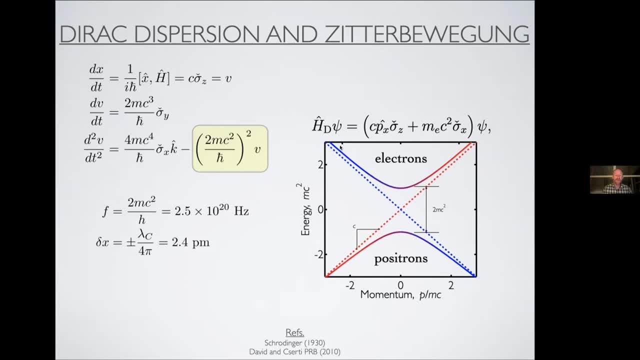 of motion for particles given by this Dirac dispersion. And simply by computing the second derivative of velocity, we see, indeed, there's a second order differential equation for velocity, meaning the velocity and therefore precision will undergo oscillatory motion with frequency given exactly by these expressions. 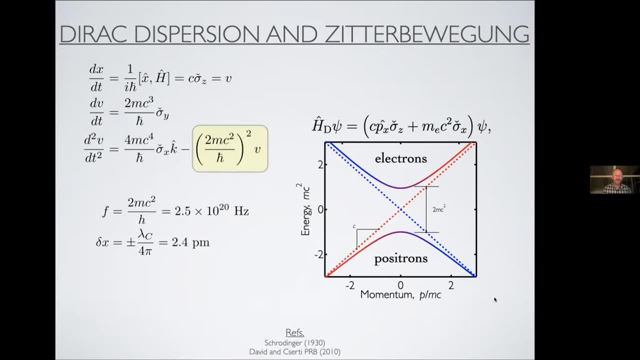 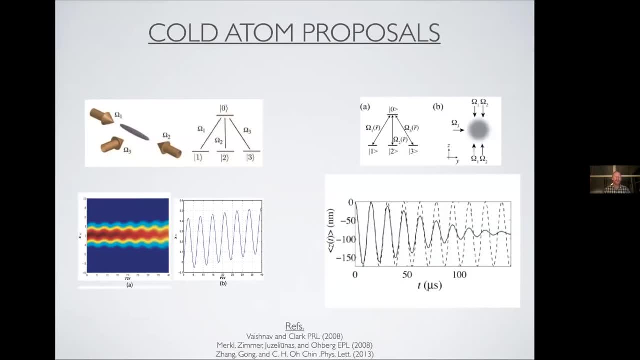 All right. so that's what's going on, And now let's talk about doing it. Well, I was inspired by a series of called Adam proposals, both of which used what I mentioned earlier- gauge fields to create a Dirac dispersion. 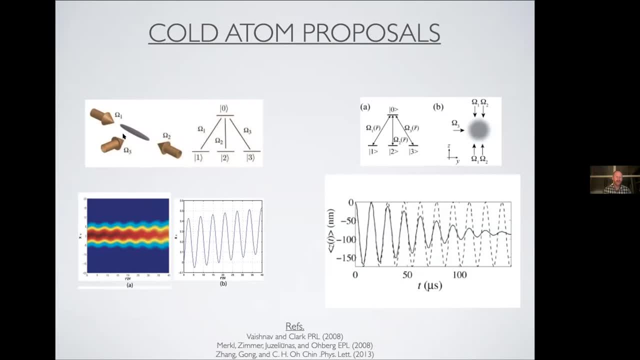 So what these graphs are telling you is that we have a cloud of cold atoms and we're shining a bunch of lasers on them, And for the purpose of this talk, that's really all you need to know. And in both cases, the theoretical prediction is a system. 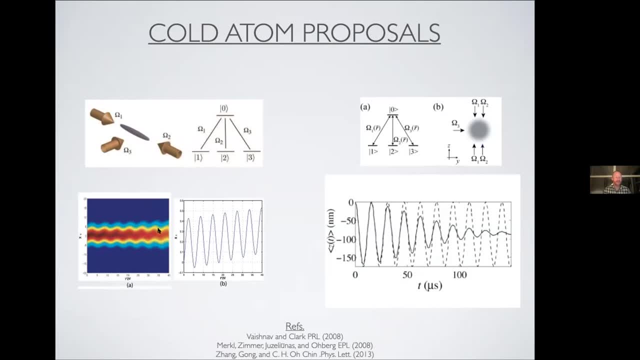 if you just looked at where it is, should undergo an oscillatory motion, which is exactly the Zitterbewegen effect. So let me tell you in pictures: this is the Zitterbewegen effect, which is exactly the Zitterbewegen effect. So let me tell you in pictures: 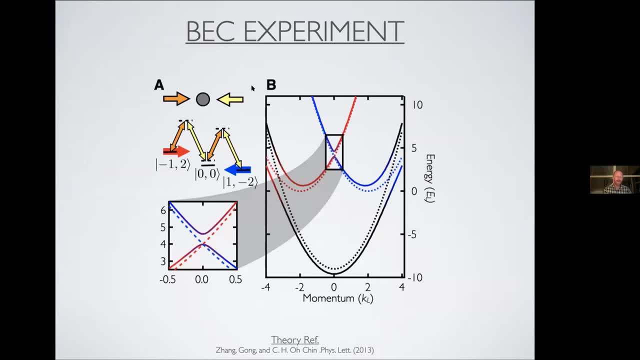 how we did this. So what I'm showing you here is again, energy on the vertical axis and momentum on the horizontal axis, And this is the energy momentum relationship that we get if we shine a certain combination of lasers on the atoms that couple together different spin states of these atoms. 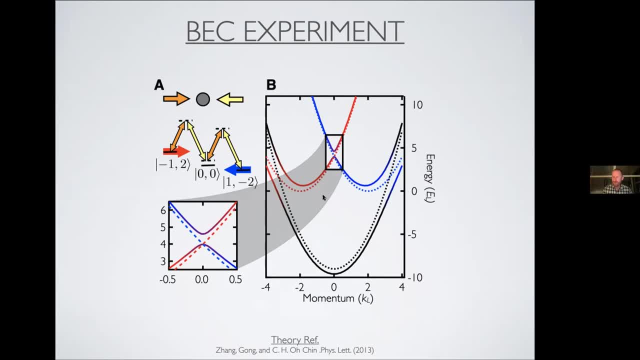 And you'll look at this and say, well, that picture is both confusing and it looks like it has nothing whatsoever to do with the Dirac dispersion. And the idea is: well, if you zoom into this black rectangle, if you zoom into this black rectangle, 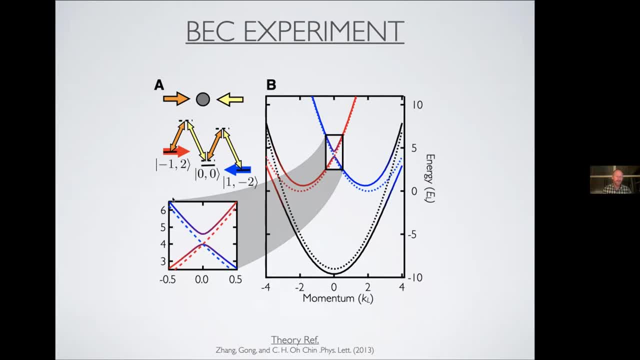 you'll see that in the general vicinity of that rectangle the energy momentum relation becomes indistinguishable with the Dirac dispersion. Remember the gap in this gives the mass and the slope. the angle of this curve up here tells you what the effective or rescaled speed of light is. 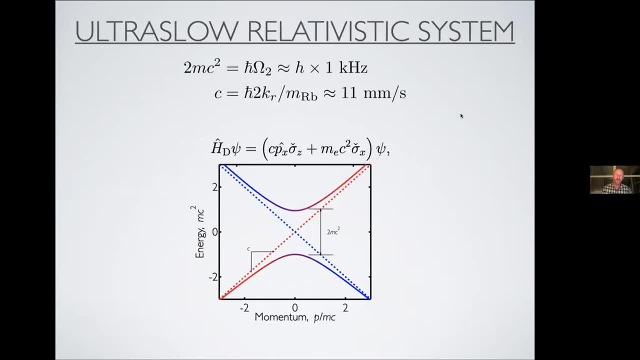 And in this case we have engineered an ultra slow relativistic system. So first, the scale of the rest mass, or the frequency associated with it, is just a couple of kilohertz. Remember kilohertz, that's an audio frequency. So if we compare that, for example, 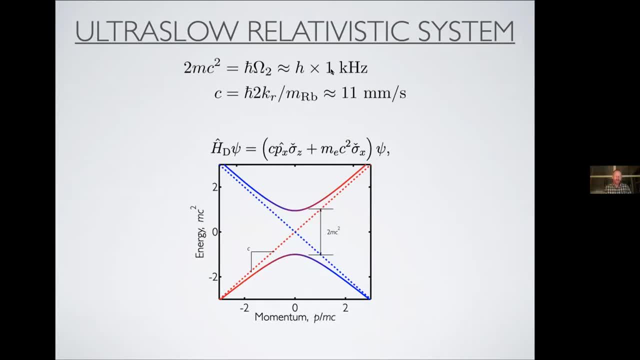 to middle C, which is 440 Hertz. it's living right in the middle of the piano. You could hear this experiment. And the second thing is: what velocity are we talking about? Oh well, this velocity has been scaled down to 11 millimeters per second. 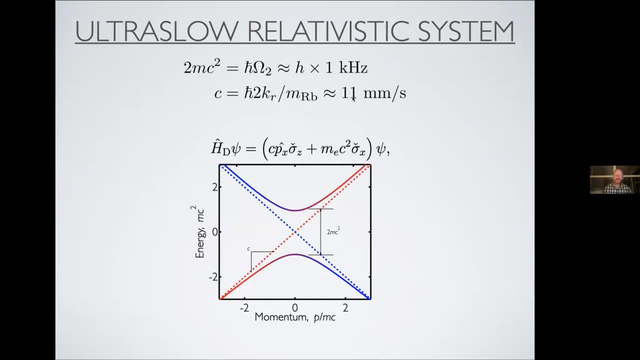 I mean, that's sort of your hand moving about this speed. That's a completely terrestrial scale. So what we've done, then, is taken physics of Zitubo-Vegu and transformed or transduce it to a scale where we can perform experiments in the laboratory. 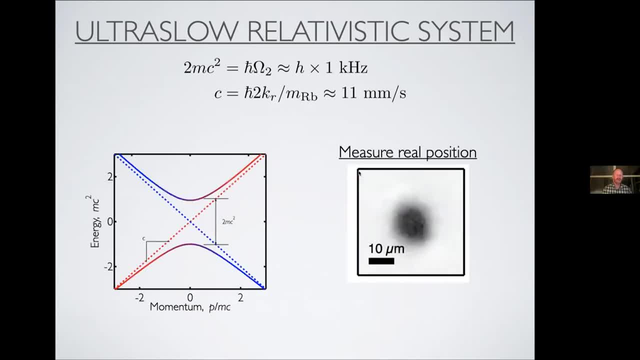 And what do we do? Well, we engineer this environment and we're going to literally measure the real position of these atoms. So here's a cloud of atoms, And the size of this cloud of atoms is is about 10 micrometers. 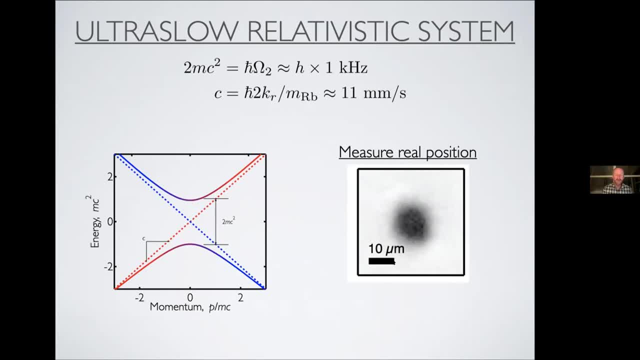 And to give a sense of scale, that's a 10th or seventh or so of the diameter of a typical human hair. So it's small, but it's not really small, And this is a typical microscope image of such a cloud of atoms. 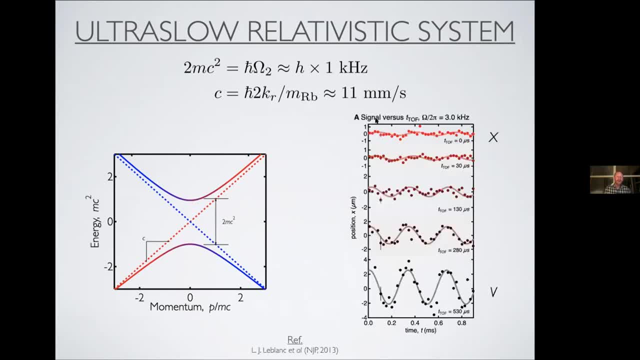 So we performed that experiment. We initialized atoms according to this direct dispersion relation and let them just do their thing. We're coaches. We gave them a set of rules and allowed them to follow the rules, And indeed in this experiment by Lindsay LeBlanc, 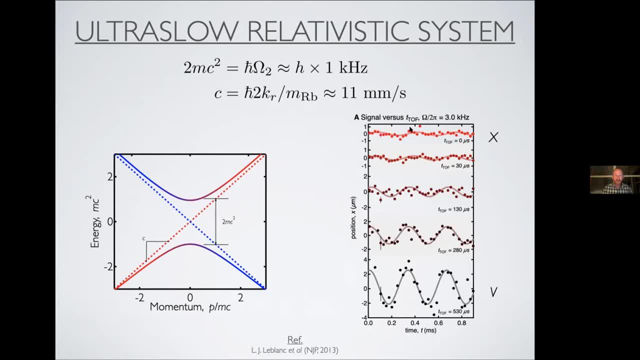 when she was a postdoc in my group, directly showed the Zitubo-Vegu oscillation, both in terms of position as well as velocity. So we directly then measure Zitubo-Vegu, observe Zitubo-Vegu at the expected frequency. 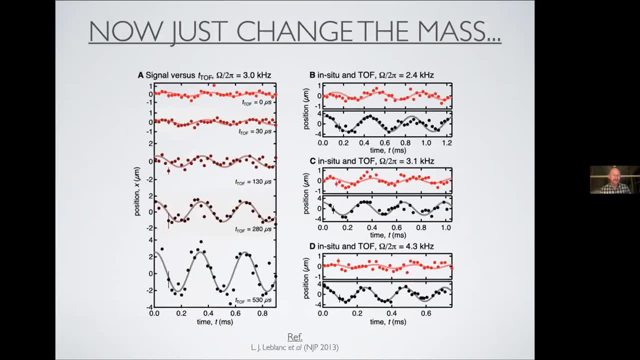 And then we can do some things that are just not really practical. in real high energy physics, For example, we can change the mass of these particles. That just involves changing the light and the intensity of our laser beams. So, for example, this is what I showed you before. 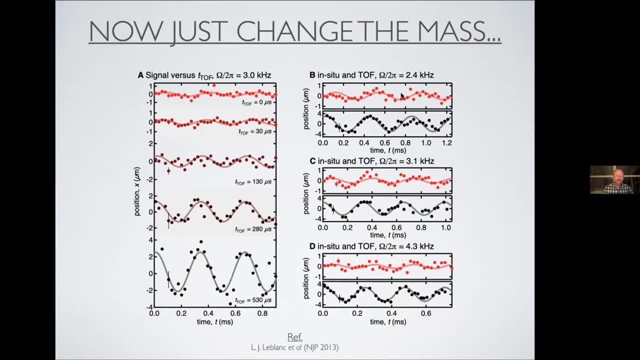 We can change the mass, We can increase the mass And what you'll see is the frequency of these oscillations are going to be increasing as we increase the mass, exactly as you're expecting from the Zitubo-Vegu effect. Okay, 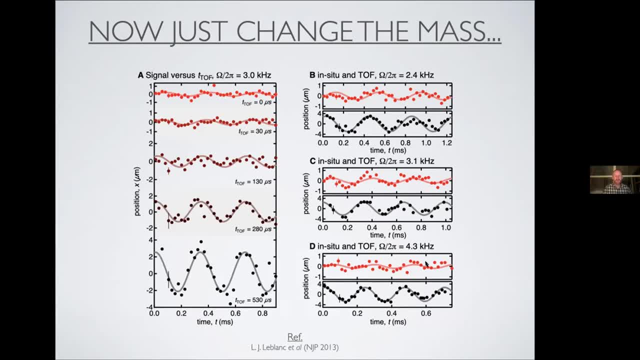 So this is really showing that we're observing the predicted Zitubo-Vegu by tuning different parameters in our rule book- our Hamiltonian- and observing that the changes are in line with what we're expecting to see. Now I'd like to conclude my description of Zitubo-Vegu. 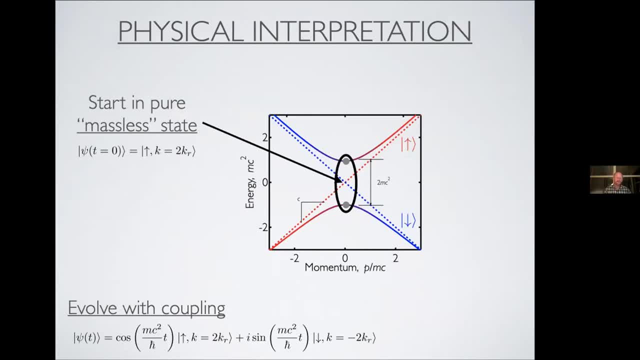 in terms of a more physical interpretation. So let me describe what the experiment went like. What we did is we started actually the particles in the red massless state And then suddenly we turned on the lasers that caused the direct dispersion to exist, and then followed with a subsequent absolution. 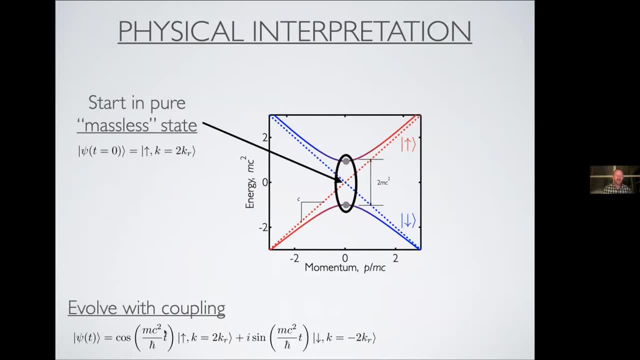 It turns out that the equation describing this motion is oscillatory, with sines and cosines in it, And the system was always in a superposition, a quantum superposition, of both the plus velocity and minus velocity states. Now, to an atomic physicist, this is incredibly familiar. 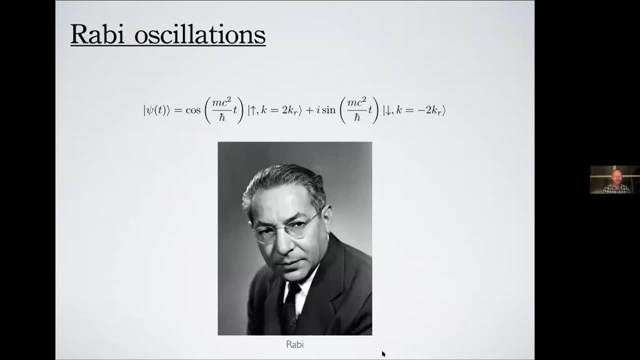 These are Rabi oscillations. So here's a prediction, a picture of JJ Rabi- Sorry II Rabi when, a sort of contemporary for when he developed both this idea and this tool. So what Zittabuggen really is is Rabi oscillations. 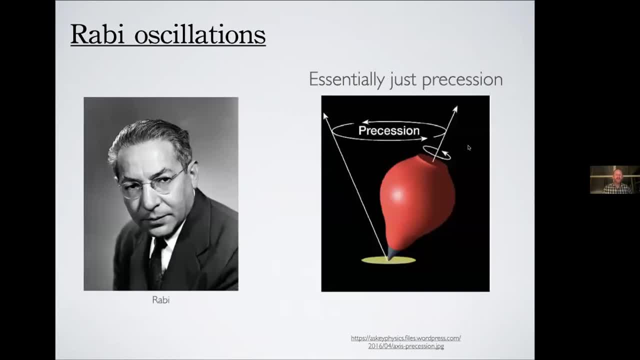 but maybe you don't know what Rabi oscillations are, but probably you do know what precession is. So if you've ever had a top and caused it to spin and tilt at an angle, you will see that the top precesses. 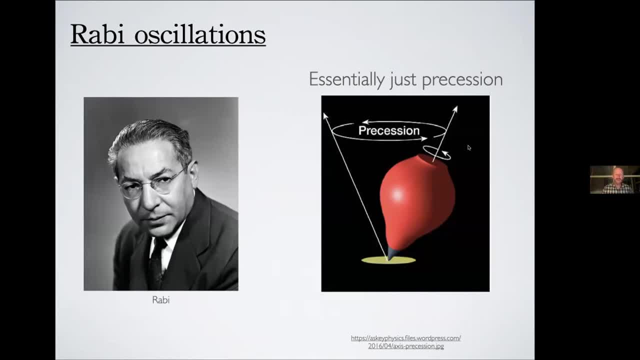 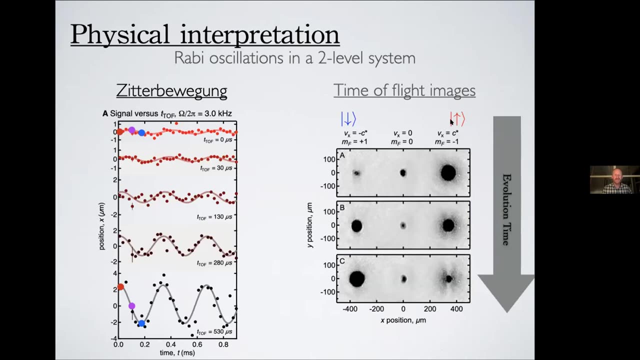 around the vertical direction. This precession is the classical physics analog to Rabi oscillations and therefore the classical physics analog to Zittabuggen. So we could directly confirm this as well by looking at the probability that the atoms resided in these two initial positive velocity. 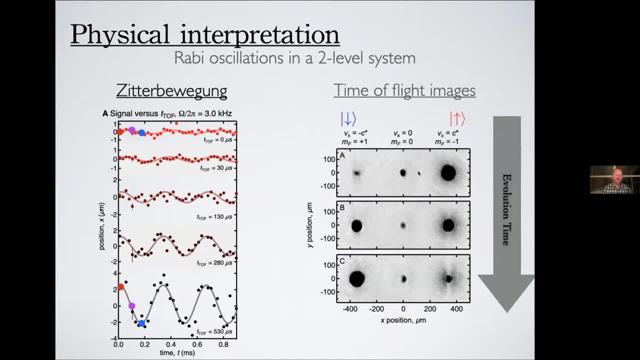 and negative velocity states and indeed observed the Rabi oscillation between population in those states. So the takeaway here is that Zittabuggen both is an iconic figure of quantum mechanics, but it's also an iconic figure of quantum mechanics from the early days of quantum mechanics. 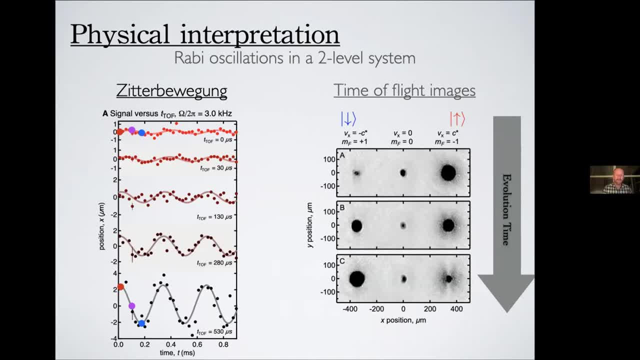 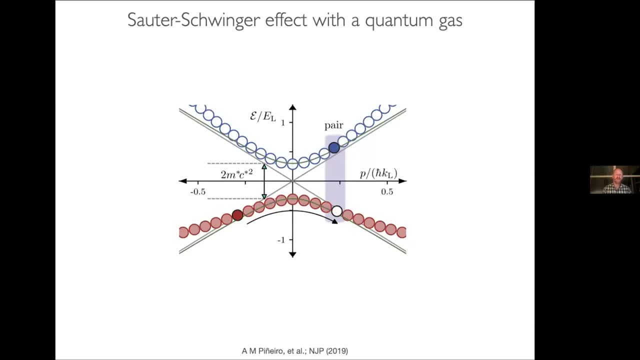 that rears its head under a different name in atomic physics and that we can directly measure in the laboratory using this rescaled system. The second piece of relativistic physics that I'd like to describe to you today is the Sauter-Swinger effect. 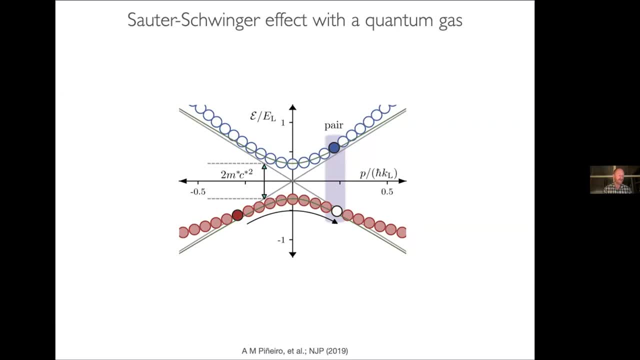 also realized with the quantum gas of Bose-Einstein condensate. So I'd like to take a little bit of time to describe the figure I've plotted here, because I haven't mentioned at all anti-quantum gas, I haven't mentioned at all anti-particles to you. 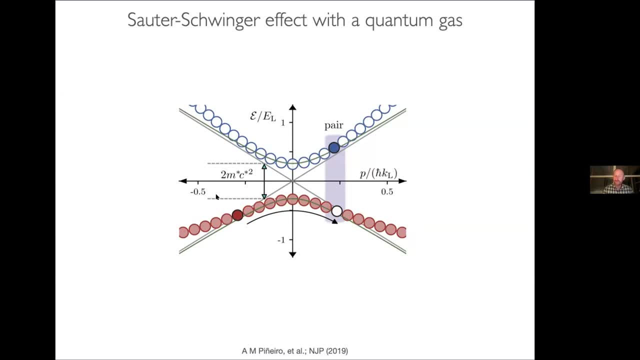 although I've implicitly showed them in graphs I've had before. So particles on the top curve here are in a very obvious way analogous to electron states. For example, this blue circle here would correspond to an electron, to momentum given by whatever's plotted here. 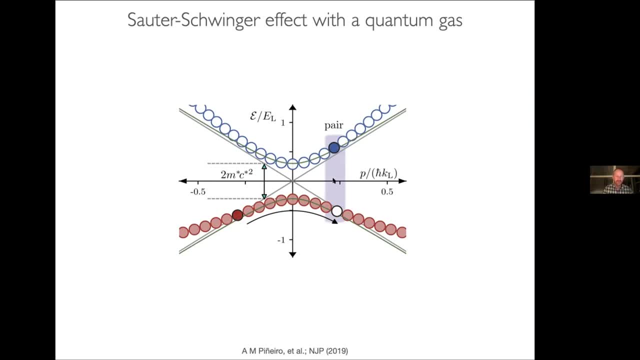 on the horizontal axis. So that's really simple. But the vacuum is a little bit more confusing to think about. What if there's no electrons and no positrons? Well, counterintuitively, that corresponds to occupation of every single negative energy state. 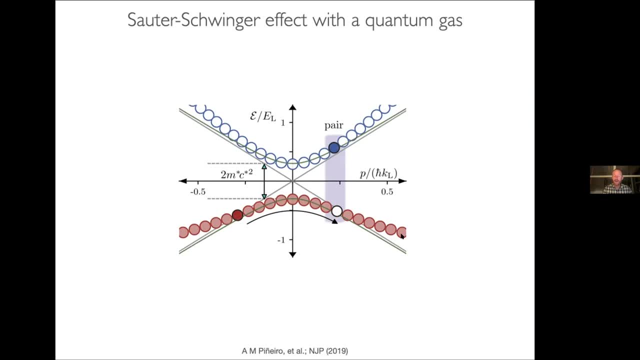 These would all be occupied, and that's your vacuum of nothing. And what a positron actually is is when you grab one of these field states and you empty it, For example moving it up there. This then corresponds to an electron up here. 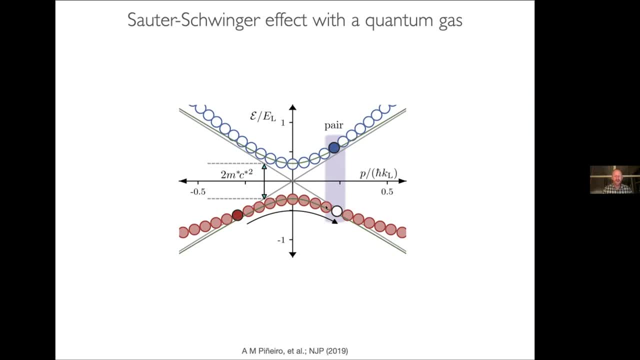 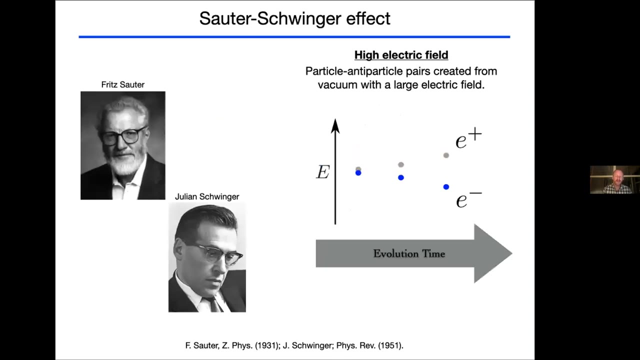 and a positron down there, And that effect is why the positron, for example, has a negative charge. If you think to condensed matter physics, this is therefore electrons in holes in semiconductor physics. Anyway, All right. so the Sauter-Swinger effect, 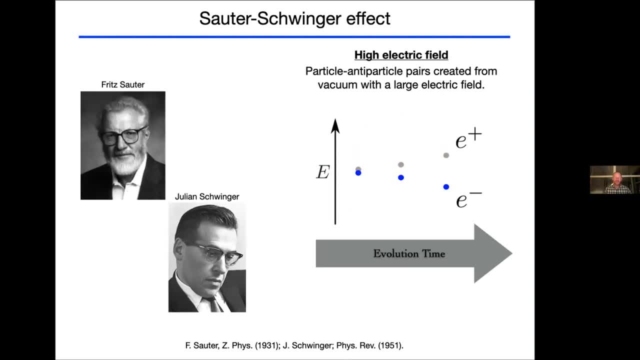 One way to think about this is that the universe consists of a sort of fluctuating quantum vacuum- And again this is somewhat accurate- And where electrons and positrons are constantly appearing and disappearing And what we do is apply a very, very large force or electric field. 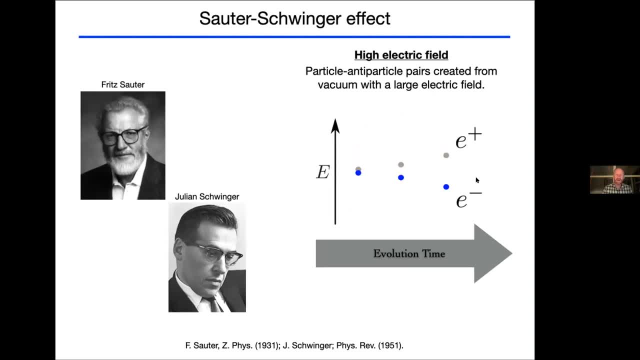 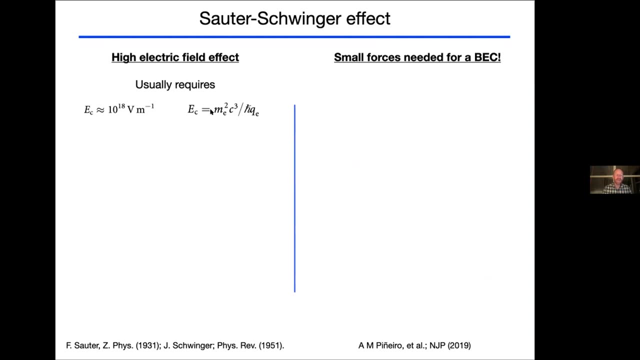 that pulls these particles apart before they've had a time to recombine and continues to accelerate them, thereby producing a positron-electron pair, giving real life to these otherwise virtual particles. As before, this is an extremely high field effect. The required electric field: 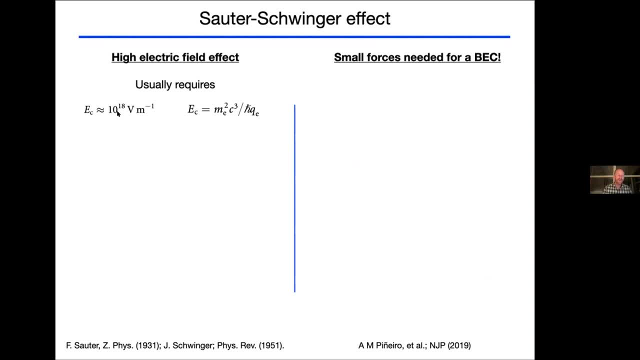 to see any appreciable amount of particle hole. production is 10 billion billion volts per meter. So the scale of volts per meter to simply have an arc, a zap, is only maybe a thousand or so, A couple thousand volts per meter in air. 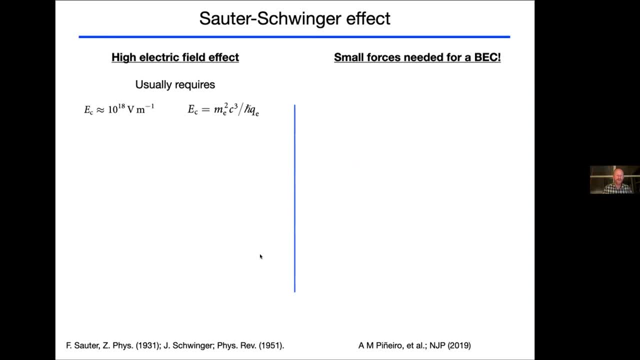 So imagine how much electric field is required to have the Sauter-Swinger effect. It's astronomical. So here, graphically, is another way to think about the effect. Imagine a Feynman diagram of this type where you come along. 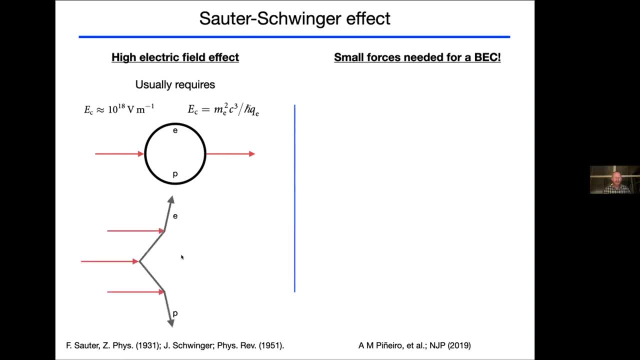 virtually produce an electron-positron pair, which of course ordinarily recombines. If instead a very, very large, constant electric field is present, as this loop forms, another photon comes along and kicks the electron. another photon comes along and kicks the proton. 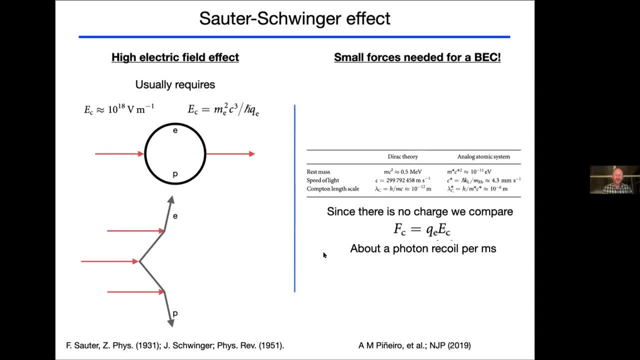 and so forth, thereby accelerating them. In the same way that we were able to transduce from very large to very small scales in the Zitterbegen experiment, we're also able to do so in this Sauter-Swinger experiment. 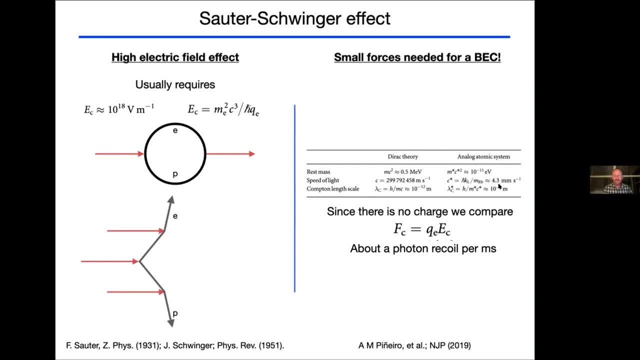 And here, for this particular case, are the scales that we're going to have. In particular, we're going to see what's going to be 4.3 millimeters per second And this sort of Compton wavelength scale, the scale over which you resolve. 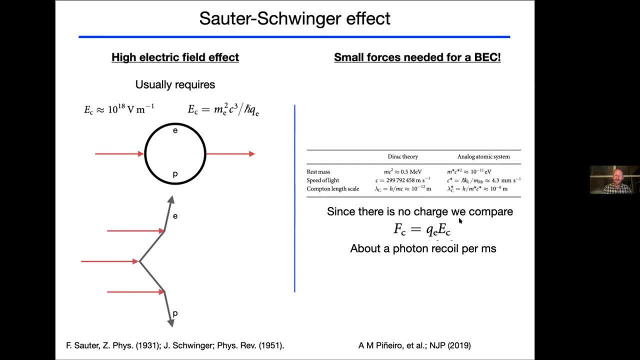 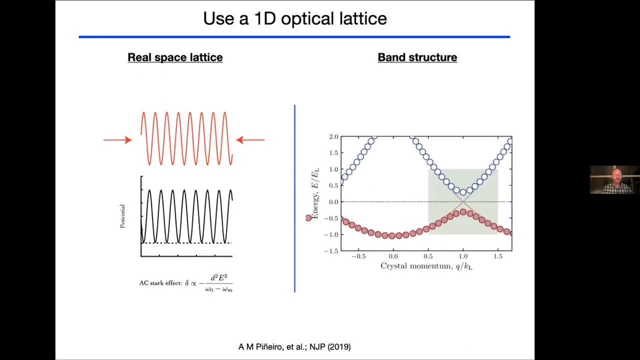 the position of the electron is going to be about a micrometer, similar to before, But now we're going to be thinking about a critical force rather than a critical electric field, because fundamentally, our particles are charge-neutral, So we always have to think about this. 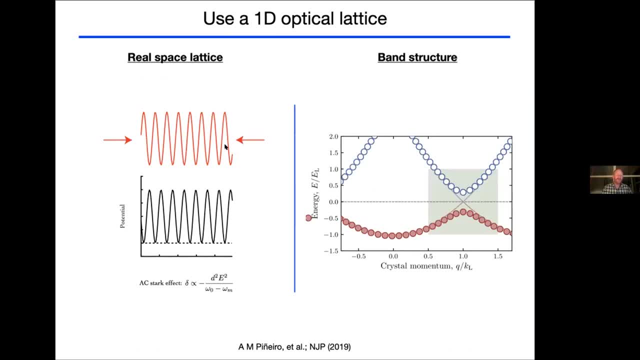 electrical charge times field product. So what's the relationship between the two? Well, she first made a standing wave of light that made this sinusoidal potential here, this energy landscape that the atoms resided in. This is the momentum relation I'm plotting here. 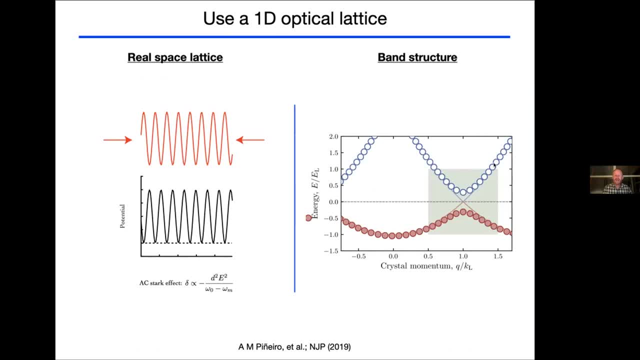 So this represents a band of energy states for what I'll call the ground band and first excited band. And, exactly as I described before, if you zoom into a small region of this where there is a crossing, you'll see that in that general vicinity. 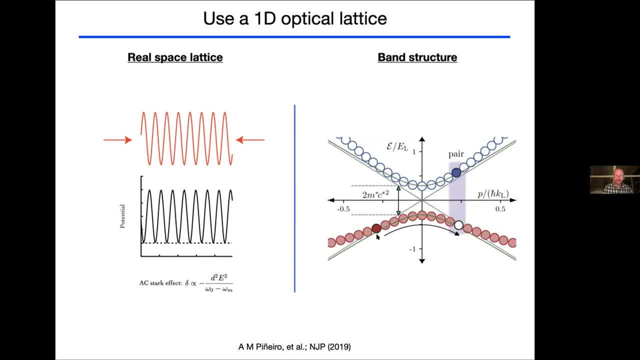 you'll see that there is a very large amount of energy that goes into the ground band. So what we're going to do is then apply a force and literally push on these atoms, causing them to accelerate. In this case, by accelerate, I predominantly mean change their momentum. 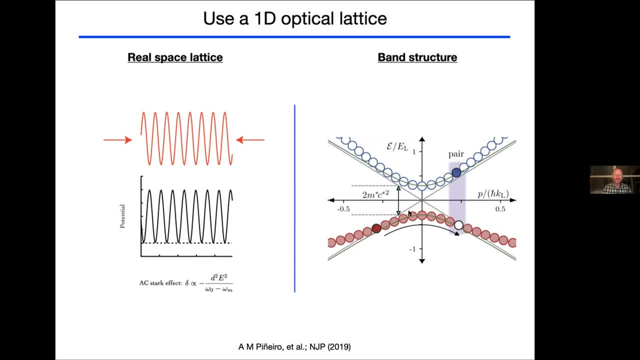 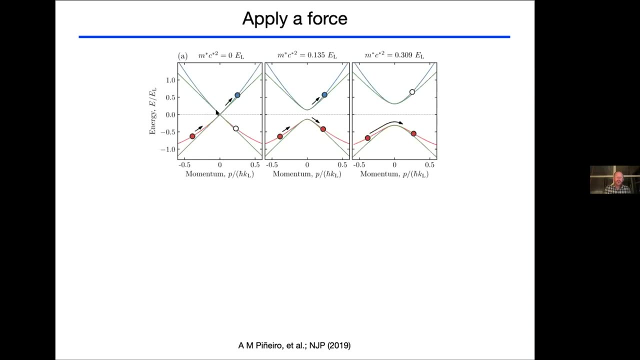 which, as a result, will have some change in their velocity. But remember, velocity is the angular slope of this curve, not really the momentum. And then we're going to see if, in this case, we're going to be able to change the momentum. 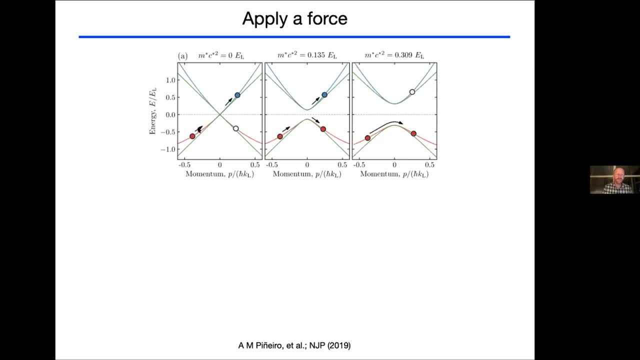 So here is sort of a picture. If there is no gap there at all, these curves continuously connect. This is the case of us doing nothing. And, no surprise, the particle traverses through this point ends up in the upper band or upper branch. 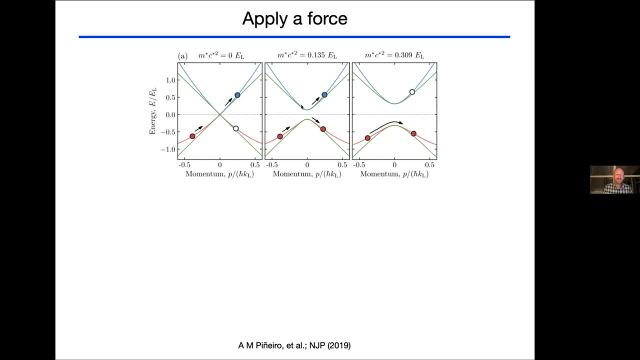 the electron branch, leaving behind a vacancy in the bottom branch. the initial state partially goes through, creating an electron partially, but leaving behind some of a filled state behind only creating part of a positron. This is a quantum superposition between the electron-positron pair. 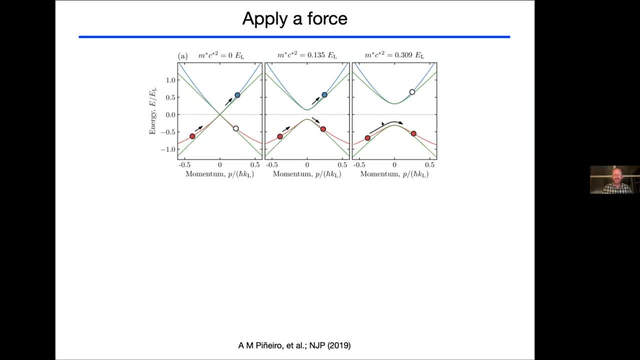 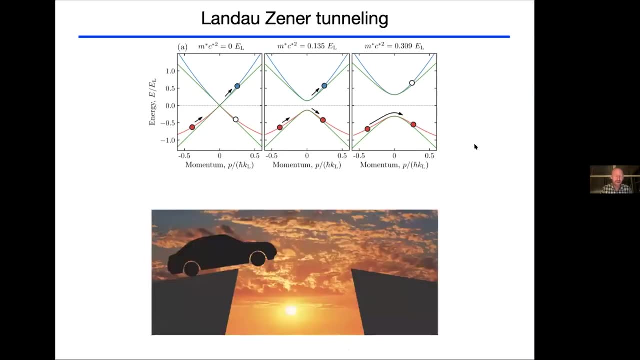 And finally, with even larger gap, that is, larger mass. when you push on it with the same degree of hardness, the state just follows through. What's going on there? Well, it's actually not particularly different than the ill-advised daredevil stunt. 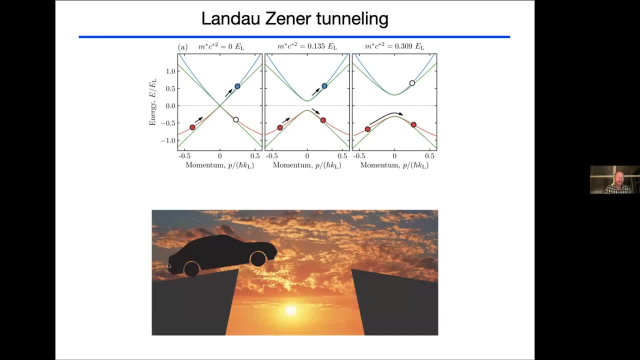 I'm plotting here. If this car is able to go sufficiently fast, it'll manage to leap over this barrier, in the same way that this state traversed rapidly through that crossing. But if this driver is driving an underpowered vehicle or for some reason doesn't go fast enough, 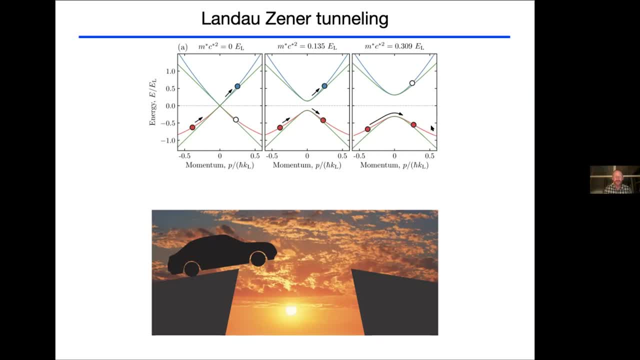 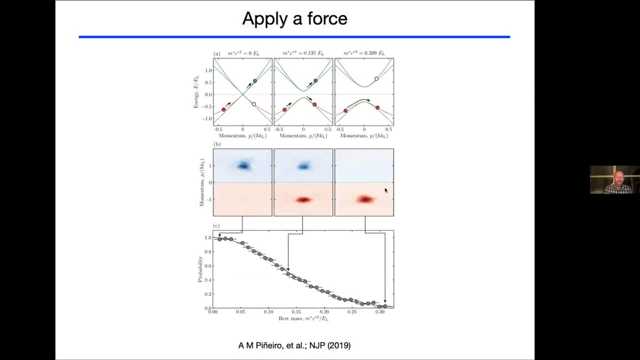 they will fall right into the abyss and therefore stay on this lower energy branch, not forming an excited state particle. So we perform the experiment, and here is what experimental data actually looks like. This is the case here. This is the initial state traverse. 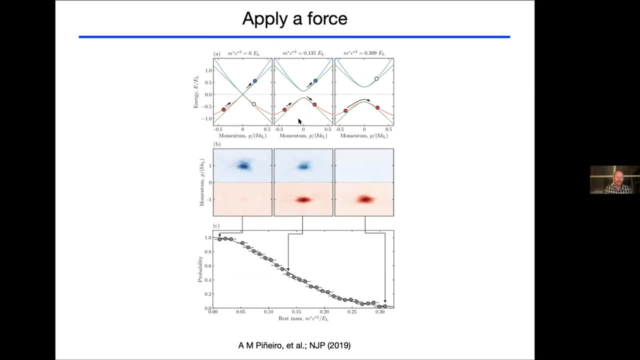 fully through the gap producing electron states. This is the case where you produced part of an electron and part of a positron, giving occupation in both states, And finally, this is the case where everything was left behind in the lowest band, thereby creating no electrons nor positrons. 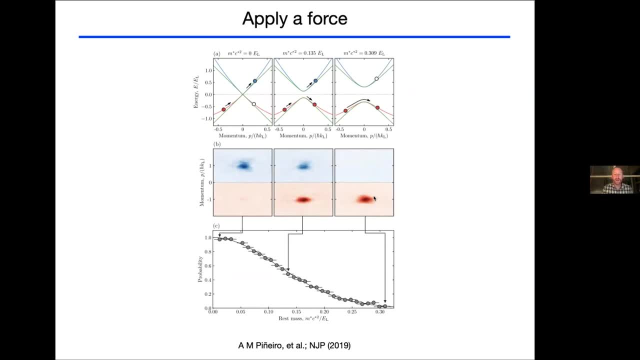 And there's one subtlety about this data that I'll point out on the very next slide, But in any case this was plotting here the probability that electrons were created. So for very small masses, 100% probability. And as one increases the mass, 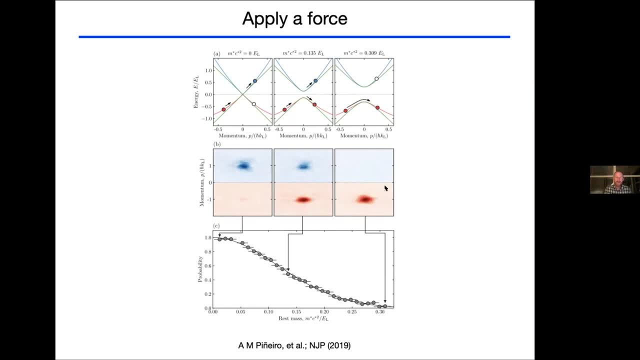 the probability drops to zero. This too has a name in both condensed matter and atomic physics. It's called Landau-Zehner tunneling And the curve underneath. this is exactly the Landau-Zehner equation, except in these rescaled units. 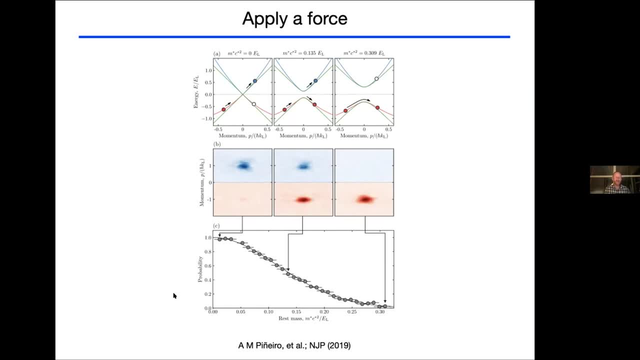 So exactly as we saw before that the effect of Zitterbewegung had an analogous interpretation in atomic physics, so too does pair production. Pair production is really the same as Landau-Zehner tunneling. So we see in physics the same ideas. 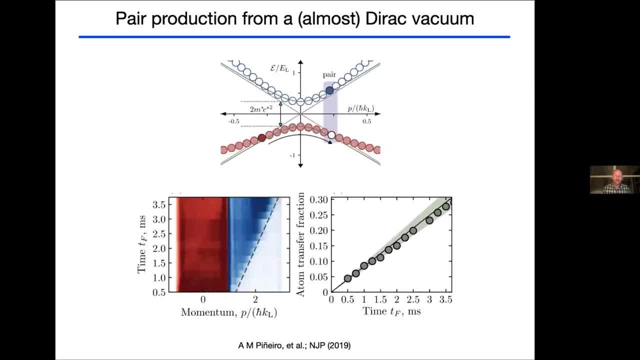 come back at us again and again. So the last thing I'd like to show is then pair production from an almost direct vacuum. So what I showed you before. in fact, we prepared just one quantum state, That was a Bose-Einstein constant state. 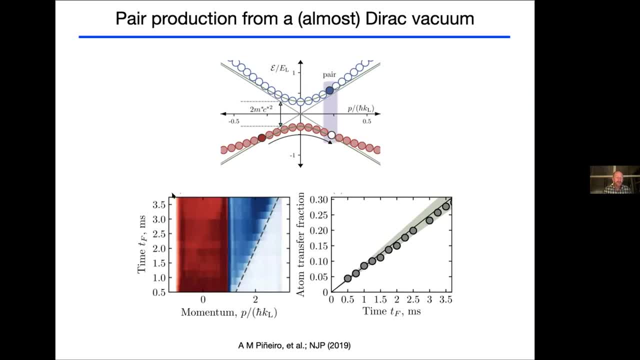 where all the atoms were in the same state. And then in physics, the next thing we did was fill every state in the lowest band, just like the Dirac vacuum has initially every state filled. That corresponds to this red region down here. 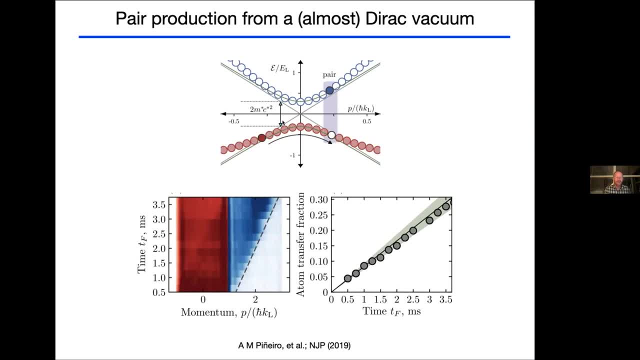 Then, just like before, we pushed on the system, causing the momentum to change and the atom, these states, to sweep through this crossing And what's being plotted here as a function of increasing time in the higher band, whose momentum is linearly increasing. 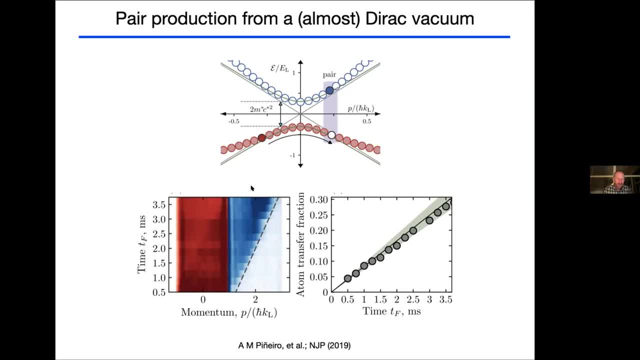 with time, just as you'd expect from this force. It's a little harder to see, but this sort of slanted line. here is the analogous set of whole states or positron-like states that are being produced as well. And finally, here is the transfer probability. 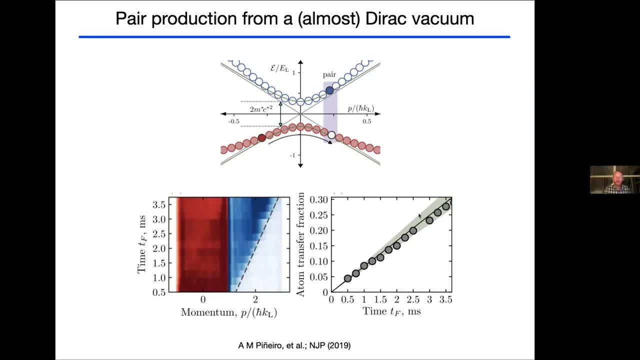 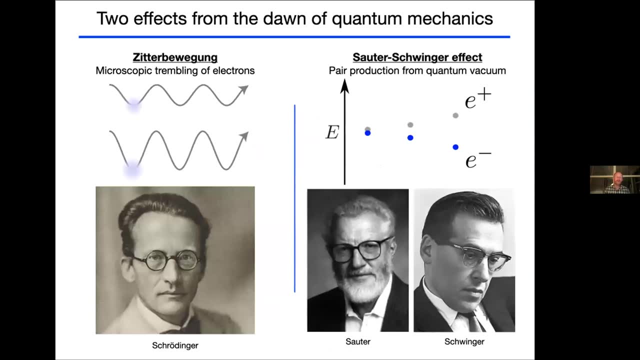 or transfer fraction as the function of time, fully in agreement with the Sauter-Schwinger or Landau-Zehner prediction. So with that I'd like to leave you. I've shown you two effects from the dawn of quantum mechanics. 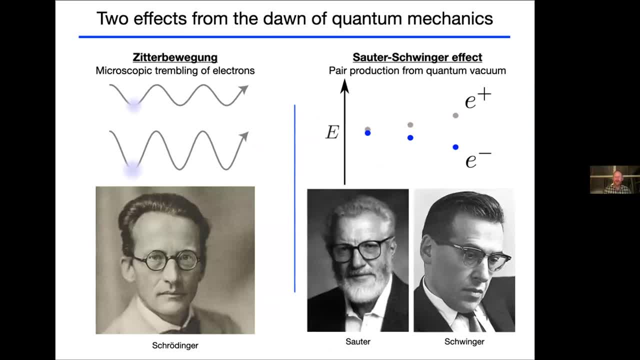 Zetupov-Weggen and the Sauter-Schwinger effect and shown that by realizing exactly the same Hamiltonian, that is, the same rule book in our cold atomic system, we're able to realize these iconic effects and directly observe them. 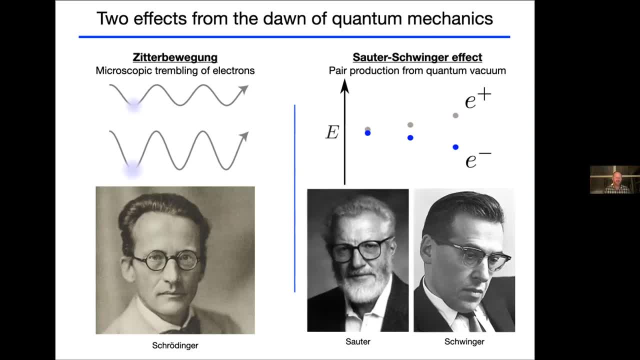 in a terrestrial laboratory on pretty much human time scales and frequency scales. So thank you very much, Thank you. Thank you, Ian. I'm looking for the button for hand claps, but I'm not very good at finding it very easily. 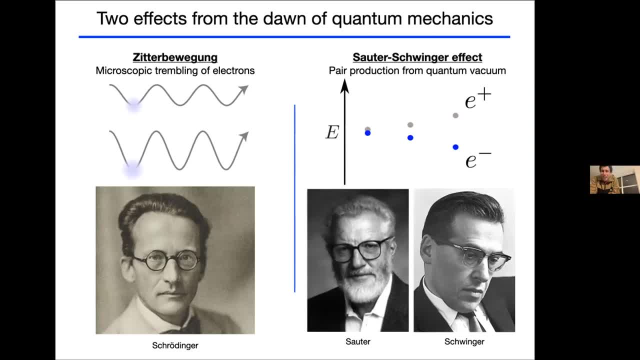 so I'll just clap my hands And I hope you all join me. So we have time for questions. If you'd like to ask a question, just press the raise hand button and I'll try to call on you to ask your questions. 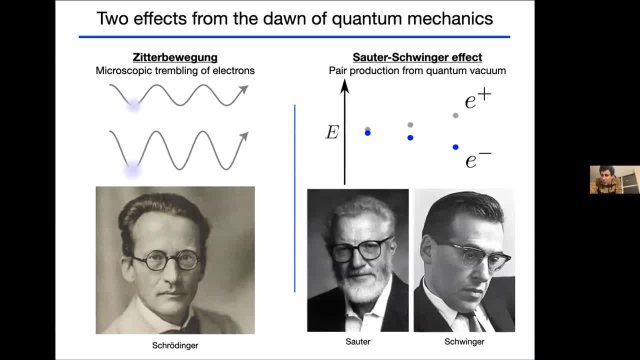 Yeah, I see a question from Ehsan Khatami. Go ahead, Ehsan. Was that a hand raised Something's in the chat? Oh, okay, My iPad was a little malfunctioning. Um Okay, Any questions? 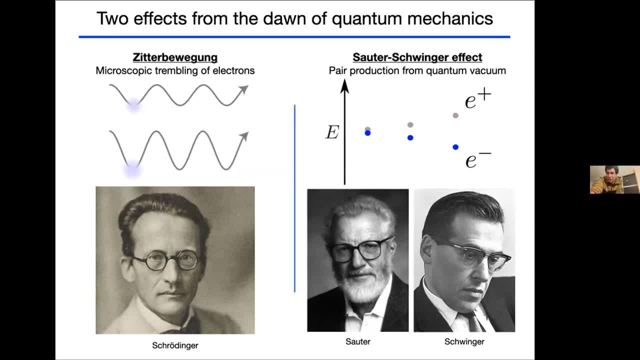 I see a question from Connor Hoffman. Go for it, Connor. Yes, Hi, So thank you. That was a fantastic lecture. I will say a little bit over my head, but still a lot of fun to listen to. How do you measure the temperature? 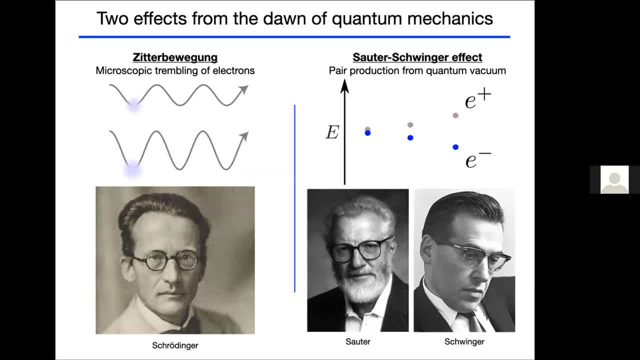 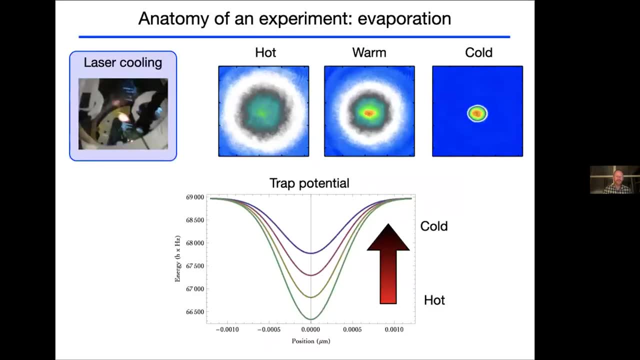 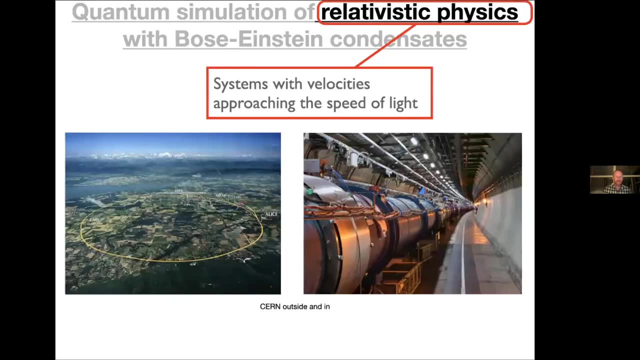 when you get down that small. That's a great question. Let me hit the back button to get some graphics to support that. Okay, I will use. I think I had another one on the temperature graph, Did I not? Oh no, 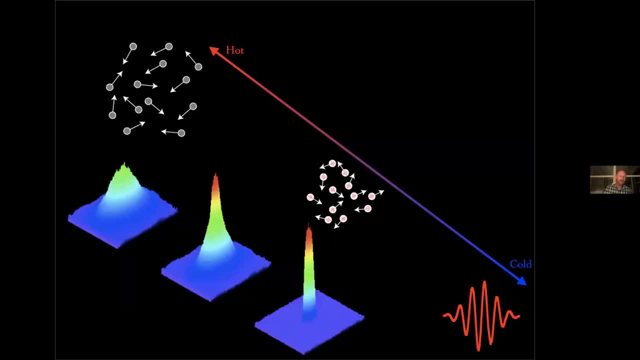 All the animations are going to come back, I will use this one. So what we do to measure temperature most of the time is to have a theoretical description of what this set of states is going to look like. So what I'm plotting on this graph: 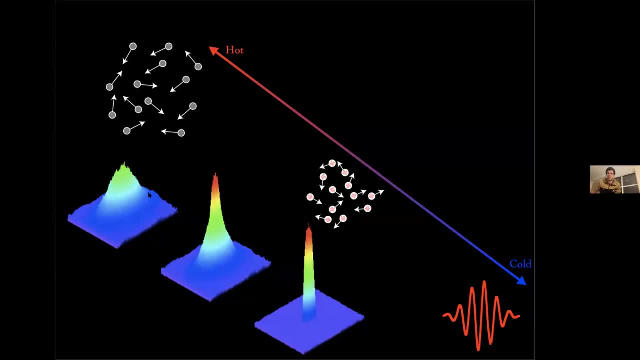 is how likely it is to find a state, or how many atoms have a certain velocity. So that's what this graph is meaning. So, because of the relationship between velocity and temperature, for a simple image like this, we can directly read off: 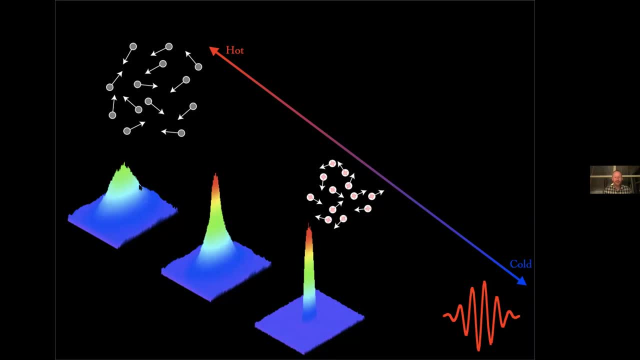 the temperature basically from the width of this peak. So as it gets colder, the peak gets narrower, which you can sort of see happening here. So, to give a little bit more detail, what we actually do is we have the atoms confined in a trap. 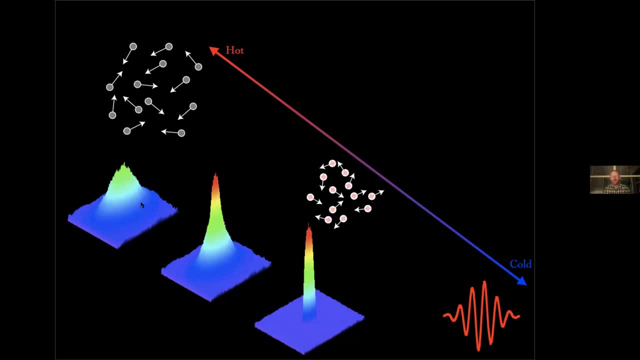 and if you look at them then you'd see it would look like what I showed you in the experiment where you'd see where the atoms were. So actually what we do is we turn off that trap suddenly and a lot of the atoms should just fly. 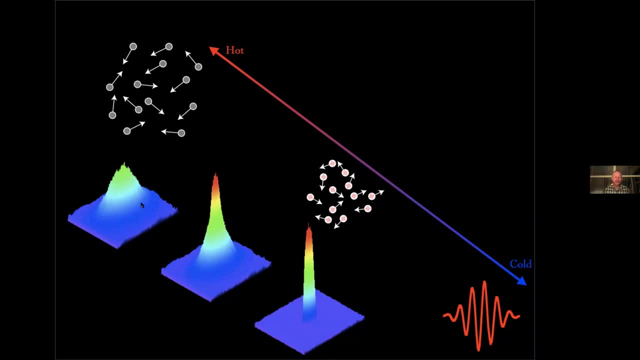 or ballistically expand is the more fancy way of saying it. and then, after that flight period, you see a picture like this that gives you where they ended, which, of course, is telling you how fast they were going. So then, by plotting the width of this, we get the temperature. 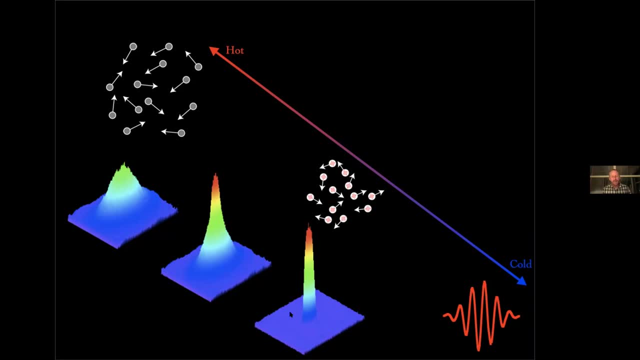 So most of the time this is the most direct way to get temperature. It breaks down with data, like the very right hand plot here, where this is a Bose Einstein condensate and the width of this doesn't have anything to do with the temperature. 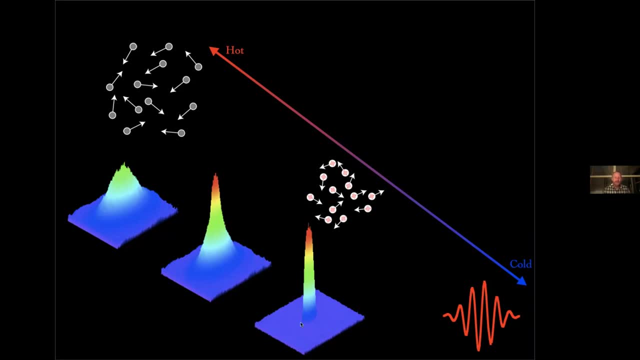 The width of this has to do, in this case, with the interactions between the particles. So for very, very cold systems, you need different ways to measure the temperature and, to be honest, my group has hardly ever used these techniques. I see something in the chat. 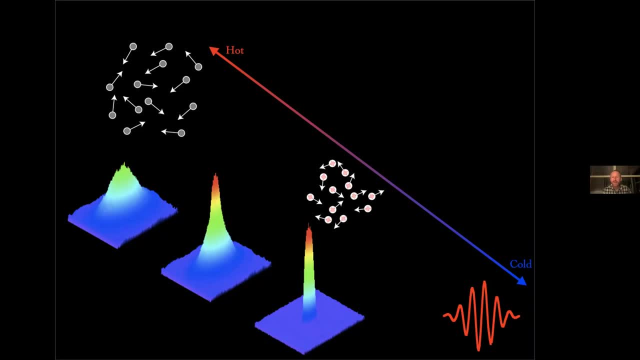 So Ken Rosenbaum asks: thank you for the talk. What are the practical benefits that your research may help enable? All right, So, Ken. so the talk I gave today is very much a fundamental physics kind of talk, So we're aiming at understanding. 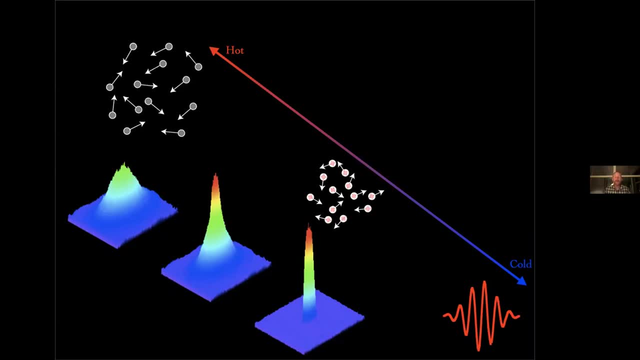 different aspects of how our physical description of the universe works. So we're going to talk a little bit about how the universe works. So this particular piece of physics, I think, has very limited applications because really we're not quantum simulating anything that itself has applications. 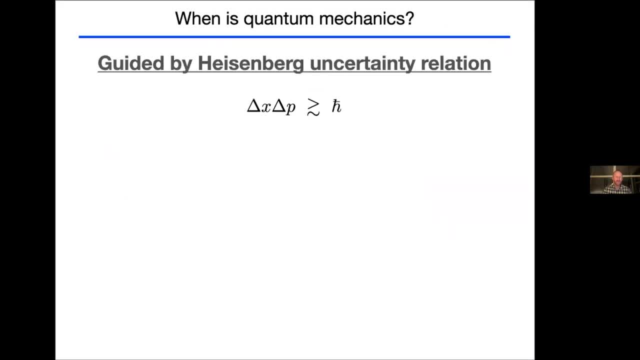 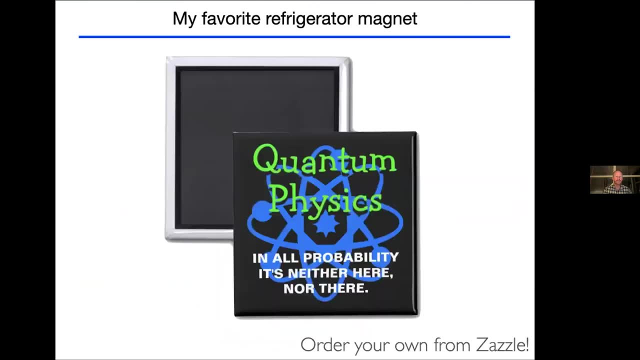 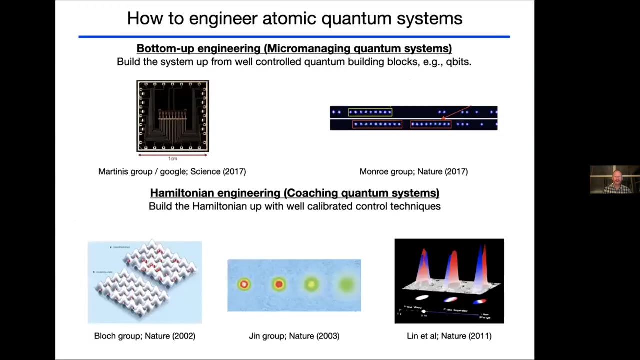 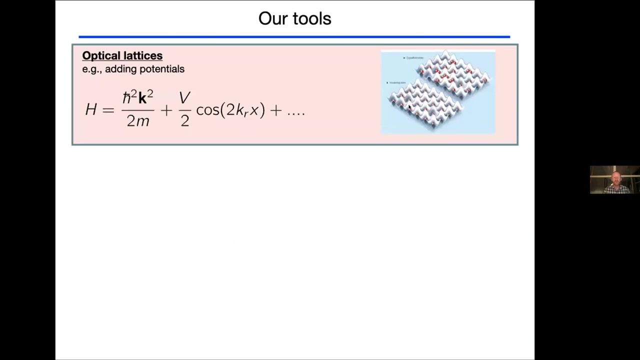 In the bigger framework of quantum simulation, though let me go to a different slide that will maybe elucidate this. I'll use this one here. So for pictures like this, this is also a quantum simulation. The atoms are sitting in this sort of egg crate-like landscape. 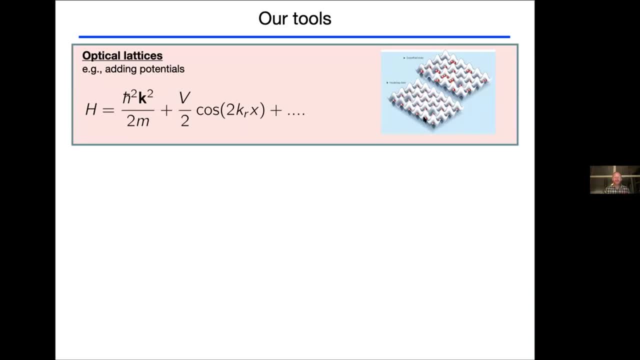 where they can move between In real life. a lot of particles that are fermions move in egg crate-like potentials as well. These are called electrons moving in lattices, And what lattice? Well, crystal. So virtually every element. for example, 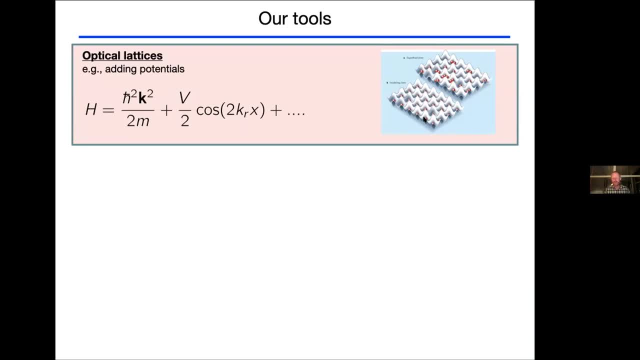 active element of your computer is a semiconductor that's typically crystalline and occasionally amorphous, that electrons are moving about in. These are well understood, these sort of room temperature semiconductors. But really important questions arise when you cool the system down. 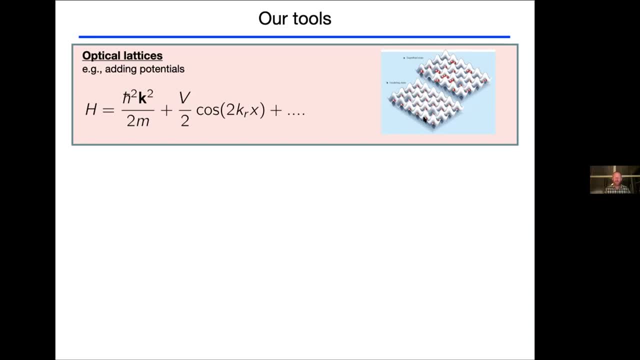 So at very low electron temperatures- this might be single kelvin or milli kelvin- a myriad of effects appear, many of which cannot be explained theoretically. One of these effects that probably has the highest technological impact is high temperature superconductivity. 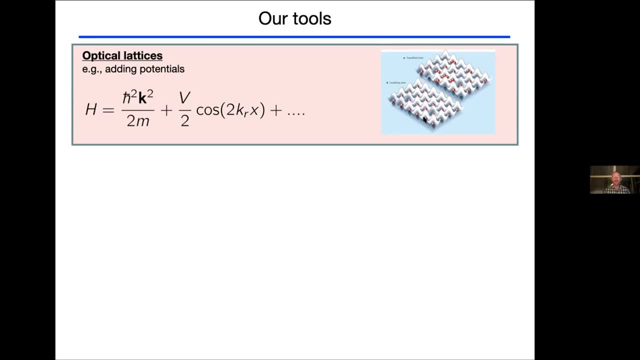 where high temperature can exist, to temperatures maybe as high as 150 kelvin or, in an absolute scale, about half of room temperature, And the sad state of affairs is that no one actually understands for certain how high temperature superconductivity works. There are ideas, there's proposals. 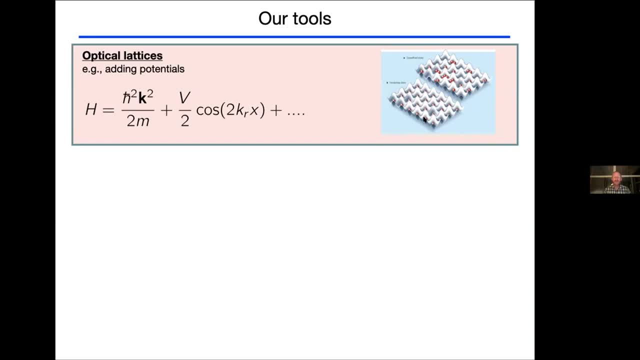 and there are people who are strongly opinionated that their idea is correct But truthfully, we as a community of physicists don't know. So we have to look at these systems, these quantum analog systems, and ask questions of them to understand. 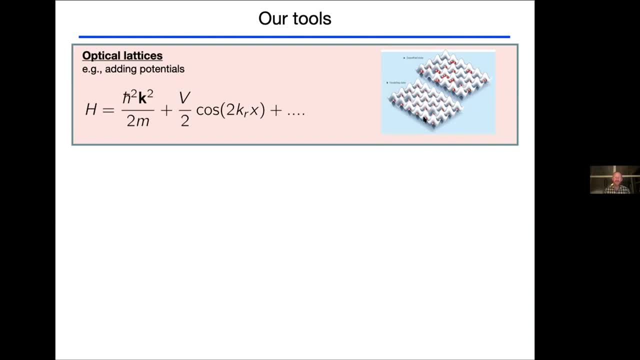 whether different descriptions of high temperature superconductivity are correct, And I think the reason this is important for the technological standpoint is that until you have a description of how something works, it's very difficult to switch from discovery to the engineering design phase where you can semi-deterministically 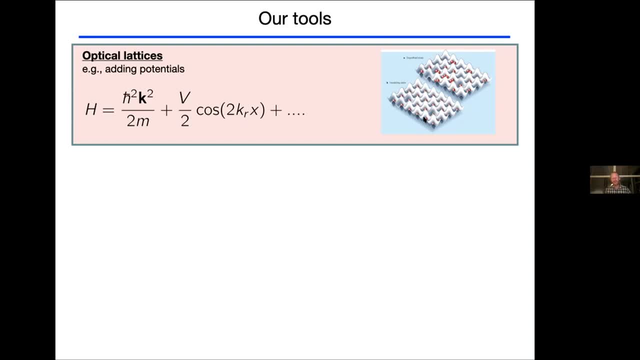 modify a system, go through an engineering design cycle and iterate to improve it. So high temperature superconductivity- a detailed understanding of the mechanism- is something that would transition that effect from an awesome physics effect to something of large-scale technological impact. I wanted to add to that. 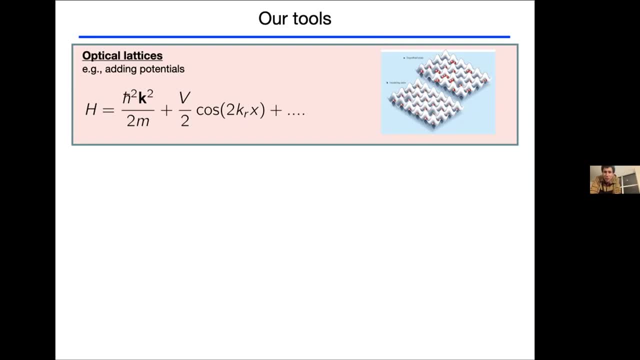 that the system of atomic condensates has been used recently for precision detection of gravitational fields, And I think it's important to note that some people are talking about using atomic condensates for medical sensing because it's so sensitive to any electric field or any gravitational field. 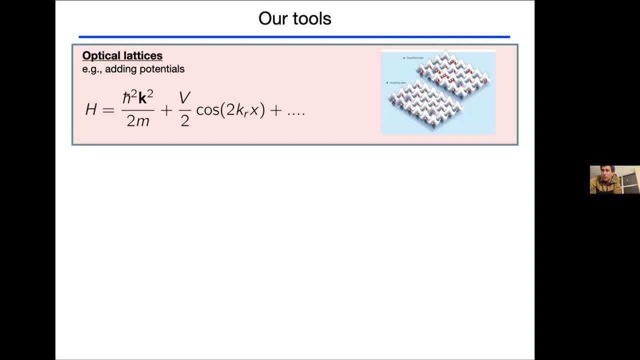 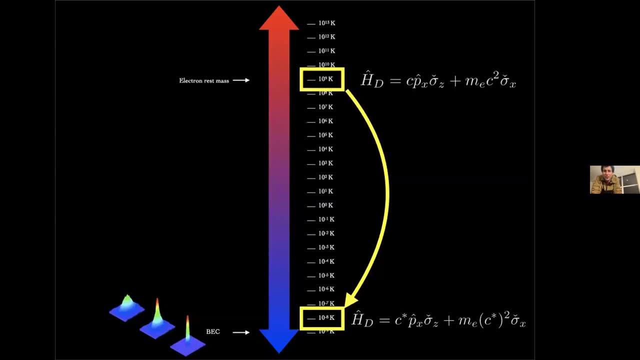 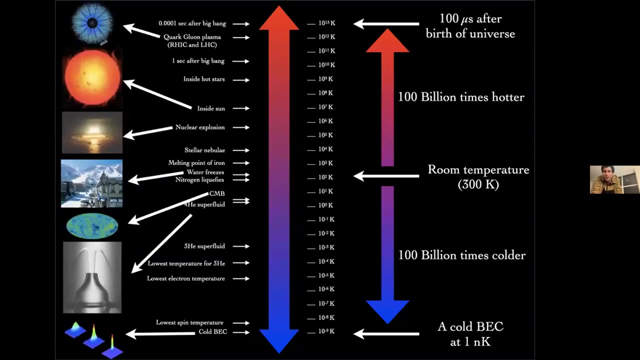 in the vicinity. There's another question from JJ regarding the temperature measurement. If you never measured the low condensate temperature in your group, how do you know at what temperature you are to correlate with the scale that was showed? Yeah, so the answer to that is that. 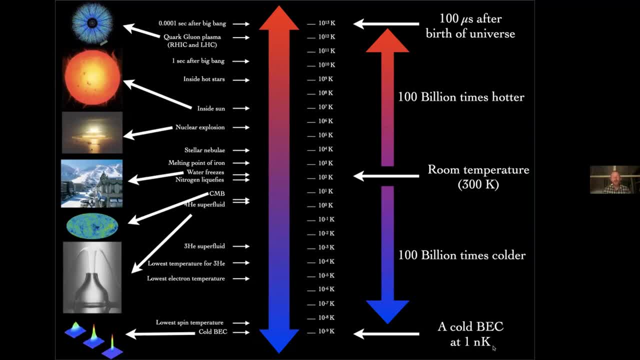 this extremely low temperature of one nanokelvin is not a temperature that my group has measured. In fact, the lowest BEC temperature that I think has been seen is Wolfgang Ketterle's group of about half a nanokelvin, so a couple hundreds of picokelvins. 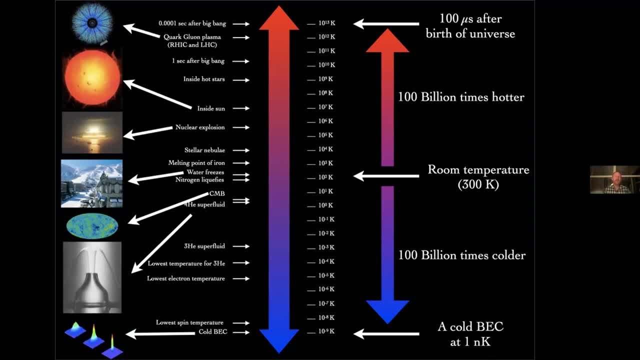 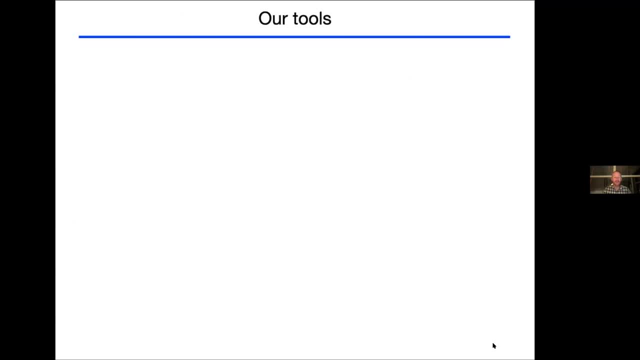 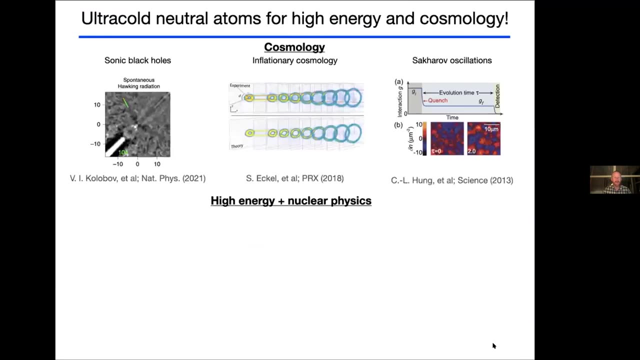 The coldest temperatures. I think that I would claim I've definitely measured in my group, and that was using exactly the time-of-flight methodology I showed before, And I'm trying to find the picture that had that on it. Yeah, so the scale of the temperature. 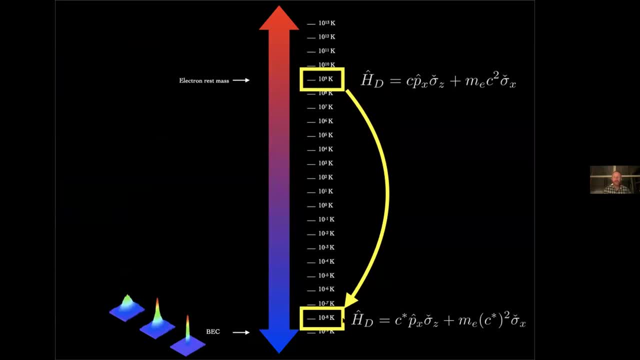 for the experiments I described today were about 10 nanokelvin, which is a place where there's enough of the non-Bose condensed atoms hanging around that you can get a reasonably reliable measure of temperature. Let me just interject. Ian, you were done with your answer, right? 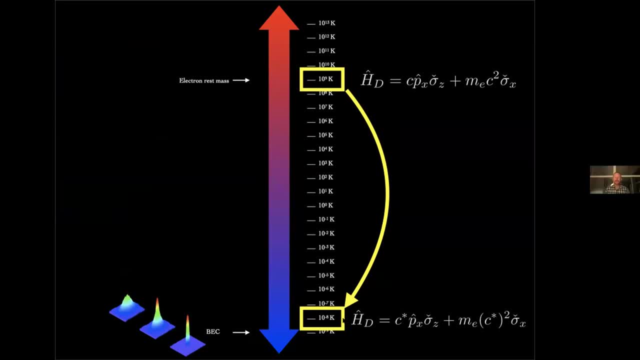 Yes, Let me just interject. Some people are going to start leaving, so I want to thank you all for attending. Stay on if you want to participate in the debate It was a pleasure to host on behalf of the Aspen Center for Physics. 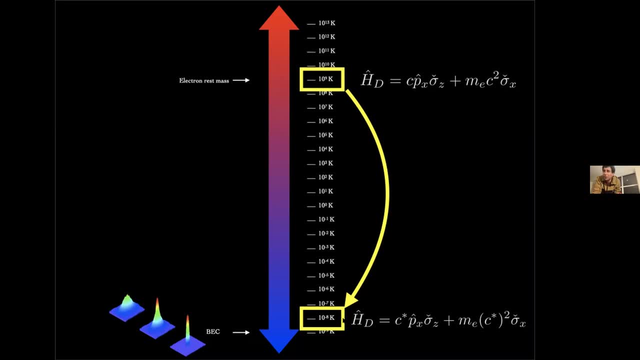 this public talk And if you would like to not stick around for the discussion, feel free to leave at any point. But again, thank you for attending. We hope to see you in the coming weeks and talks, But in the meantime let's go back to the question and the discussion. 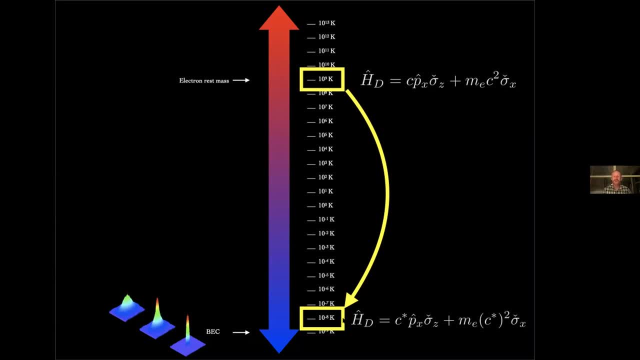 Yeah, so I see a question from Judah, No, sorry, from Richard. So Richard Fletcher asks: did you encounter entanglement? And if that's the right question, So nothing I described today would really be categorized as being particularly entangled. 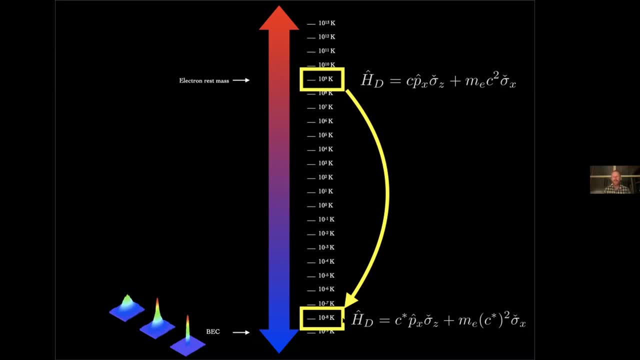 But, more importantly, there's no experiment we did that would have demonstrated entanglement. So just for the audience: usually when someone says entanglement, what they're saying is that there's a spatially non-local correlation, quantum correlation between particles. 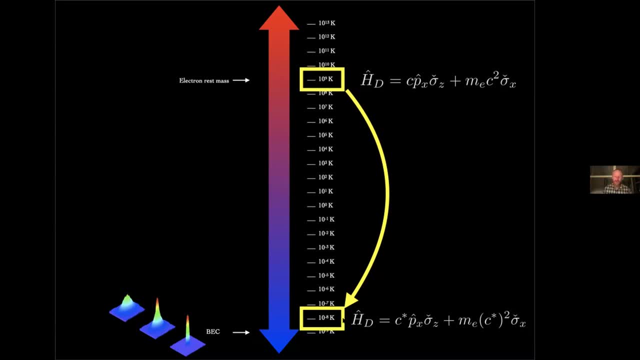 at one position and particles at another position. So I'm going to take that meaning of entanglement and say that the system we studied was practically not entangled. There have been other experiments that I've done over the years, For example looking at the superfluid-to-mod. 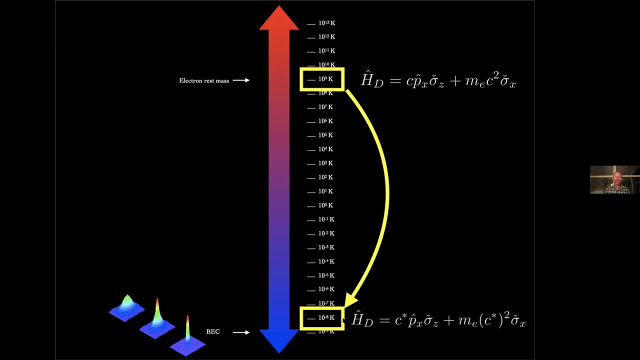 position that has a quantum critical point And at that quantum critical point that system has a modest amount of entanglement. It's not a super entangled system but it has a fair degree of entanglement. But again, we didn't do an experiment to measure that entanglement. 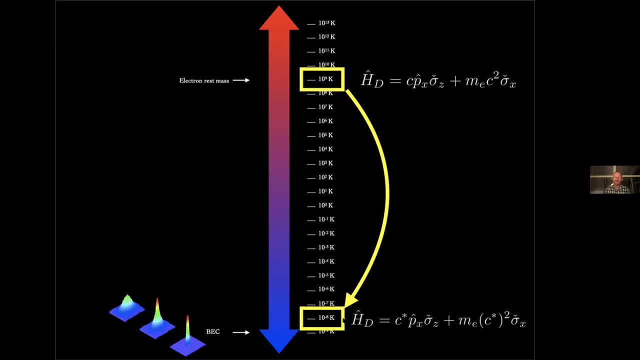 So when I say that it has some entanglement, I'm saying that our theoretical description of it predicts that it has some entanglement. Looking if there are any other questions, I see Connor's hand is still up, but I suspect that's because of the previous question, I should do have another. if you don't mind, Go for it. So you said, maybe I misinterpreted you, but you said that helium-3 kind of reached like a threshold that it couldn't get any colder. 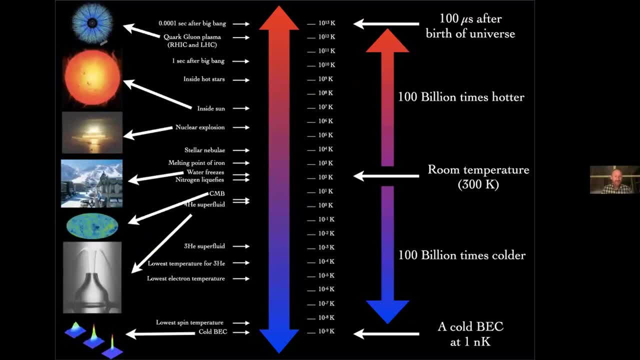 Is that right? Why couldn't it get any colder? Great. So these are actually technological questions. So the question that we So asking ourselves is: how is it that the things on this list are being cooled So starting at the lowest spin temperature? 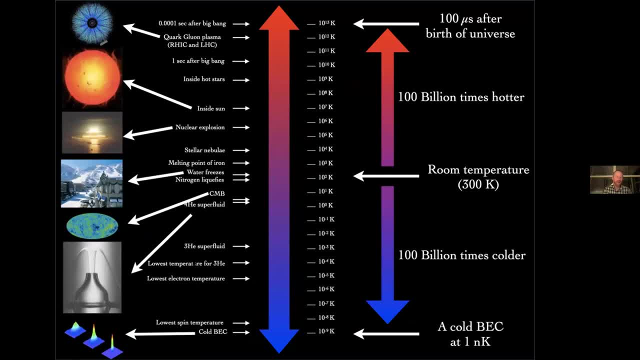 lowest electron temperature, lowest for liquid helium-3, those are all large chunks of stuff. These are pieces of metals or pieces of semiconductors or quantum fluids, like milliliters of quantum fluids that have been cooled to very low temperature. 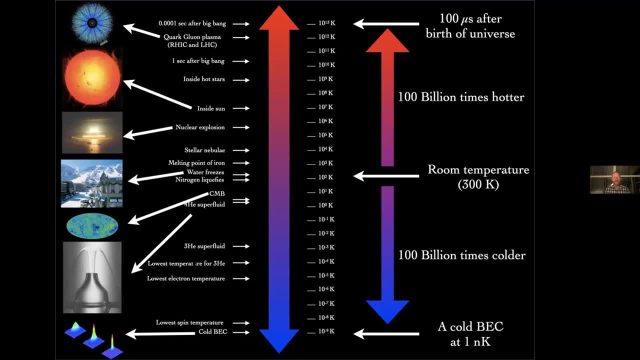 So each of these require basically more sophisticated technology to cool them. So I think in all the cases the mechanism of cooling is what's called adiabatic nuclear demagnetization for these very low temperatures, And the idea behind that is a little. 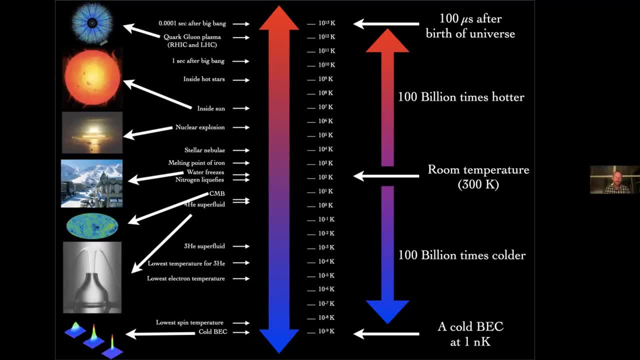 It's actually really cool. So what you do is you get a system. It could be a chunk of copper. Copper works pretty well, So you get a chunk of copper and the copper atoms have a pretty large magnetic moment And in the magnetic field the spin of that system splits a lot of energy. So there's a big energy associated with the spinning atoms in the magnetic field And what you do is you cool that as low as you can by some other mechanism. An example would be a different kind of refrigerator. 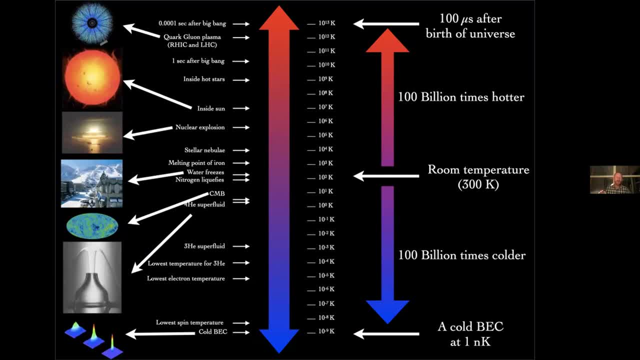 called a dilution refrigerator that can cool them, maybe to a couple of millikelvin, which is pretty cold. And the trick of this, the brilliance of this technique, is if you get, almost all of the spins is given to you by the probability that you have a small number of spins. 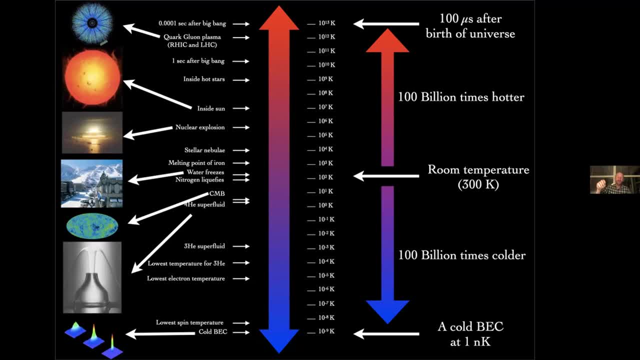 in the higher energy state And as you decrease the magnetic field, so you decouple the system from the refrigerator. It's just sitting there not touching anything, And you decrease the magnetic field, these energy levels get closer together and the temperature drops in proportion. 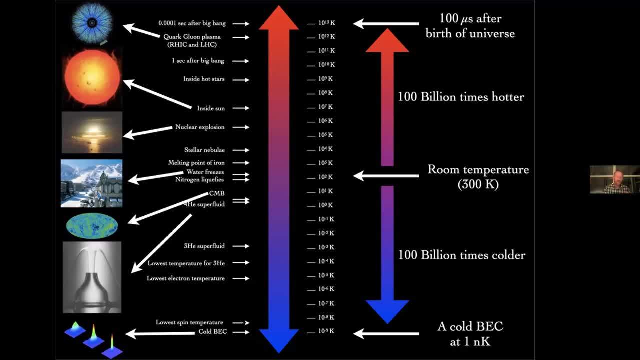 And that's why this low spin temperature has been realized. So for these other things- lowest electron temperature and lowest liquid helium temperature- you're getting such a demagnetization system and putting the other system in contact with it. So there is a threshold. 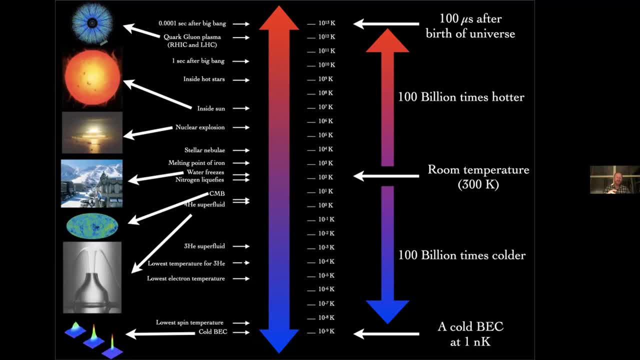 and the threshold is called the Kapitsa boundary resistance. And that's when the vibrations in the spin system that tell you about the temperature become poorly coupled to the vibrations in the lattice, that make the lattice have a temperature, and become poorly coupled to the quantum fluid. 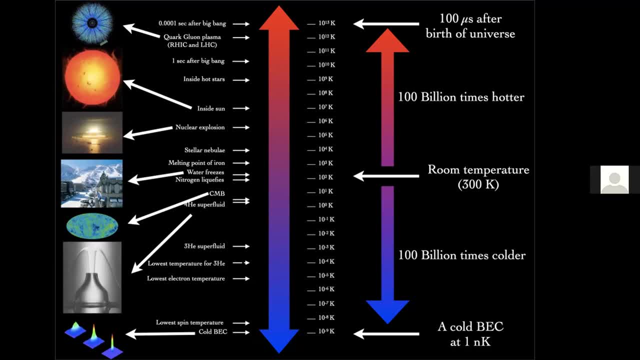 So it just kind of reaches a point where maybe not chaos, but it's like you can't quite control it enough anymore and you don't want any colder. Yeah, I mean, I would describe it as more sort of a decoupling, where the system you're trying to cool 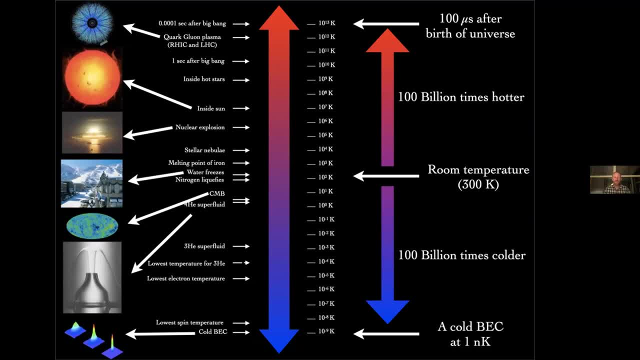 just is in so bad thermal contact with the system that's trying to cool it that it can't cool anymore. Okay, thank you. So the more general question in the chat. can you explain why matter cannot obtain the speed of light From Richard Fletcher? 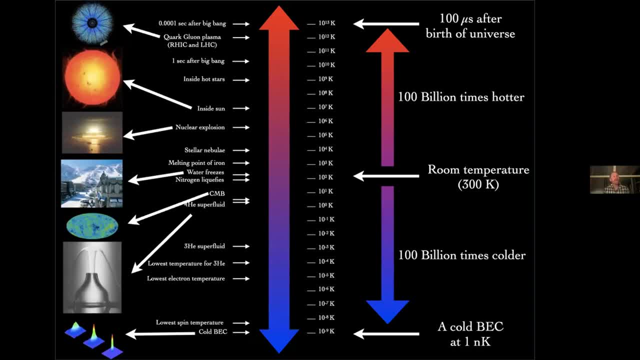 Can I explain that in a simple-minded way? So I want to say something about Lorentz invariance, and I think that that's not going to work right, So the I'll say it that way first. So we, as physicists, believe. the universe obeys a symmetry called the Lorentz symmetry. You can interpret that symmetry as meaning that if you care to, you can go into the frame that, no matter how fast you made something move any fraction of the speed of light, you could, if you want. 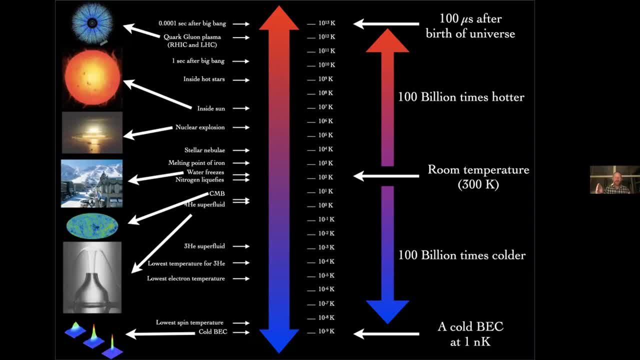 interpret the system as being at rest, with the rest of the universe moving in the opposite direction, And even you can think about this in terms of bowling balls sitting in cars- that's called the Galilean invariance- And at ultra-high speeds. 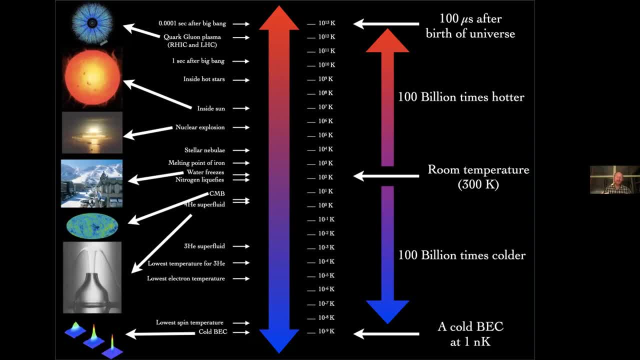 you think about the Lorentz invariance. The hand-waving description I would give on this is that if you keep pushing on a particle causing it to accelerate, you're asking for something sort of discontinuous to happen from going from less than the speed of light. 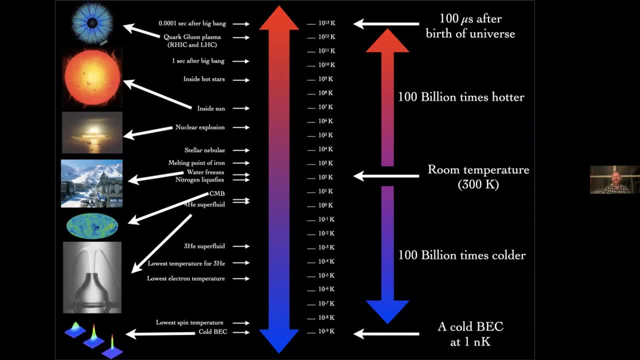 to the speed of light. So unless there are particles that can exceed the speed of light, something sort of strange has happened at that one moment where you went from not going to the speed of light to going exactly the speed of light. I realize that's not a really helpful example. 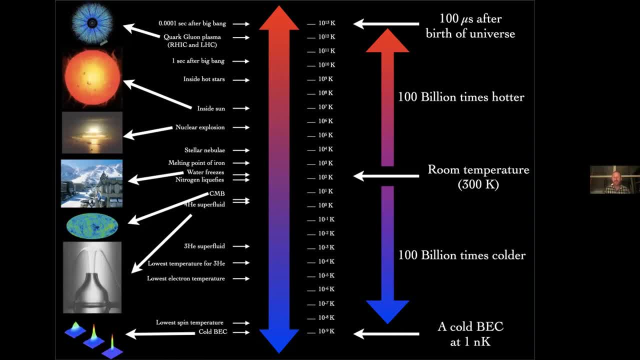 so maybe someone who has a better intuition of this phenomenon could comment more. Can you give the science fiction enthusiast version of this? The energy is a function of velocity. We know from high school physics that kinetic energy is half mv squared, half the mass times the velocity squared. 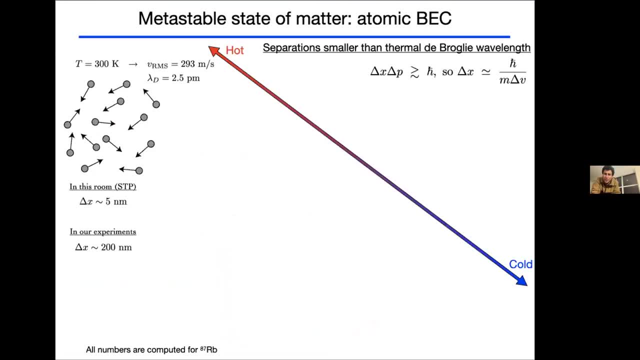 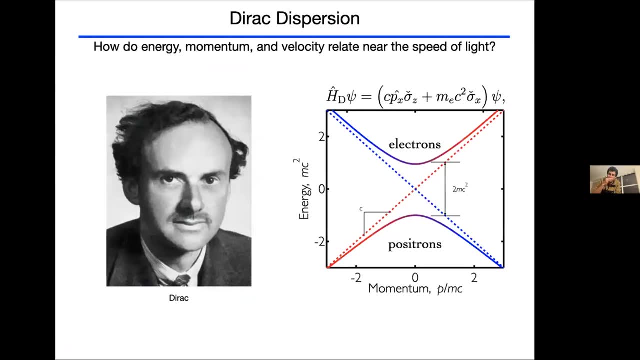 But actually Einstein corrected this equation. Einstein and Lorentz corrected this equation And they showed that actually that's the beginning. that's the low energy situation. At high energy, the energy diverges as the velocity comes to the speed of light. 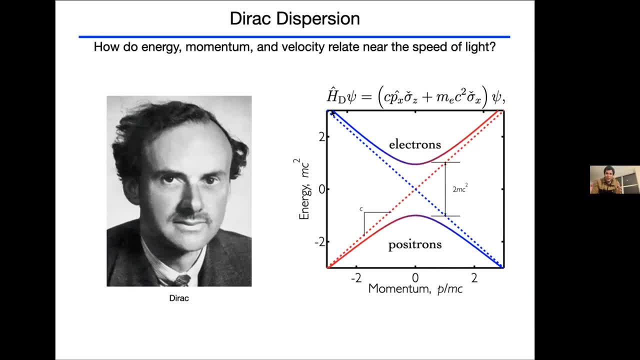 So if you're in a spaceship that has a constant pushing rocket behind you, like a ramjet that collects hydrogen and fuses it, your spaceship will constantly accelerate. However, from the rest frame of the planet that this spaceship is trying to escape, it will look like 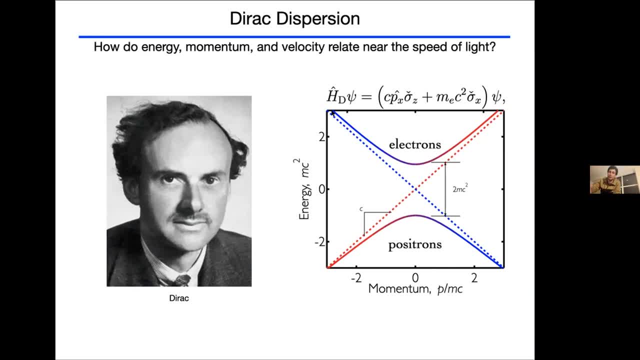 the velocity will asymptote to the speed of light but never reach there Because at any given time there's a finite amount of energy that goes into the spaceship and you need infinite energy to get to the speed of light. But you can get very close. 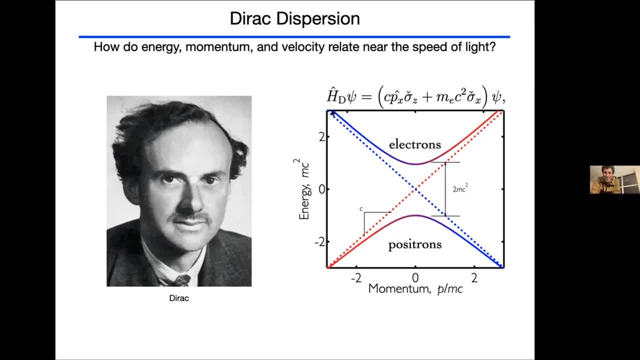 in principle. So that's my version of Fionn's explanation, if that's okay. Any other questions? Actually, Ian, I'm curious to ask. so over your years in cold atomic gases, what was the phenomenon that you witnessed that made you most excited? 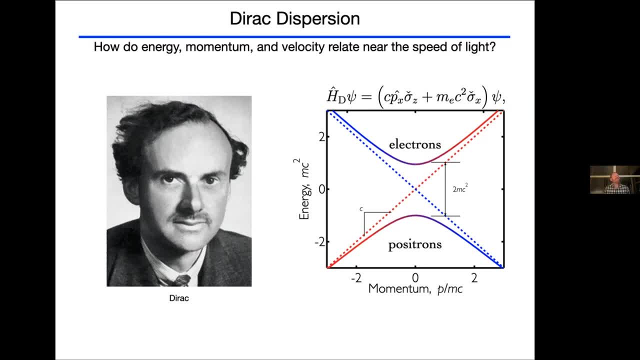 What was the thing that made me? You really get excited about your physics and I was really curious to know what's up there for you, Because one of them says something about my personality. So any time that I go into any of the labs and see 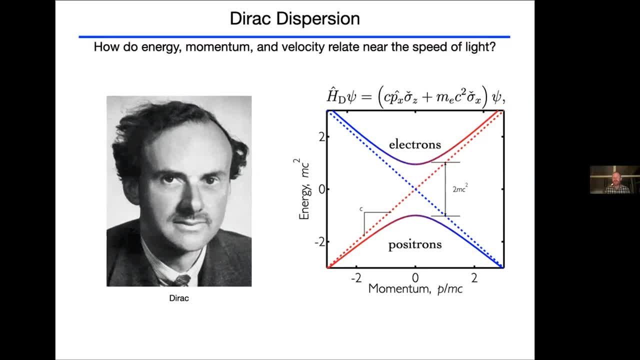 even laser-cooled atoms, but in particular pictures of VECs appearing on the screen. it does not cease to blow me away. Think about, we just took a photograph of something of thousands to millions of atoms whose temperature is a couple of nanofilms. 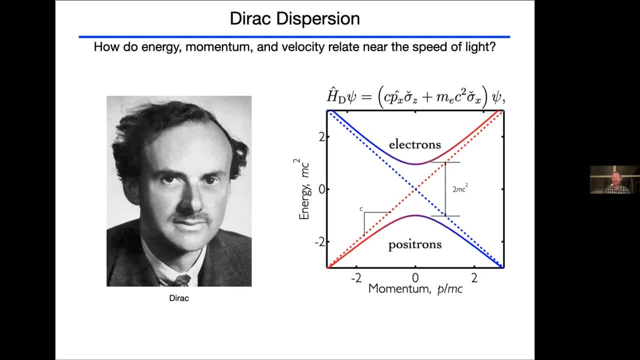 and that just blows my mind every time I see it. So I guess I haven't reached that level yet. The thing that I think was most exciting to me was when we were doing an experiment realizing spin-orbit coupling, So this was the second project. 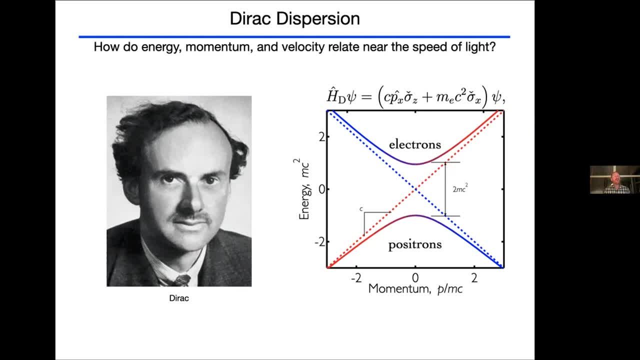 that Yuzhu Lin was working on when she was a postdoc with me, And what it had. It's a funny thing. I had written a grant proposal and realized, sort of independently of what some other colleagues had been working on, that we could do a particular 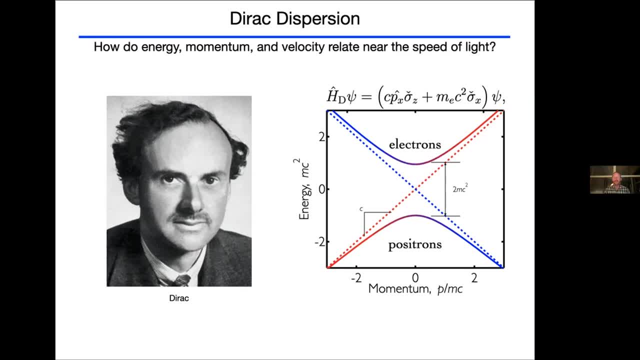 grant proposal. Then I asked Yuzhu to work on it in the lab. Then it didn't work. Things didn't make any sense And it turned out we had a perturbing, unwanted gradient magnetic field present. So then I remember, 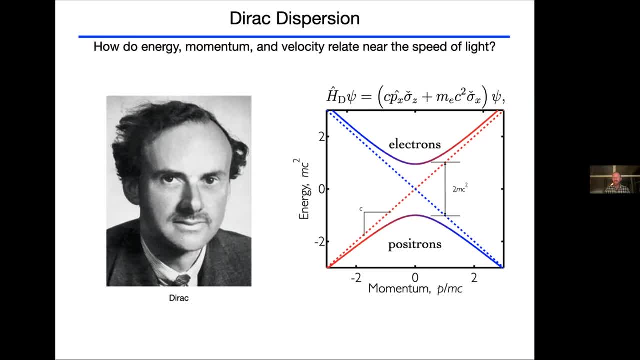 that when she compensated that, all of a sudden we had this beautiful data. That system has a mean-field quantum phase transition associated with it that no one had ever predicted. So she showed this data of the VEC and it was like half being spin-up.